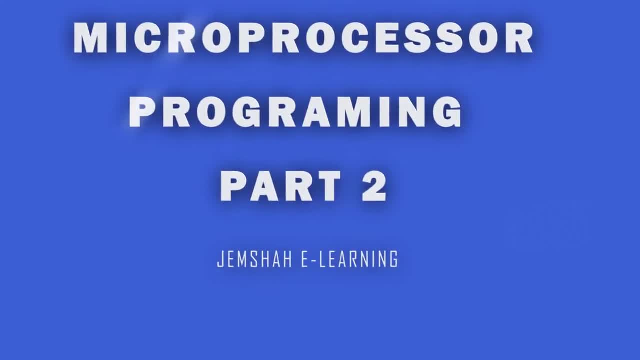 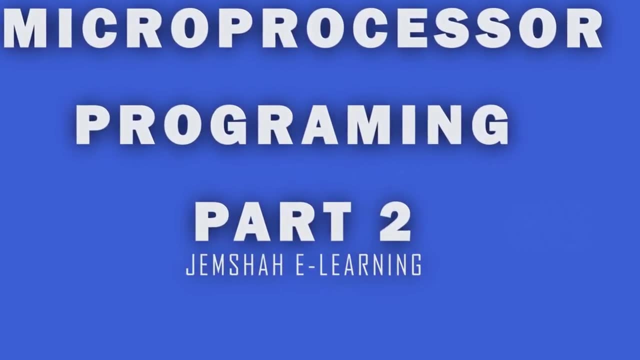 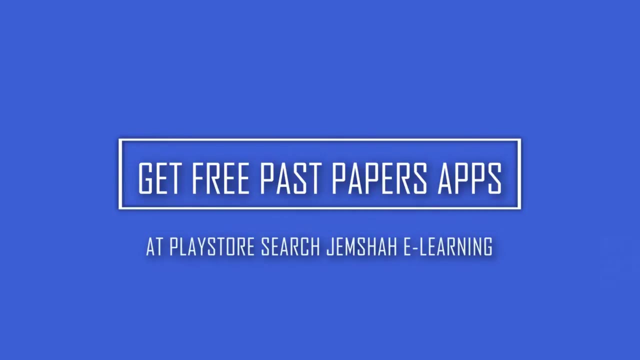 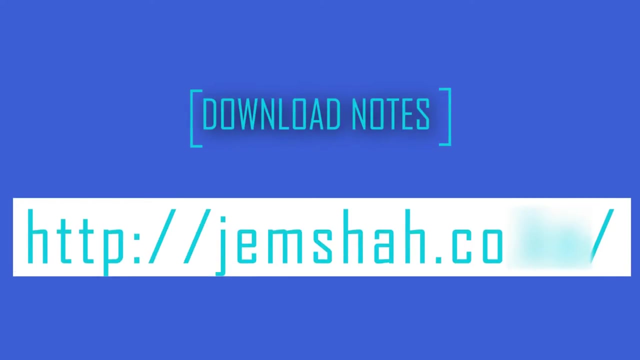 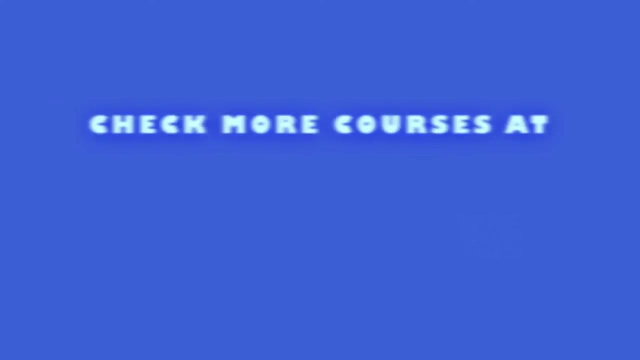 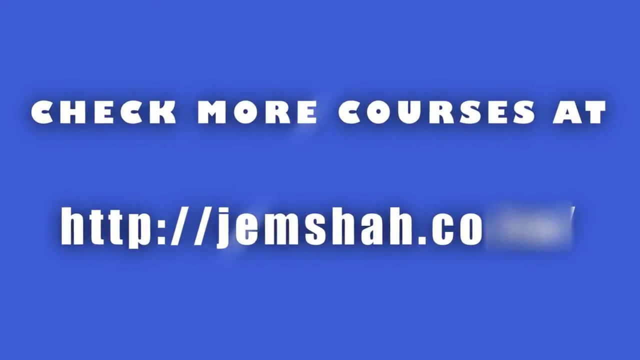 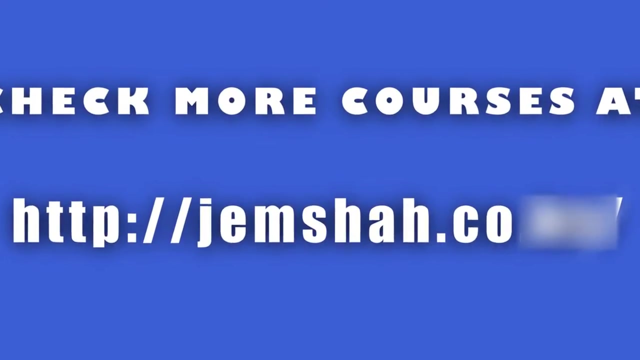 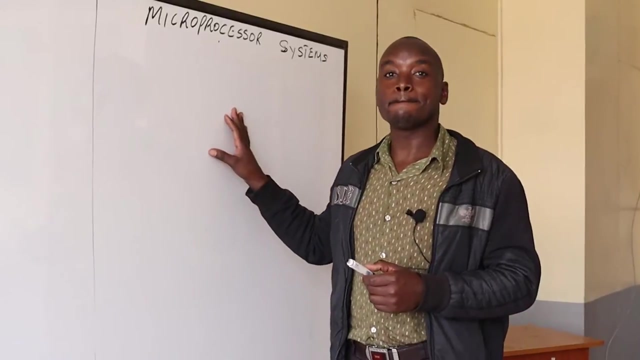 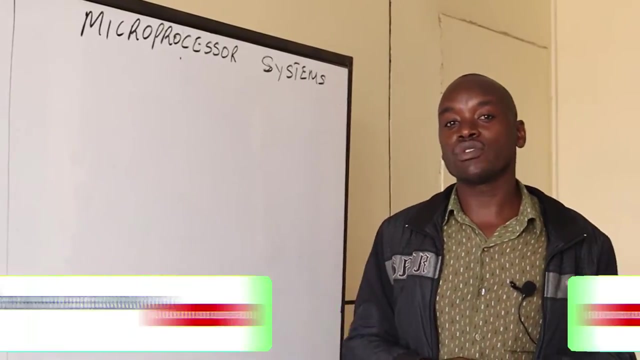 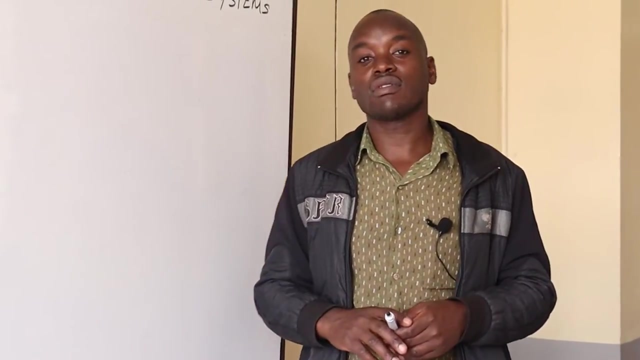 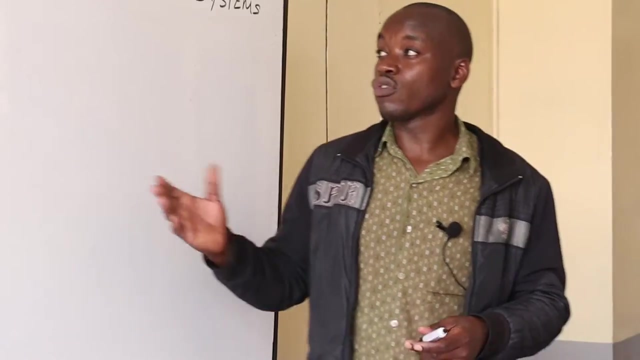 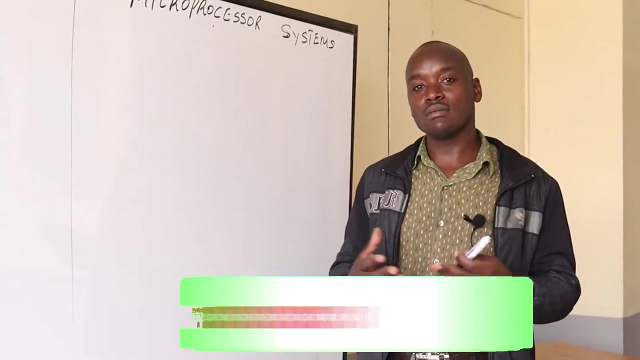 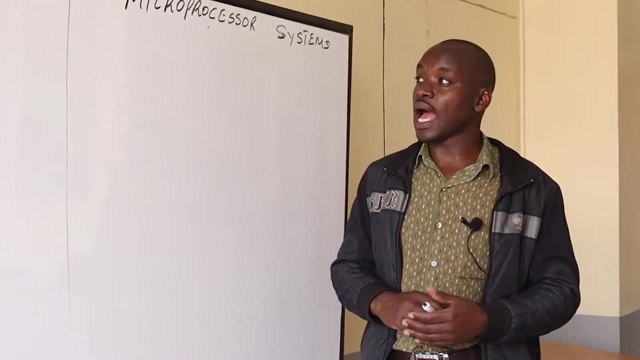 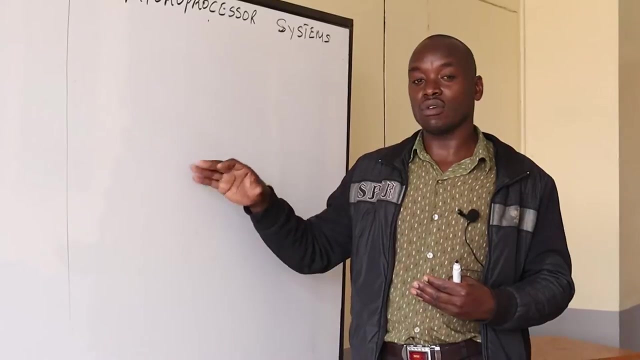 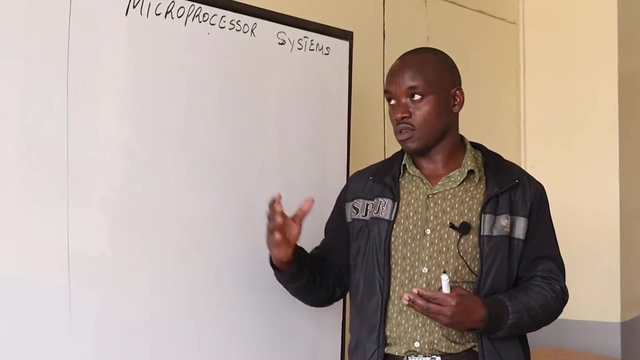 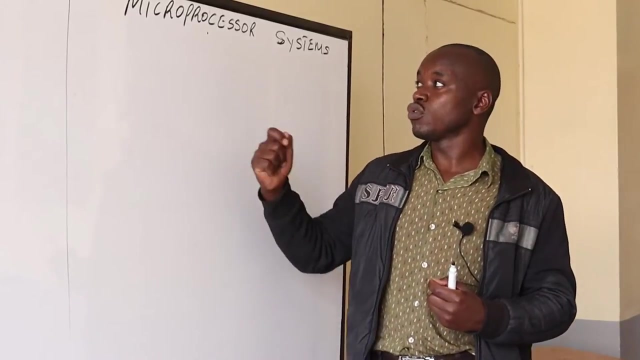 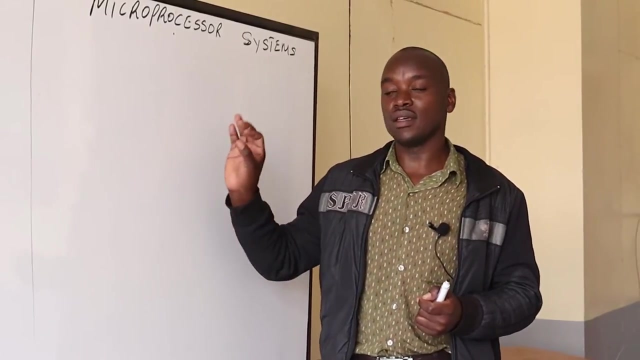 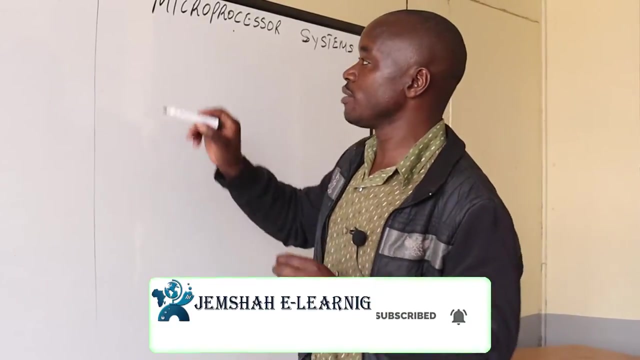 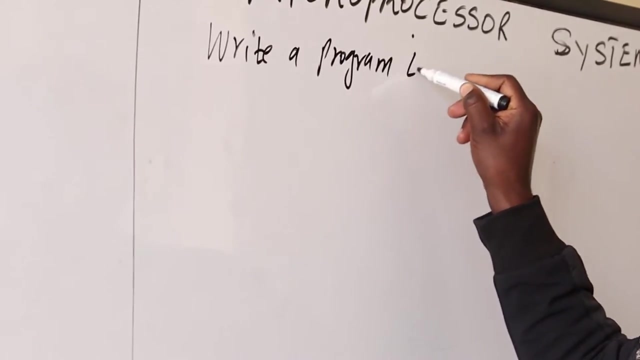 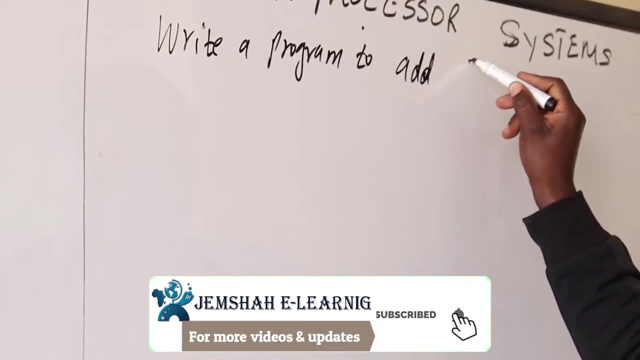 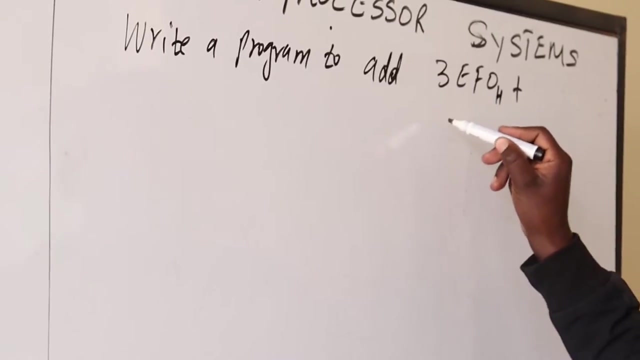 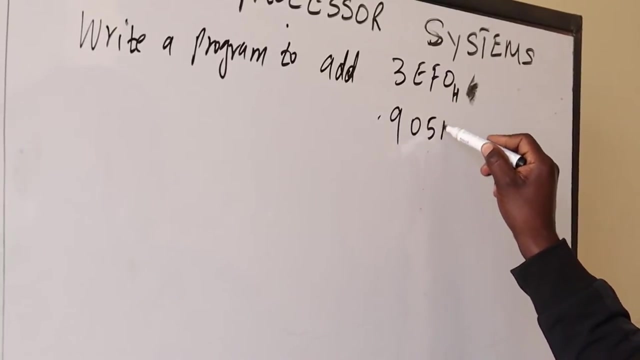 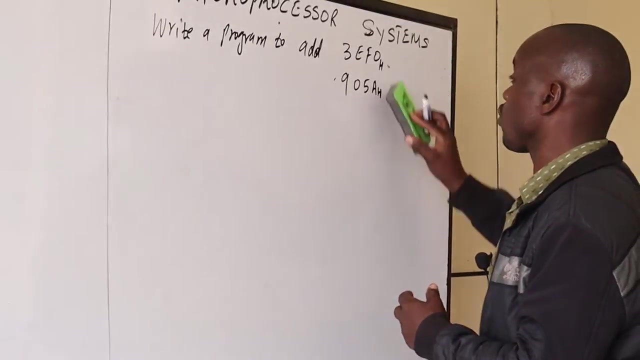 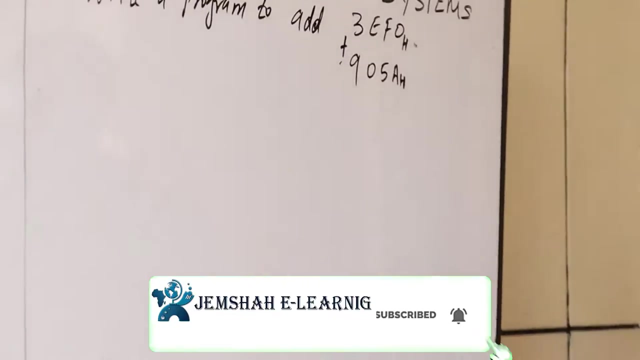 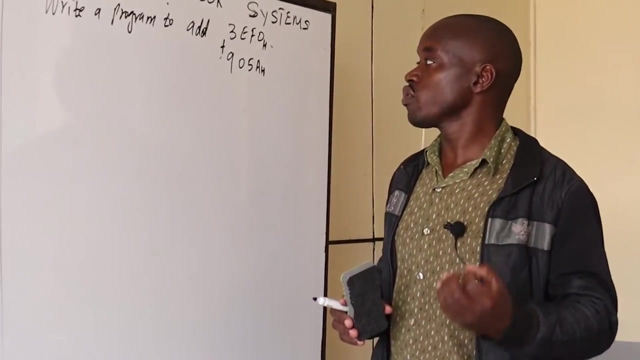 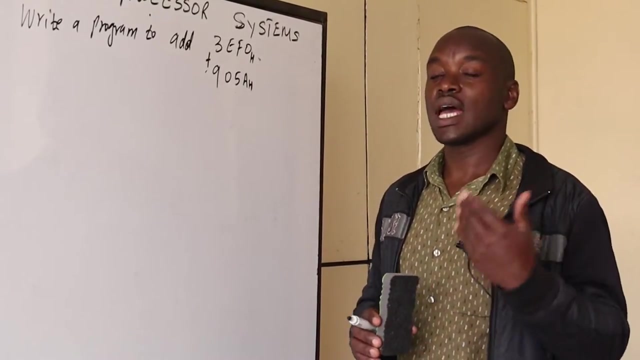 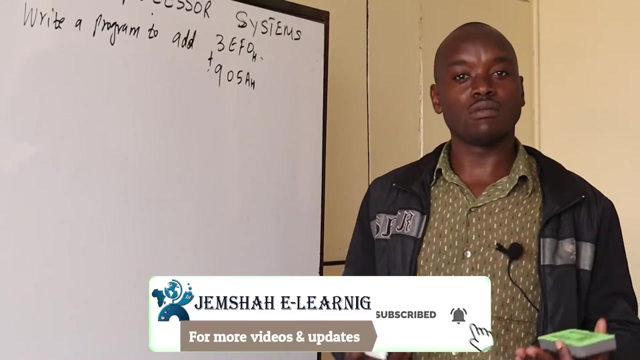 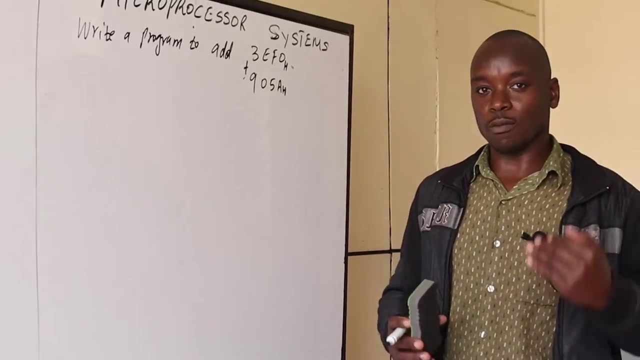 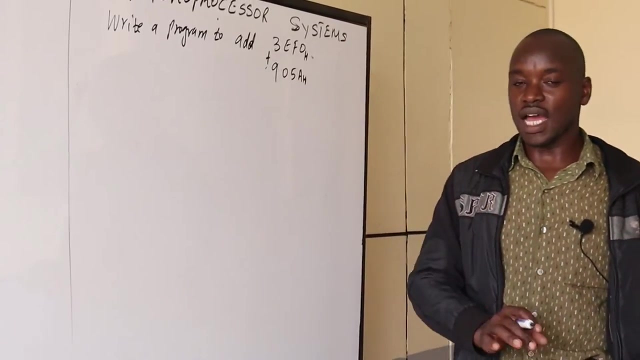 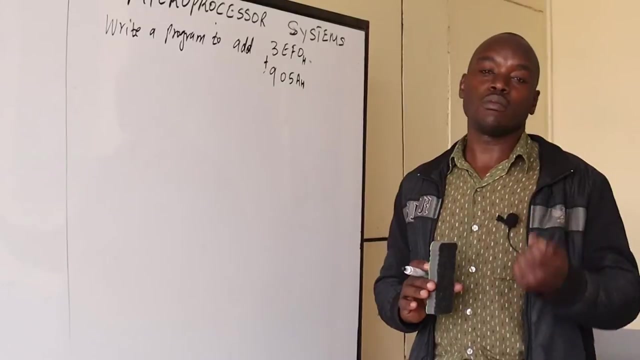 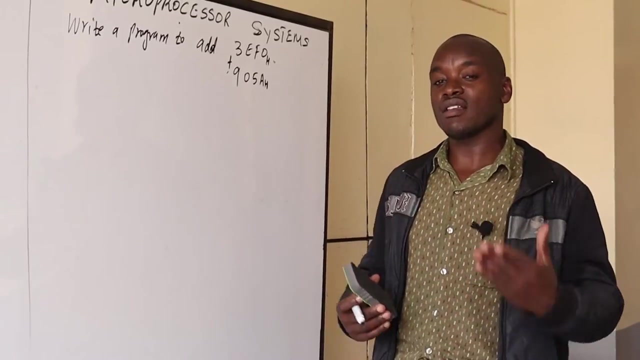 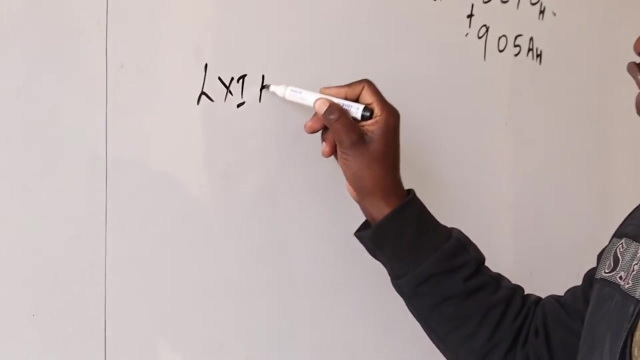 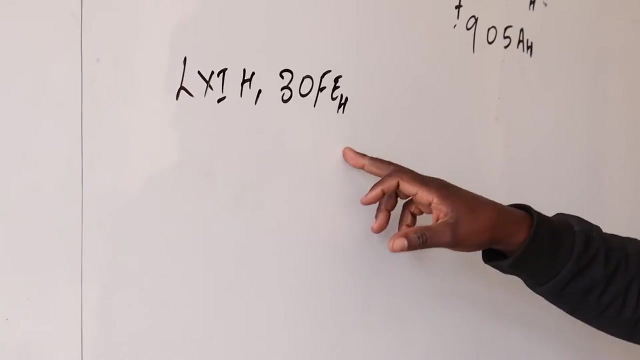 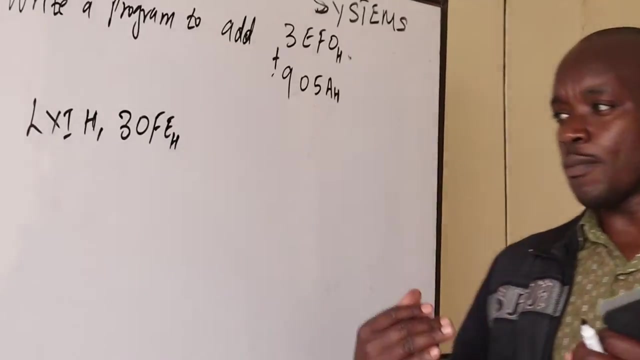 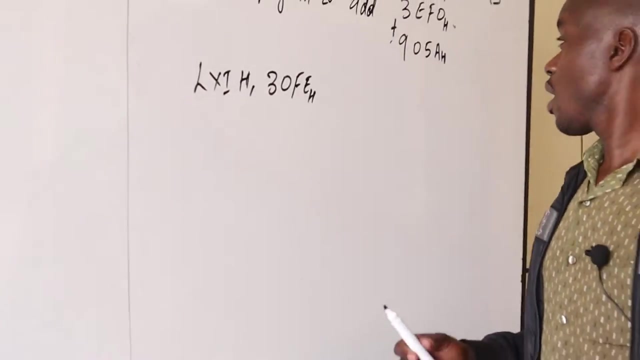 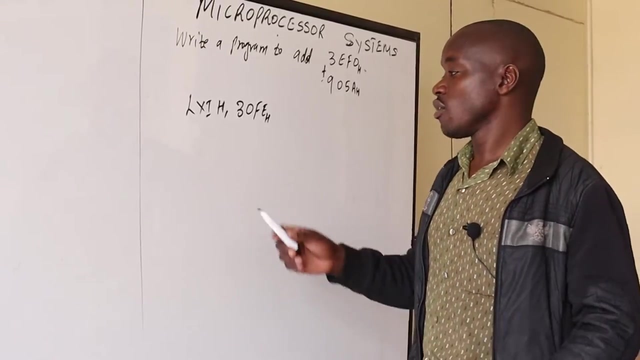 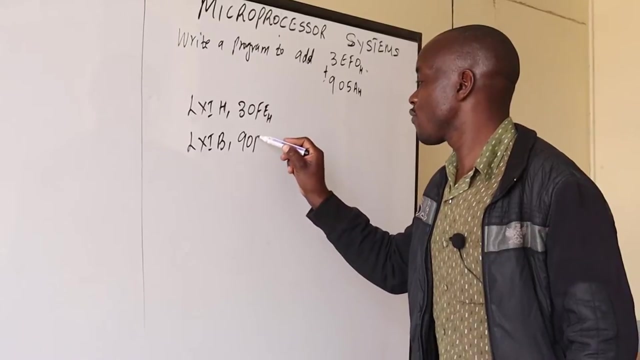 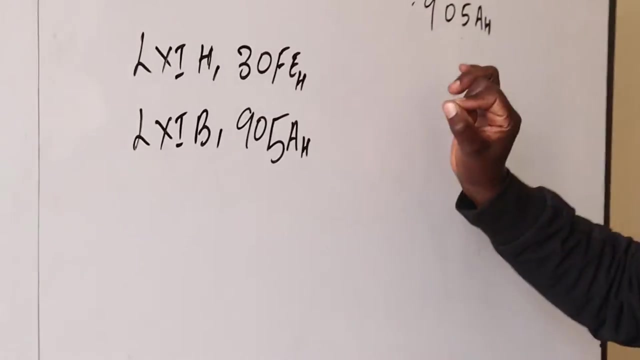 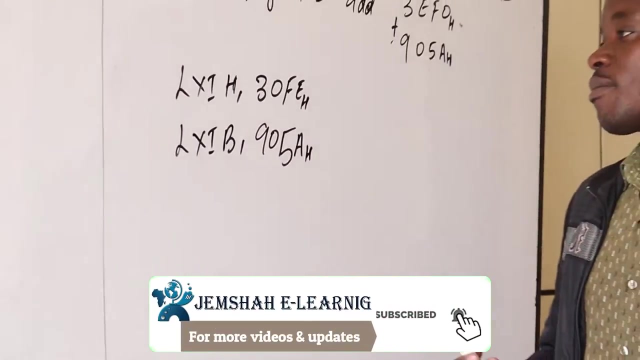 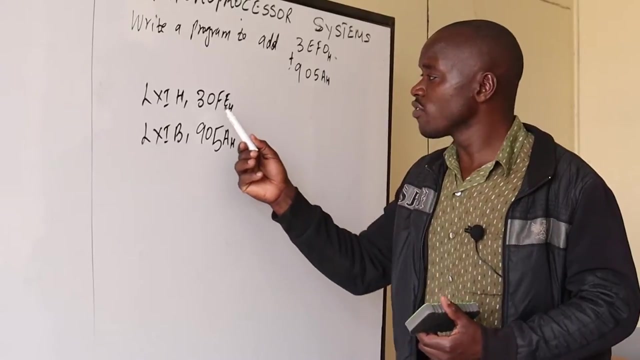 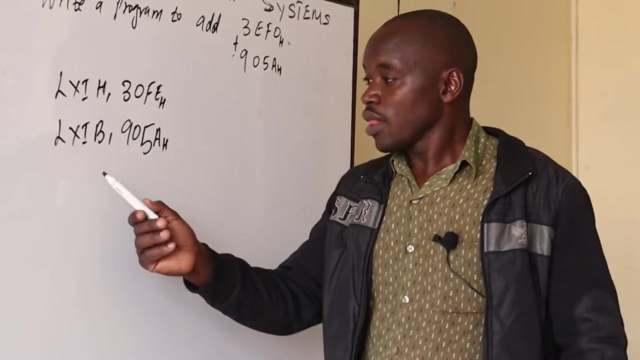 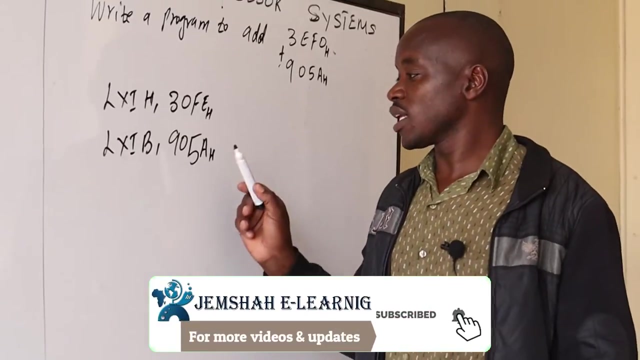 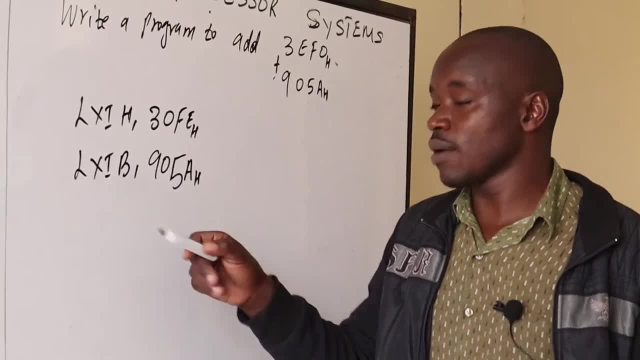 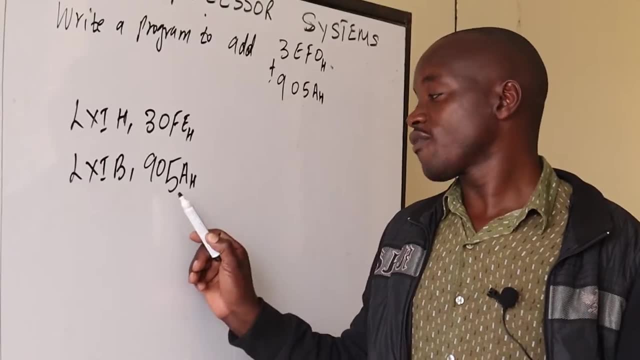 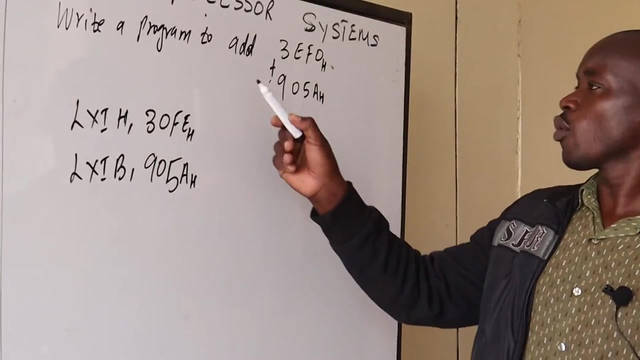 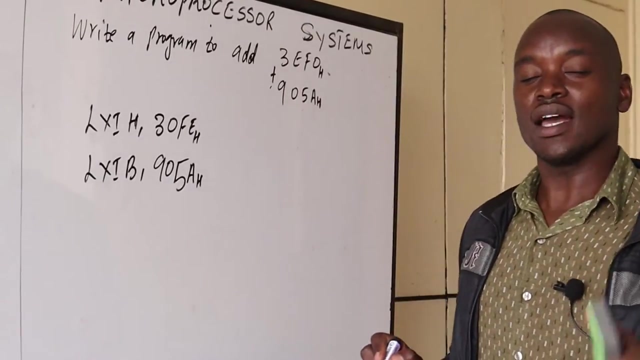 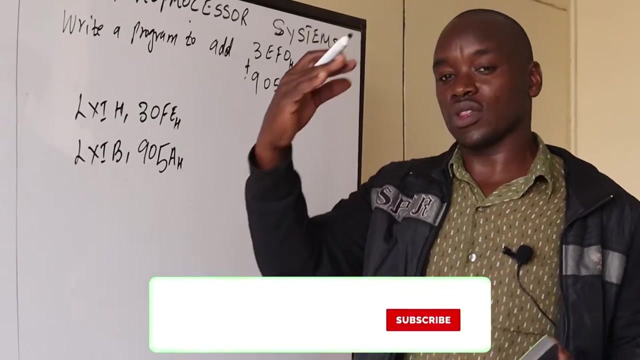 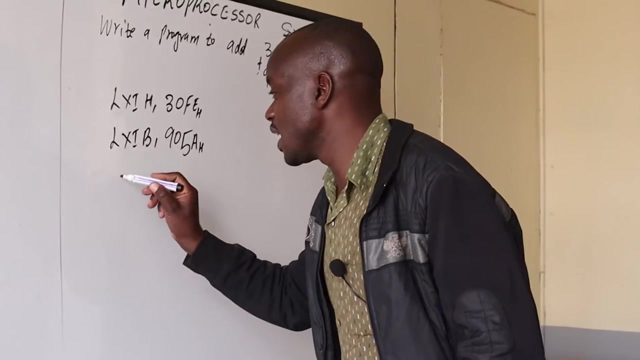 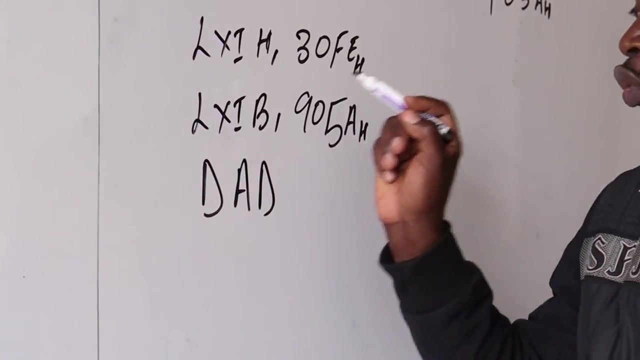 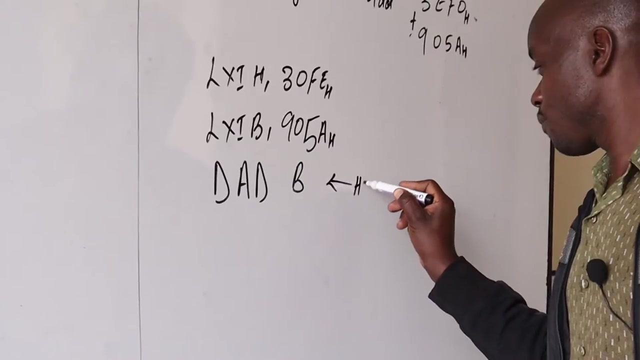 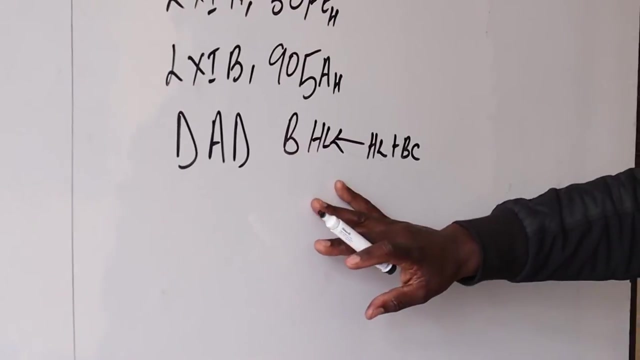 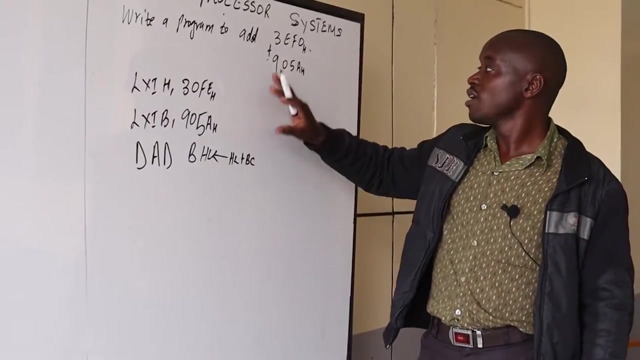 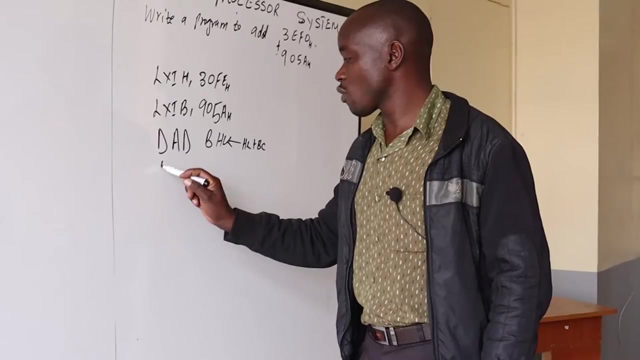 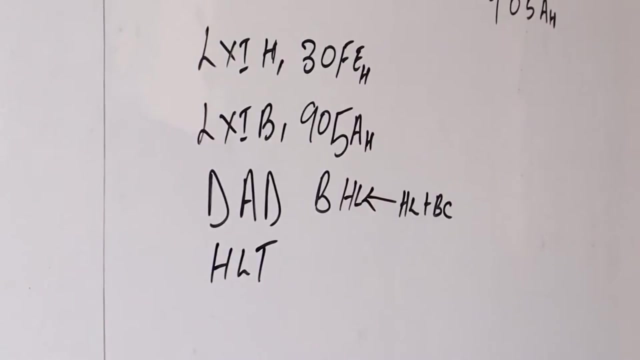 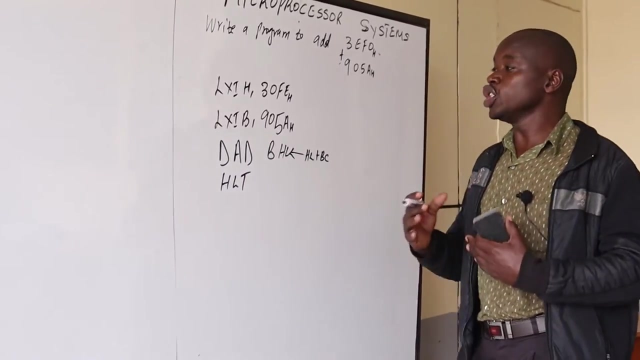 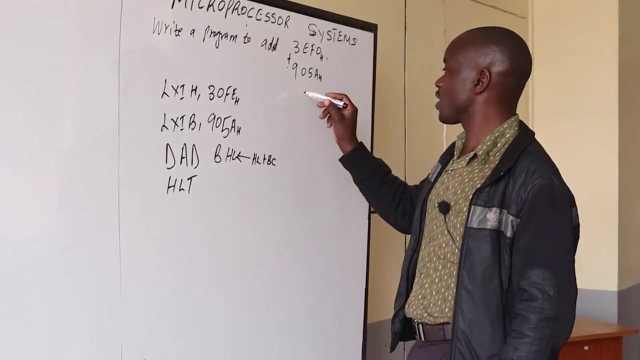 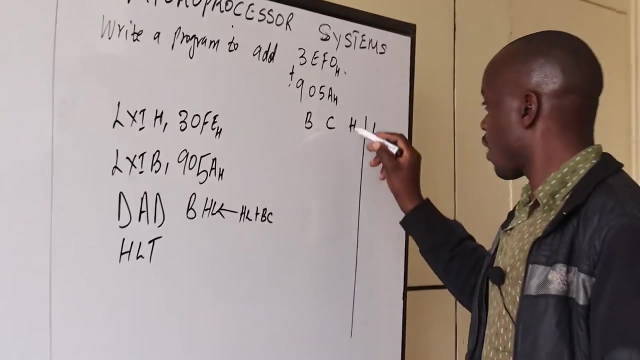 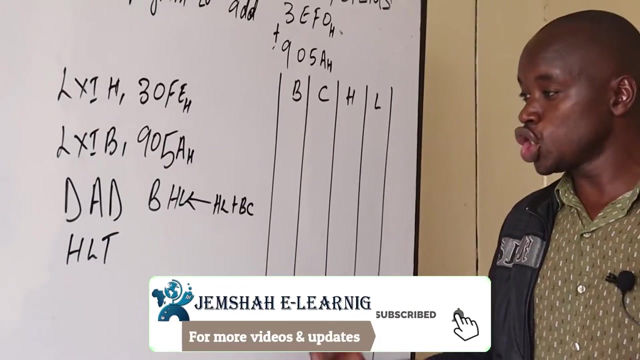 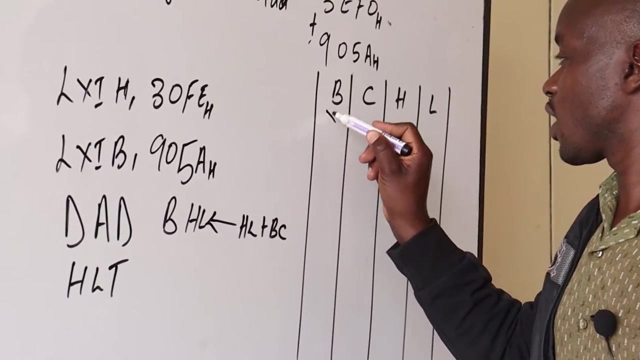 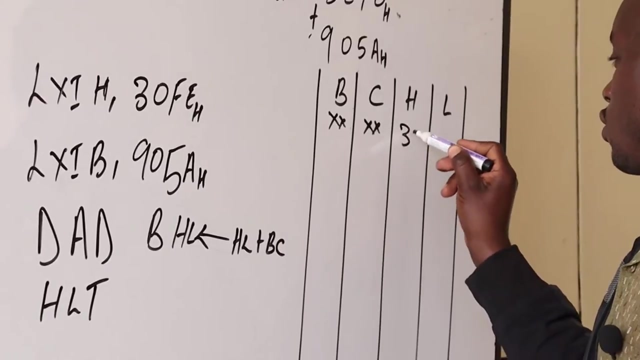 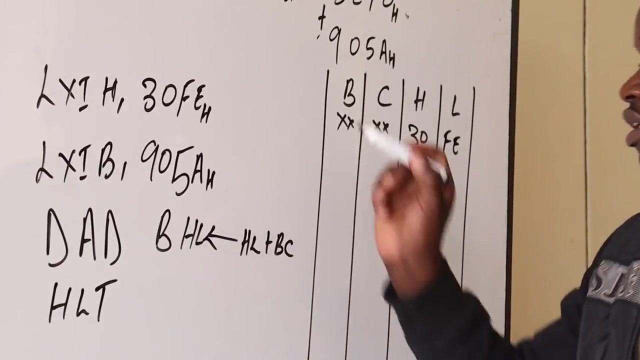 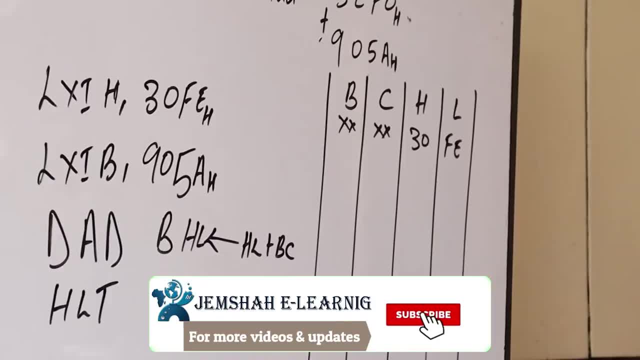 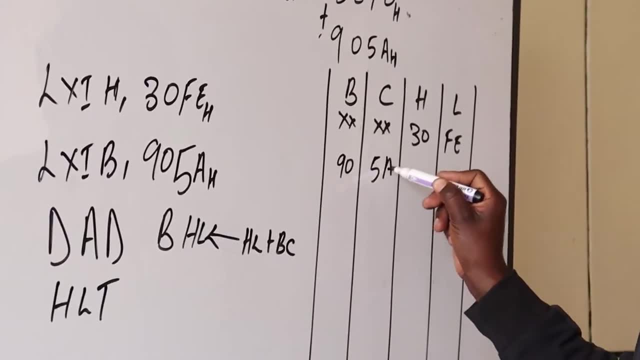 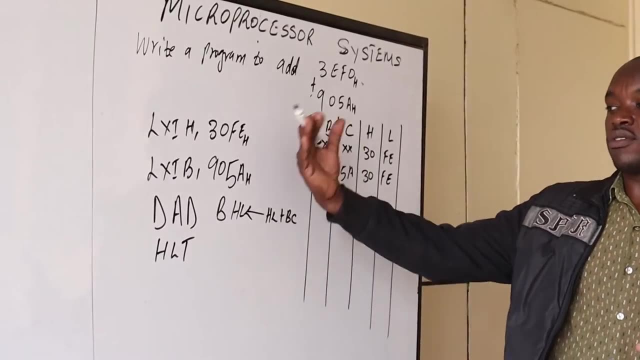 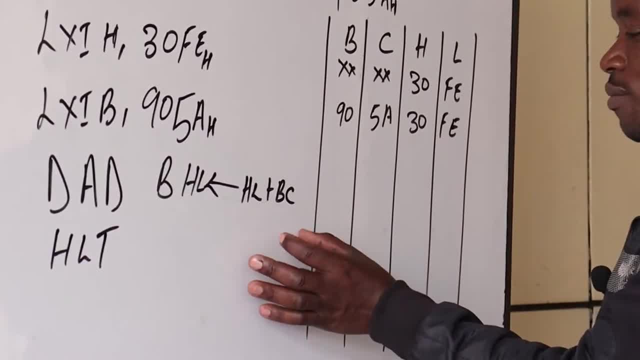 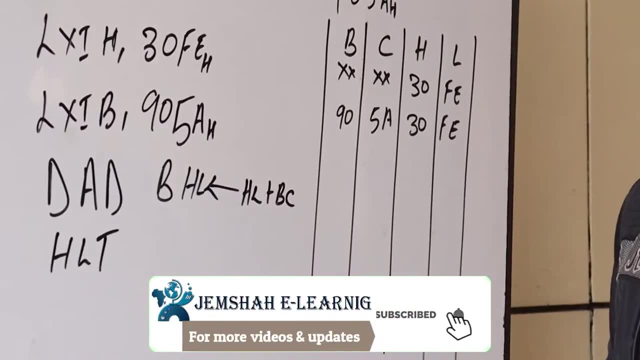 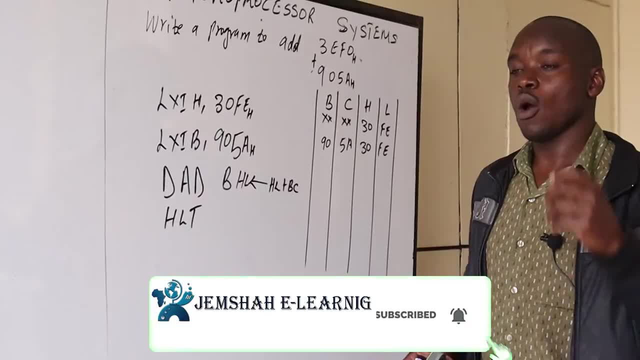 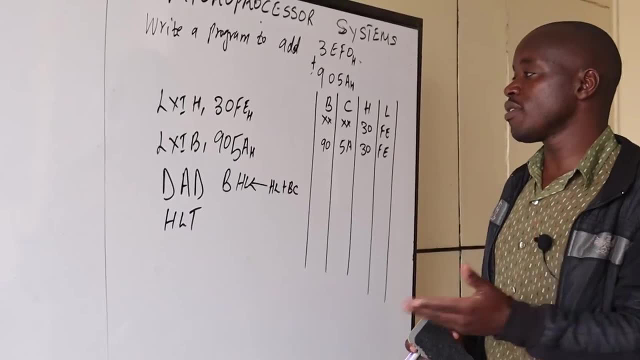 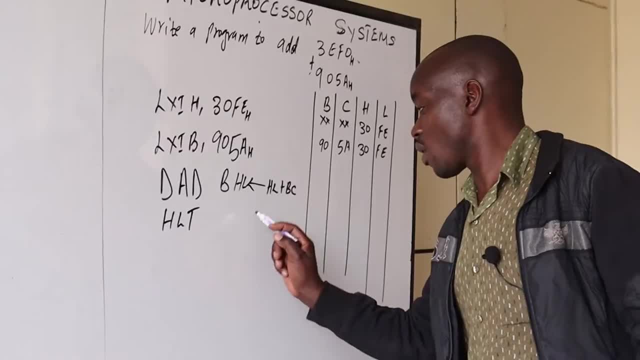 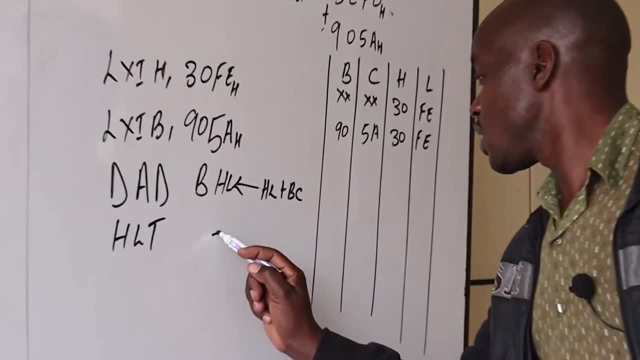 Thank you for watching. Thank you for watching. So what will happen now is- I want to do it practically before I write there. Dad B means whatever is in HL plus what's in BC. the answer goes back to HL, So it is 905A plus 30FE. 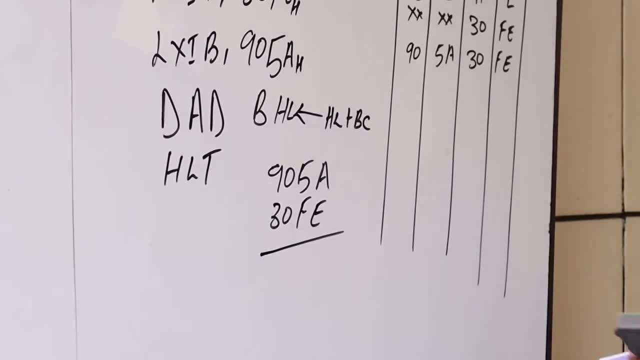 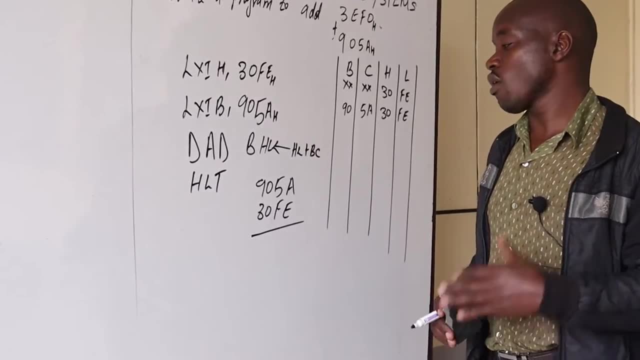 Now I want to add this. There are two ways, but I want to use the symbol as well. We have agreed that we are using base 16.. So there should be a carry when the result of an operation exceeds or equal to the base. 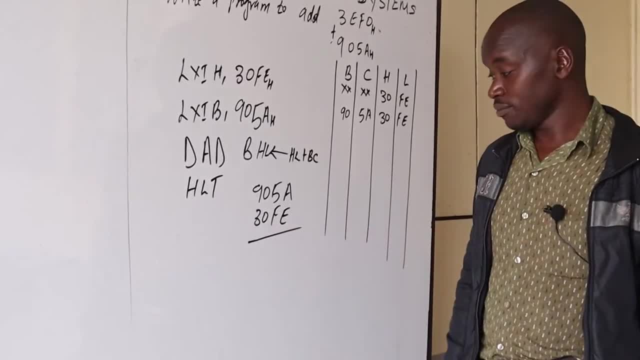 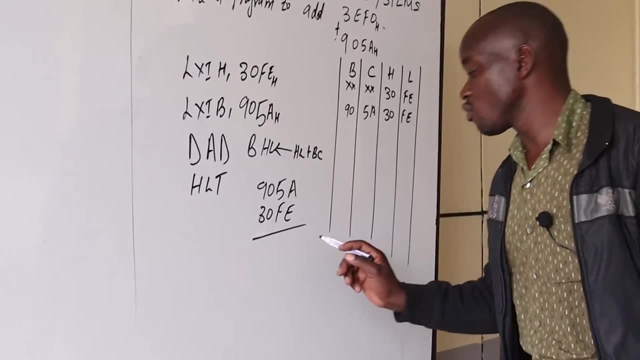 or the radix 16.. So A is 10, E is 14.. So 14 plus 10 should be 24, minus 16, the answer remains what? 8. Carry 1. The one we are carrying in this rectangle we agreed is equal to the base. 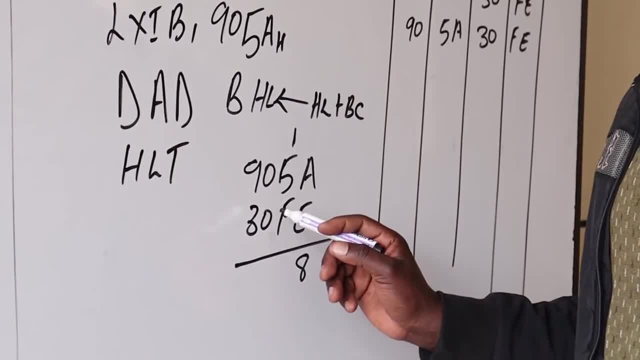 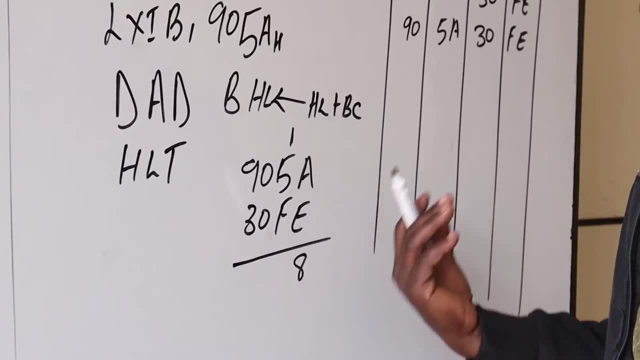 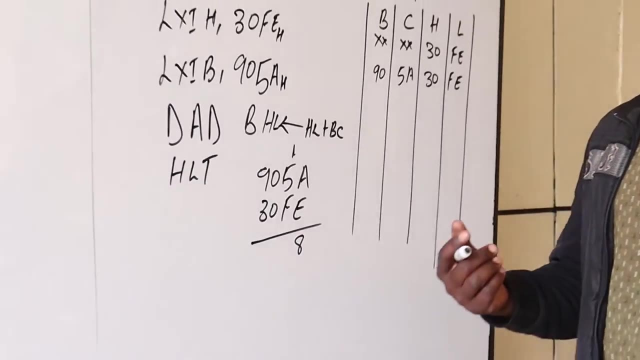 1 plus 5 is 6, 6 plus F, which is 15.. So this is 21 minus. sorry, that is 20, minus. let me see: 1 plus 5 is 6.. 6 plus 15 is 21,. 21 minus 16, the answer remains 5.. 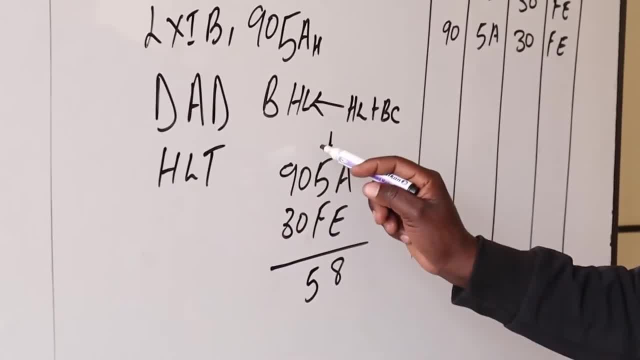 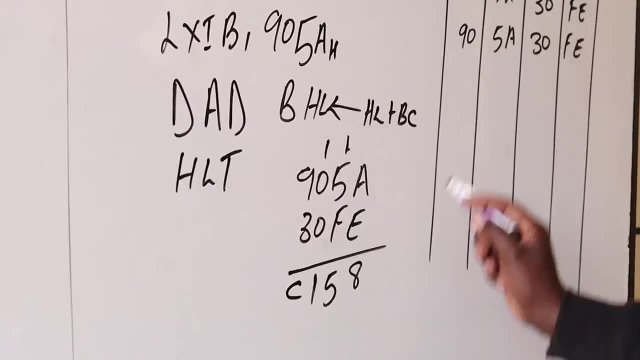 So we have 5 here. Then here there is a carry. so because 00 we have 1,, 9 plus 3, it is 12.. 12 in xylism is what C, So the answer becomes CE C1. rather sorry. 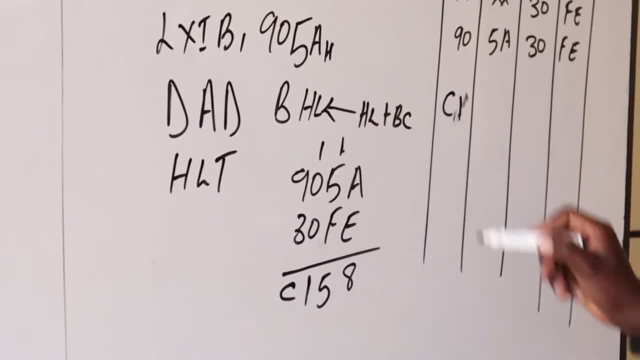 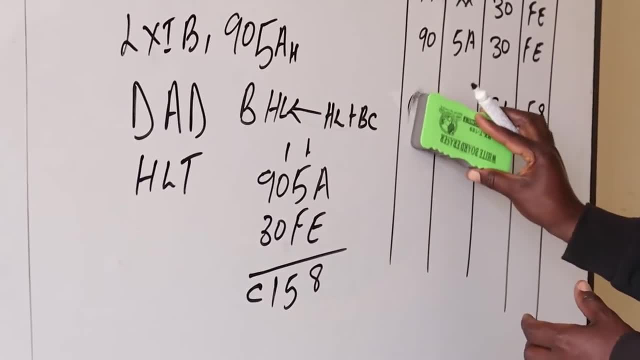 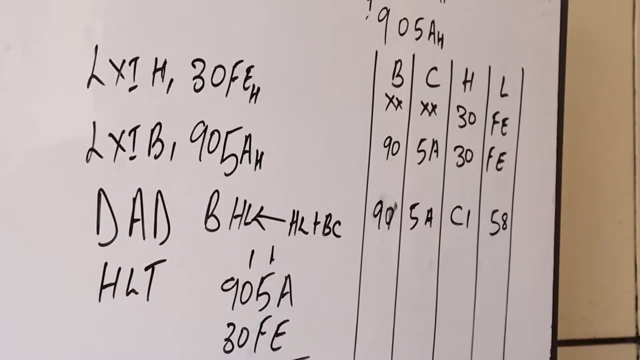 The answer should be C1, C1 in H, because the answer goes back to HL: C1,, 5, 8, but here we remain with 9, 0,, 5, A. Now, then next instruction is stop or halt. 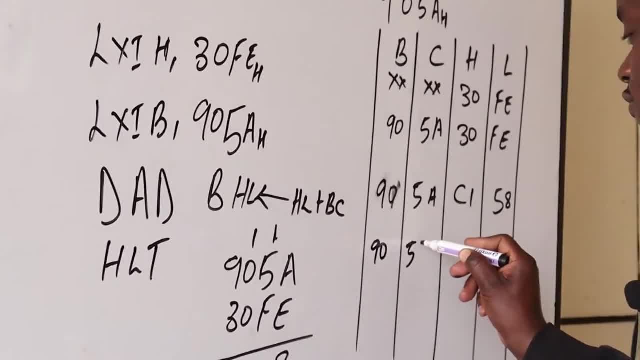 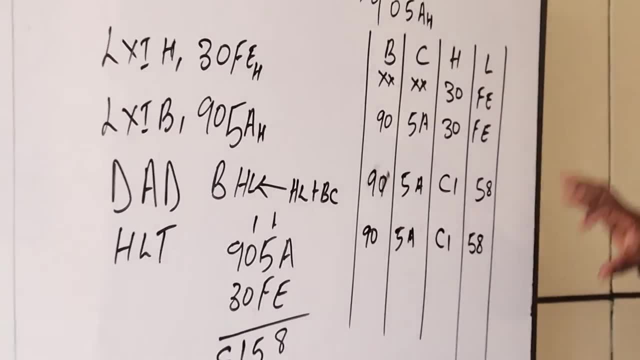 So when we stop here, we have 9,, 0,, 5,, A, C1,, 5,, 8, and this is our trace table. So I've used a trace table so that at least a candidate or someone who wants to understand 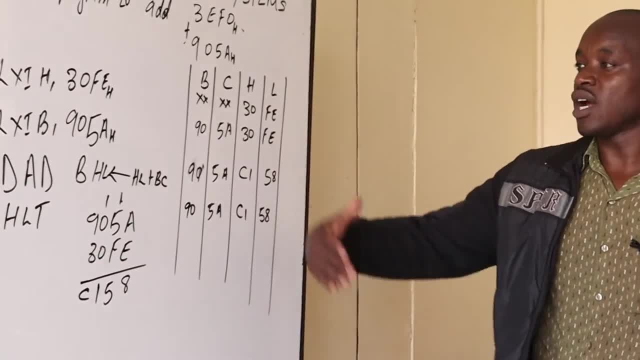 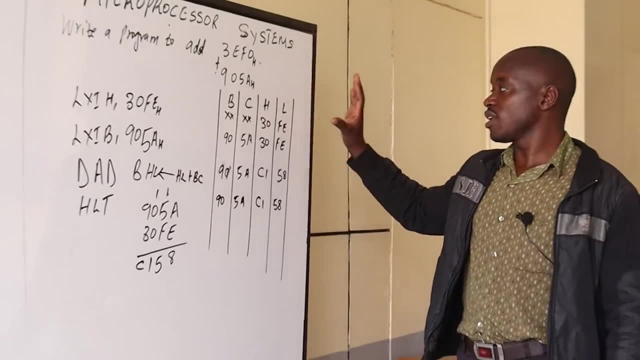 this microprocessor in 10, 8,, 8,, 5, will understand at each instruction execution what was happening. So at the end of the program, this was in register BC and this was in register HL And we agree this equation. we want to do it in two ways. 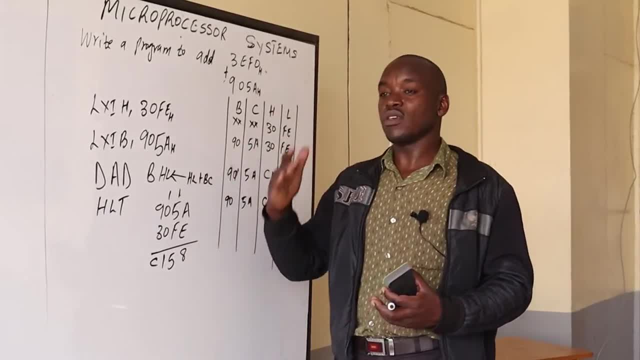 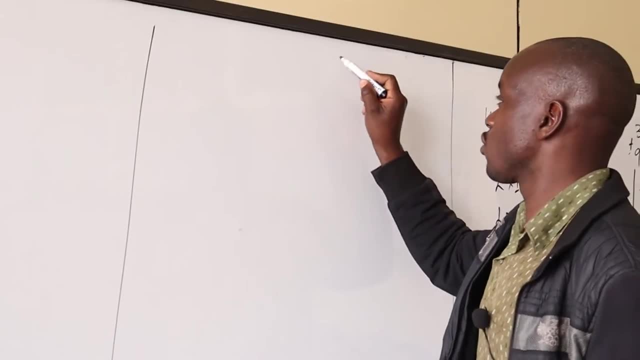 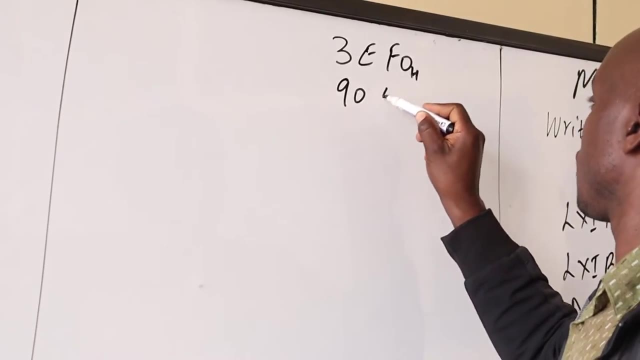 The first way was using register pairs. The second way is using registers. Now let us move there, so that now we do it. what Using registers? Remember the equation is addition of 3EF0H, then 9,, 0,, 5.. 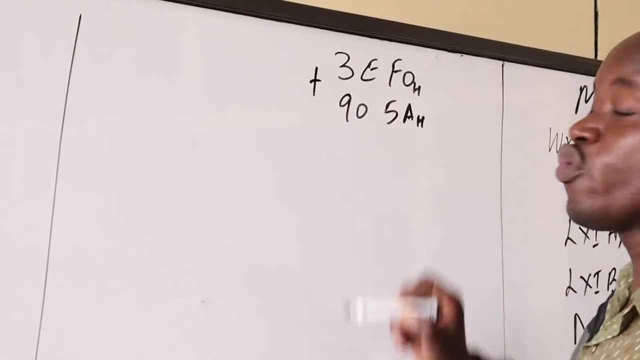 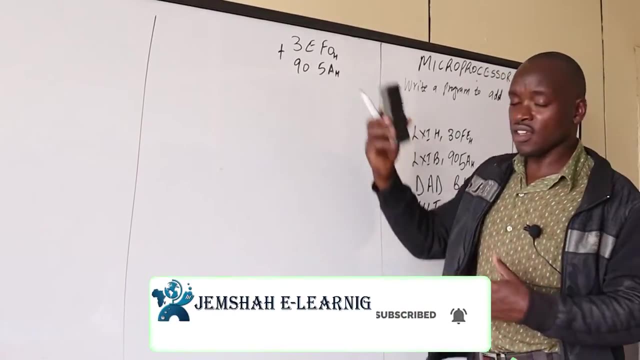 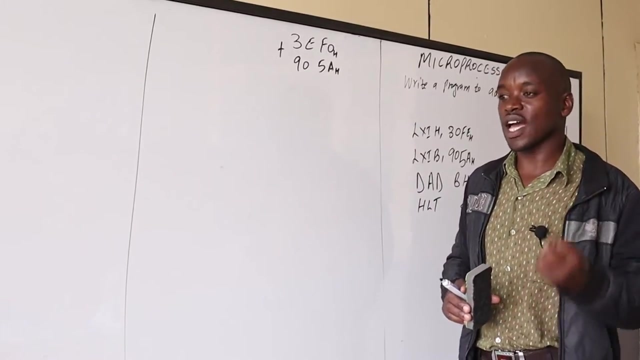 5, A H. We want to add this using registers, because we don't know what the examiner would examine us. he might ask us using registers, pairs or just using registers. Now, what we are supposed to understand and remember is in registers. a register can only. 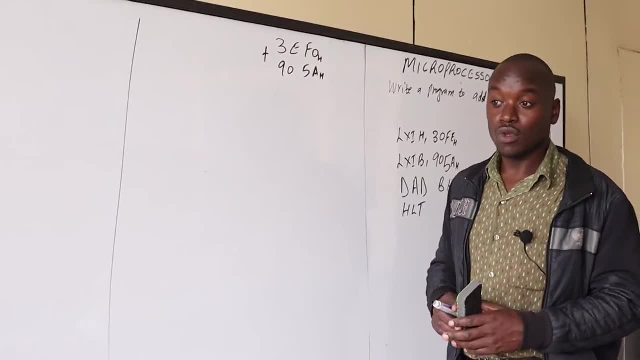 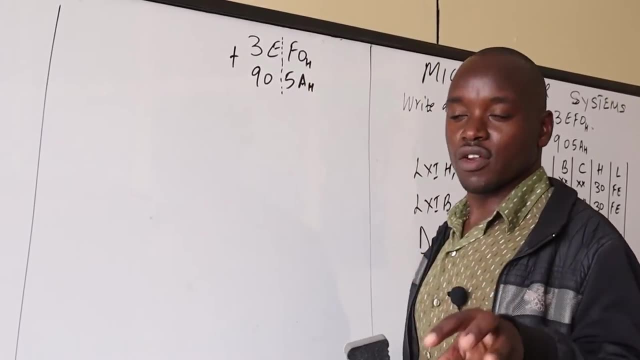 take how many bits In? 8, 8,, 5,, 8 bits only. So I know, from F, from 0 to F, these are 8 bits, so I'm supposed to add this one first. put the result somewhere. 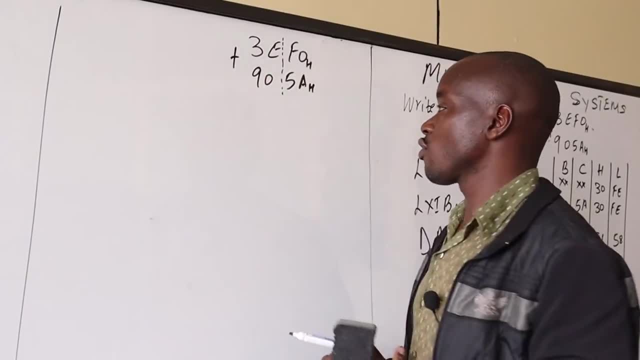 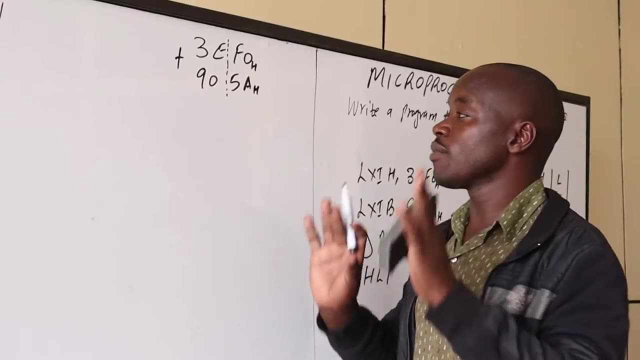 Before, Before I add again this, the other A 8 bits. So in addition of 8 bits in register pairs, HL is our accumulator In 8 bits accumulator is register A. So we start the first thing we start will be. 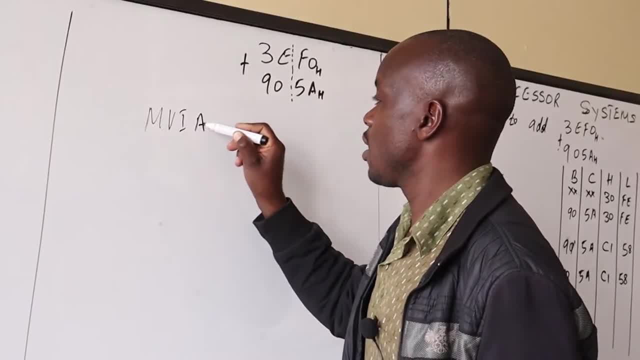 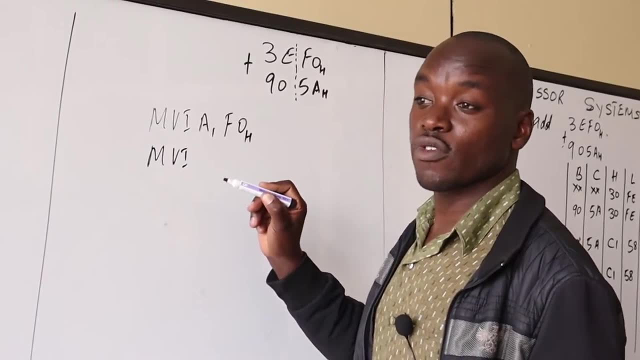 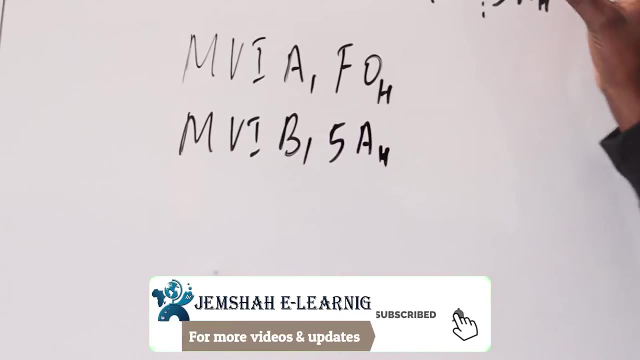 move immediate MVI A, F, 0, H, Then MVI, the next general purpose registers which we agreed, which was register B, what 5, A, H. So These two bytes of data, which are 8 bits, are in different registers and we are supposed. 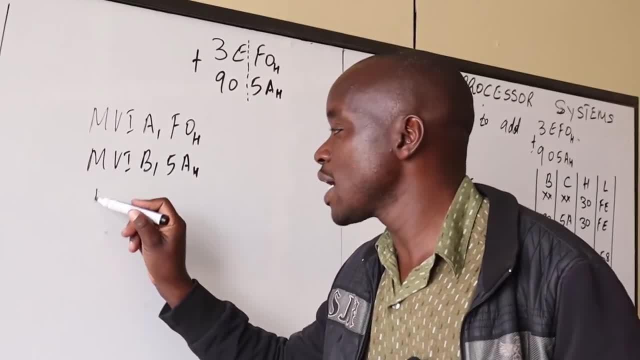 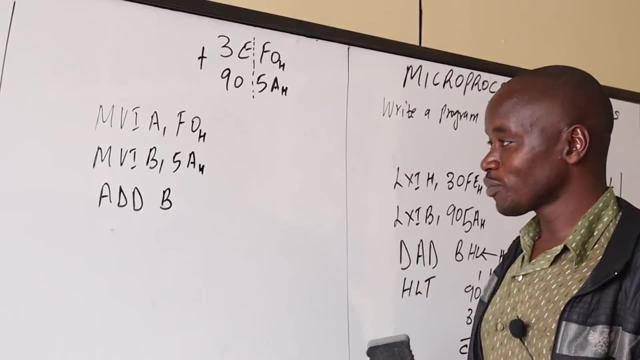 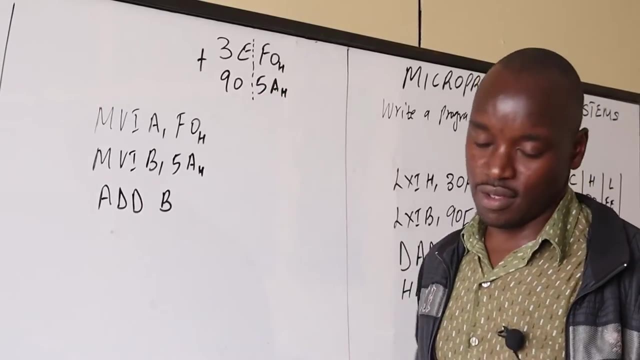 to sum them or add them. So that will be ADD B, which means check what's in A add with what's in register B. the answer goes back to A. Now, since I want R3, E and the 9, 0, and the first submission. 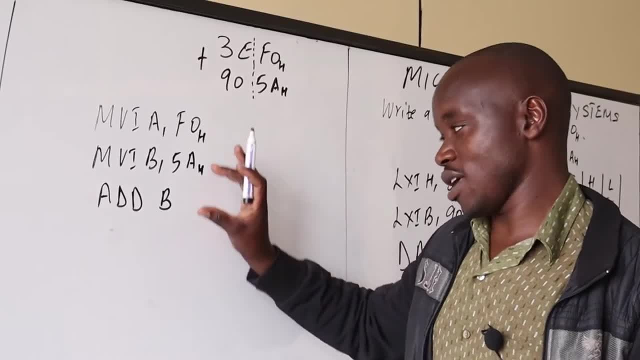 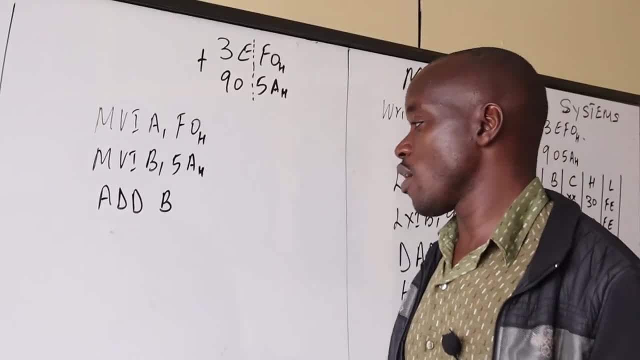 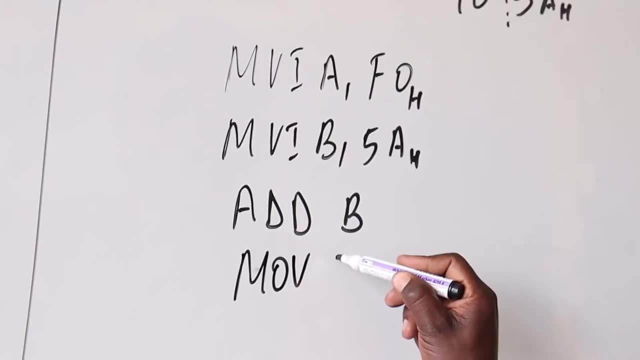 you remain with the original and I copy somewhere. So what I will do, I will come here and then I say MOV, copy, MOV to another register. I can even decide to use C Copy to the register C what is in A? So why am I copying? 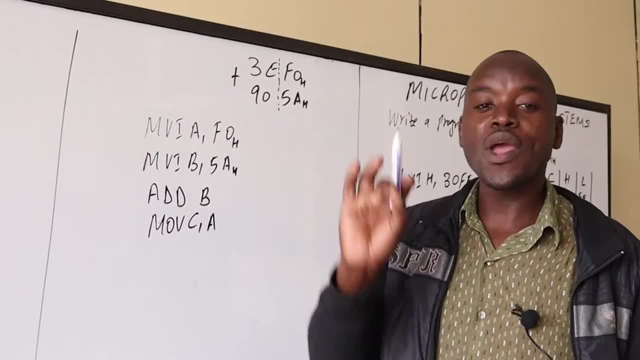 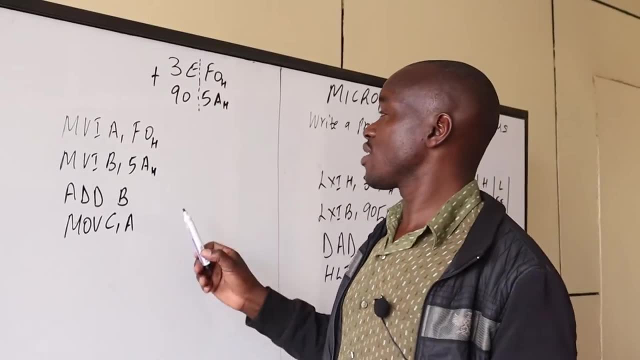 Because the candidate should understand why we are copying. We are copying reason being: the result of F0 plus 5A is in the accumulator And the same accumulator is supposed to use to add 3E and 9.0.. So the only 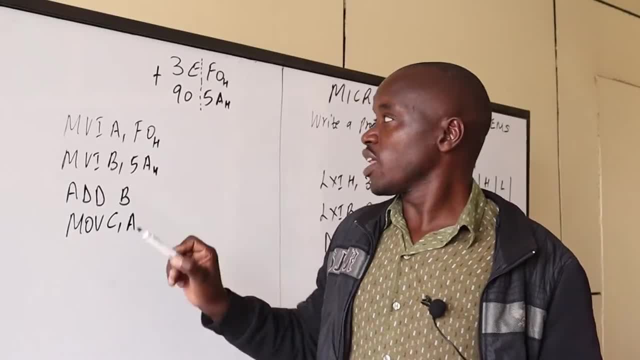 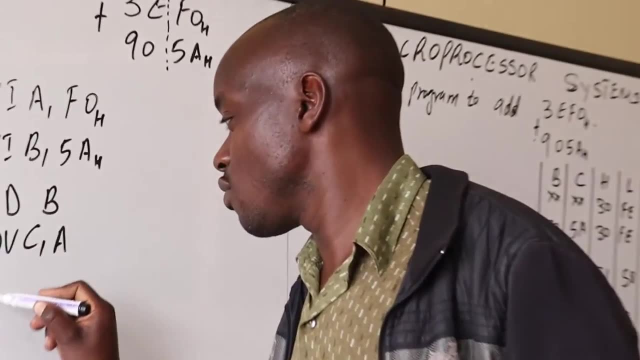 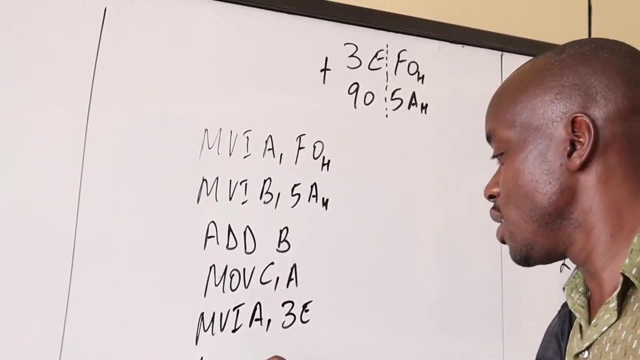 option is for us to save this result somewhere so that I now use A to add 3E and 9.0.. So we come here and then we say: MOV, immediate MOV, immediate register A, 3E. then MOV, immediate register B, E. now I can use D. 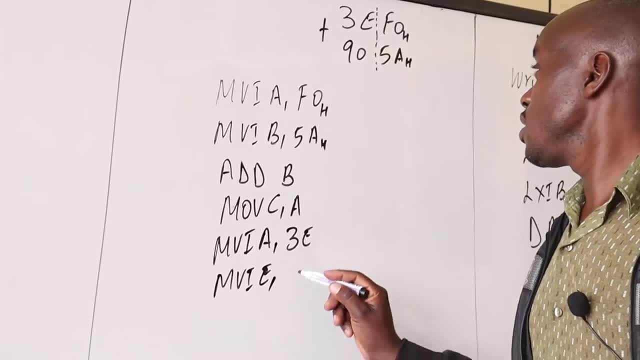 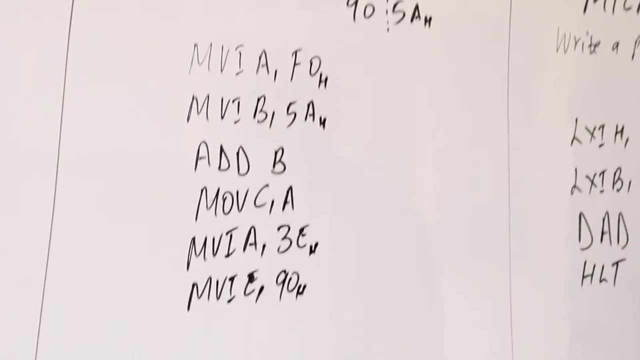 or any. I can even use again B E 9.0.. So the data is in H, It is in hexadecimal. So now, before I add this, I have to check. when I was adding this here, F0 and 5A was. 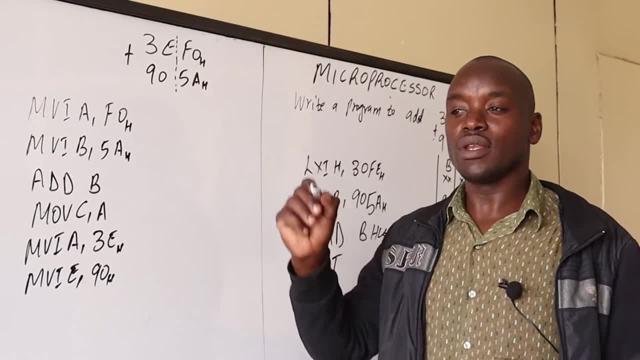 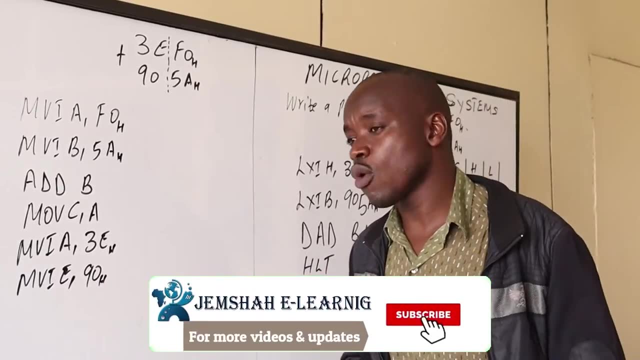 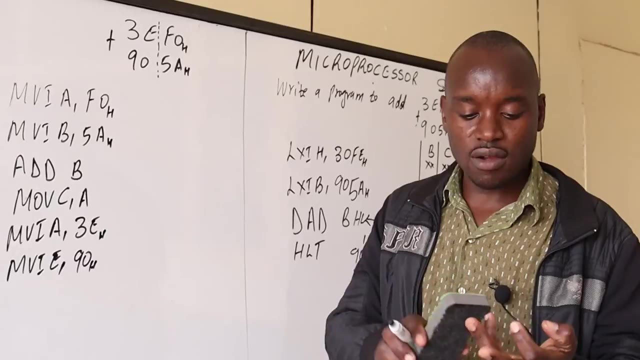 there a carry? If there is a carry, then I should remember to add, with an instruction which remembers, a carry in the carry flag. Remember, when we were doing the flag register, we talked about several flags in the flag register. We talked about the carry flag. 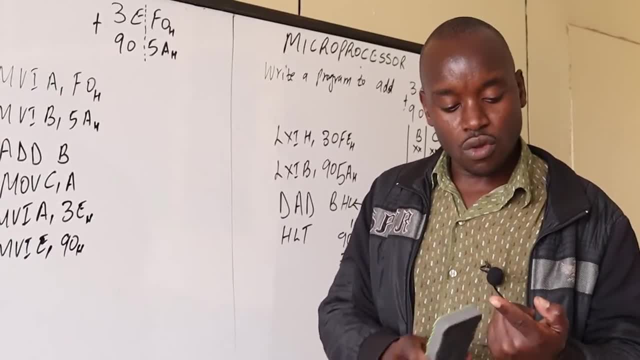 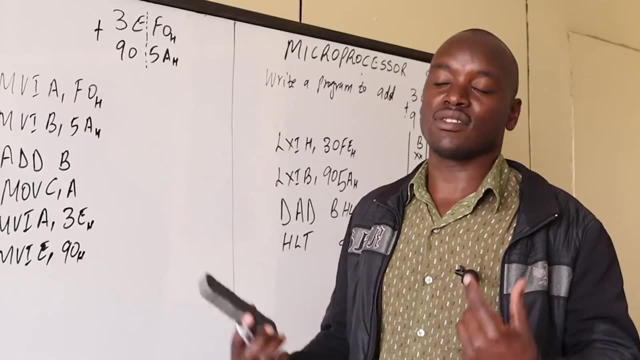 we talked about the auxiliary carry flag, we talked about the party flag, we talked about the sign flag and the zero flag. So if there is a carry, we agree that the carry flag would be set or would be at logic 1, indicating a. 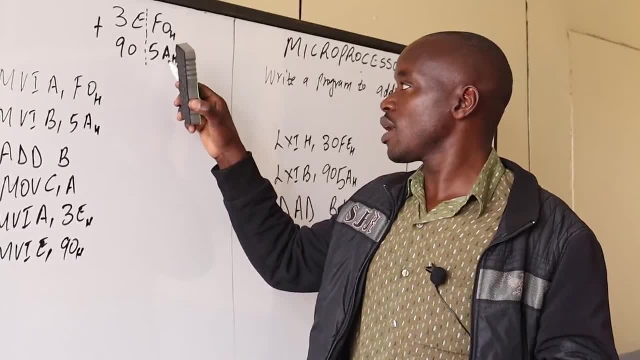 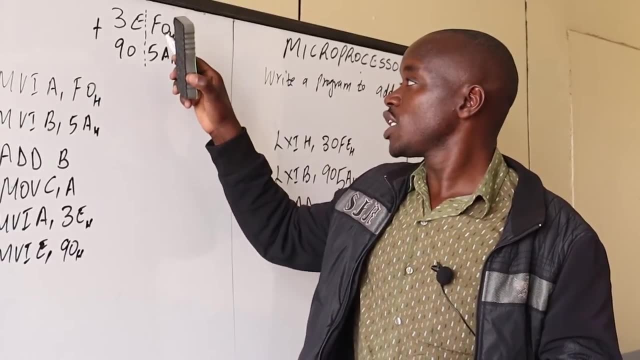 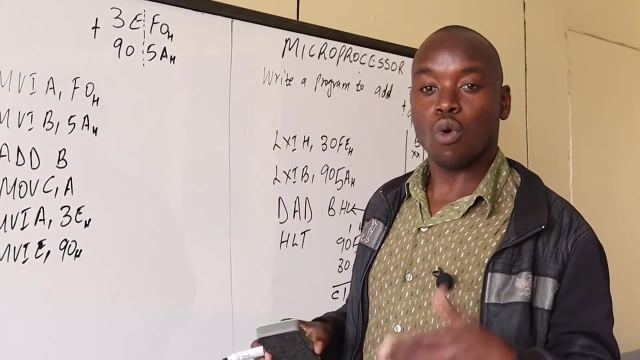 carry, as occurred. For example, 0 plus A is A, but F, which is 15 plus 5, is 20.. So 20, if you now check here, 20 minus what? 20 minus 16 would be 5 carry 1.. 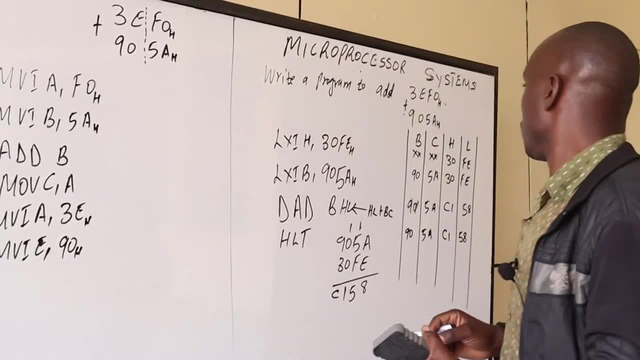 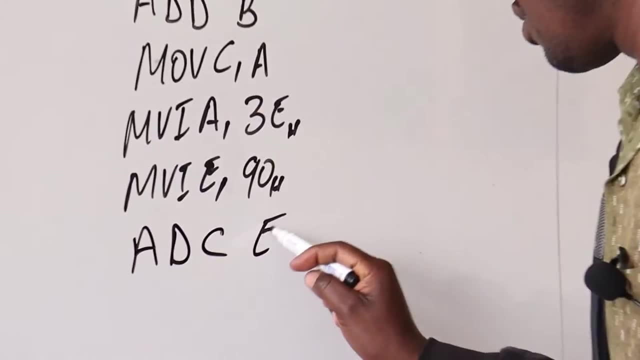 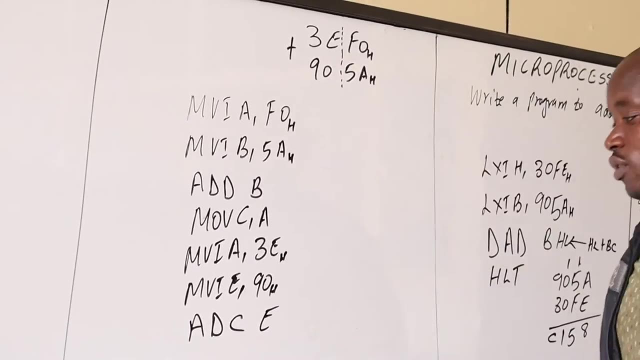 So now what happens here is: let us check, Let us see what will happen here. So I have to come here and say: add: with carry, what register E? So it will check whether there was a carry here and then remember the carry. So then 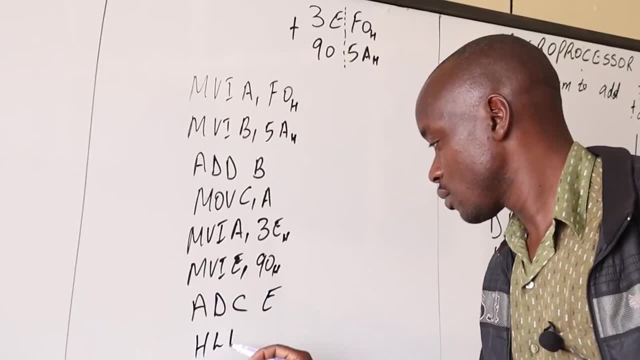 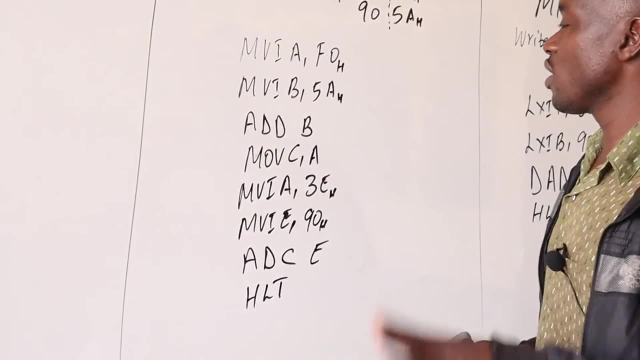 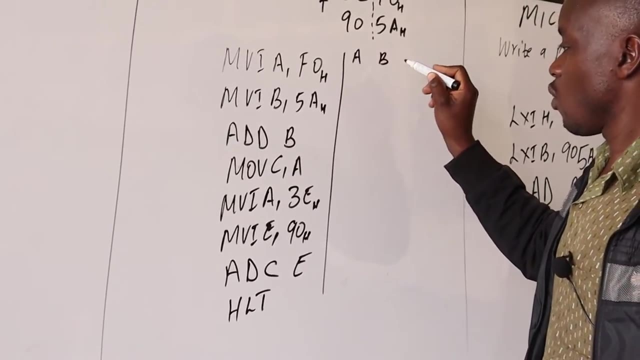 here. now we stop. after doing that Again, we draw the truth table to show what was happening in each instruction execution, So that at least candidates can understand. So we have register A, we have register B, we have register C, we have register E and 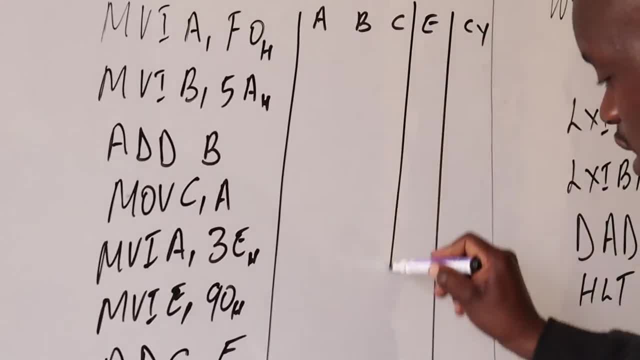 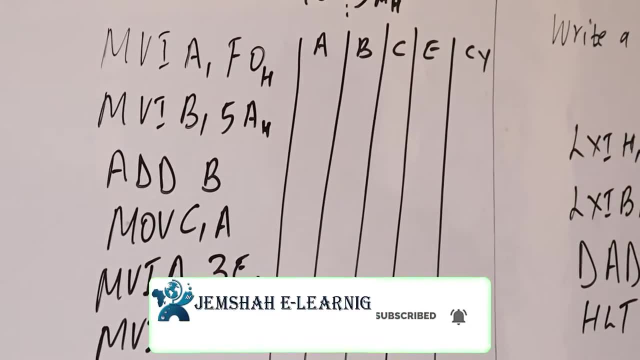 we have to remember the carry because we have to indicate that during addition, if there is a carry, the carry flag will be affected. Let us start the truth table. The first instruction is: move immediate A F0.. So we know that in A we have. 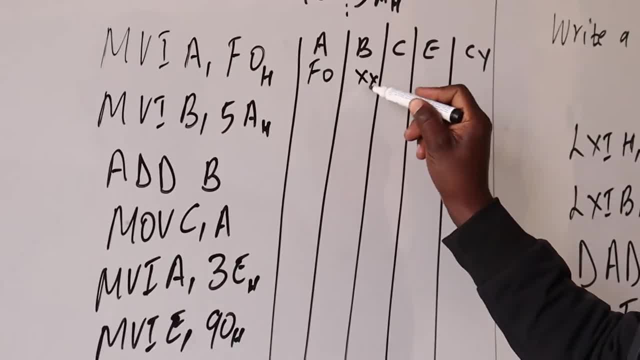 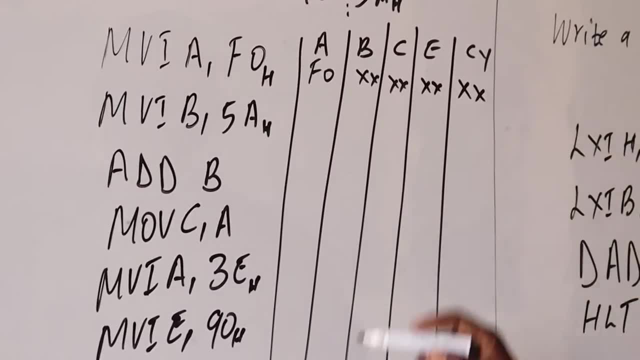 F0.. Here we don't know what is there, So we put it on the case Here. we put it on the case Here. we put it on the case Here. we don't know if there is something, So again we put it on the case. 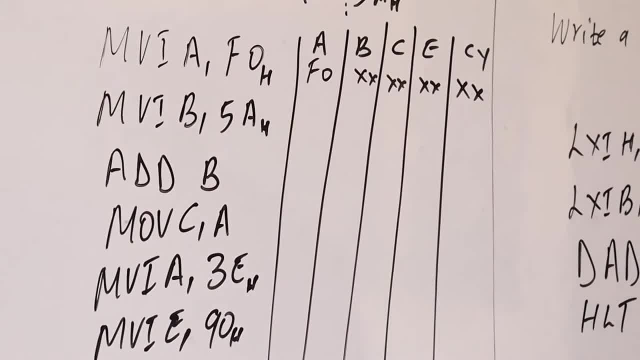 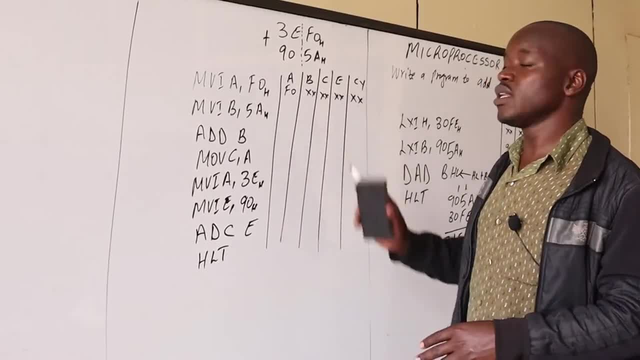 Unless we are sure that a register has some data, Don't put anything there And we are not going to put 0 because we don't know if somebody used these registers. So in digital electronics we, or in microprocessor we use, don't case. 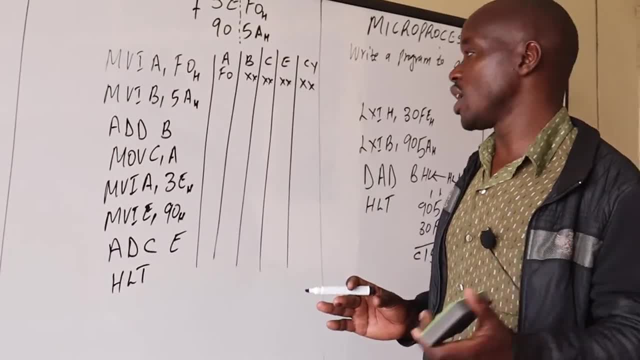 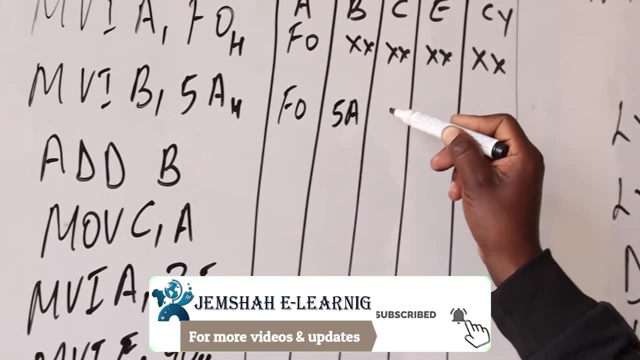 to indicate that we are not sure. if there is data or there is no data, Then move B 5A. Now we are sure in A we have F0.. In B we have 5A. We don't know what is in C. 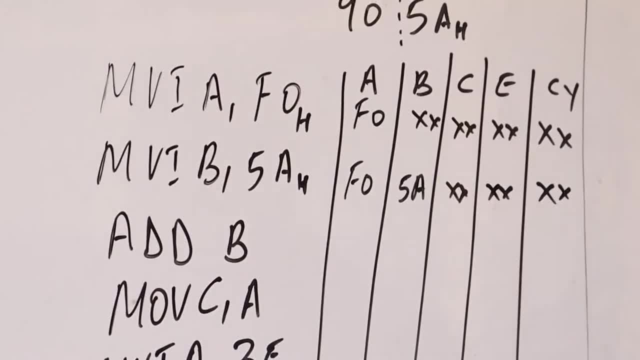 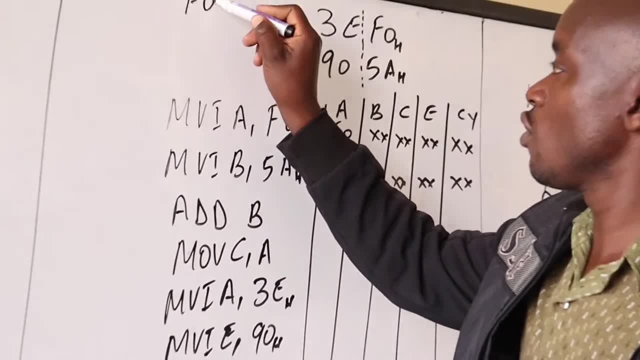 We don't know what is in register E And we don't know what is in the carry flag. Now the next instruction is add B. What will happen? Add B means whatever is in A, which is F0 plus this 5A. So let us. 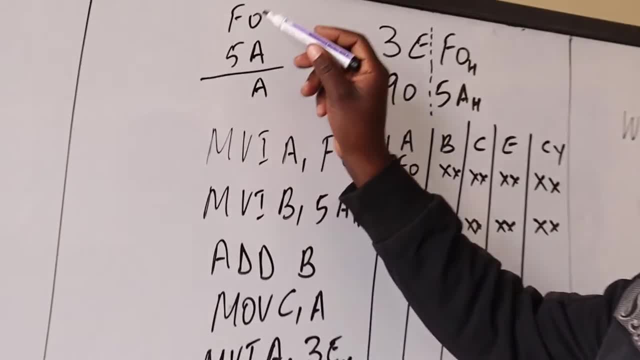 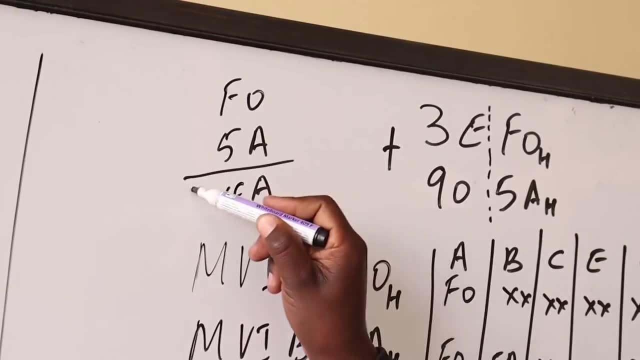 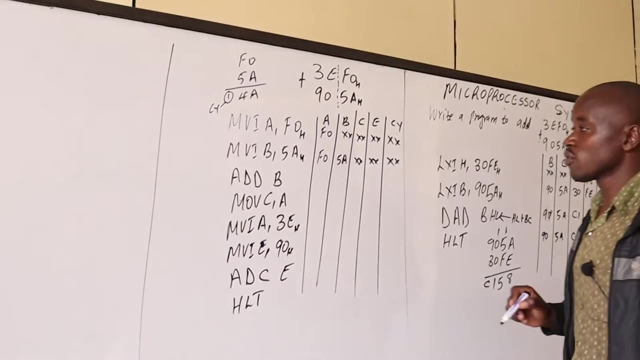 see, This one will be A 5 plus 5 plus 15. It is 20 minus 16 is 4. Carry 1. So this 1 will go to the carry flag. So now we know what is in the carry flag. So the 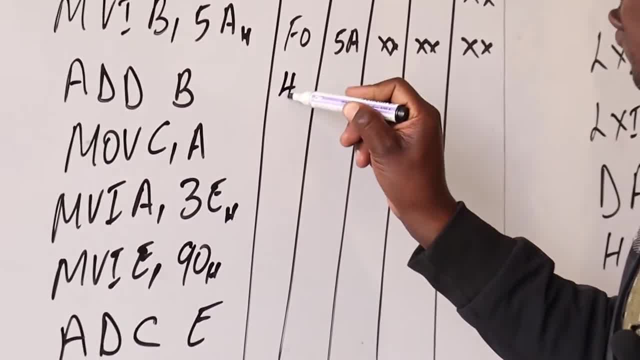 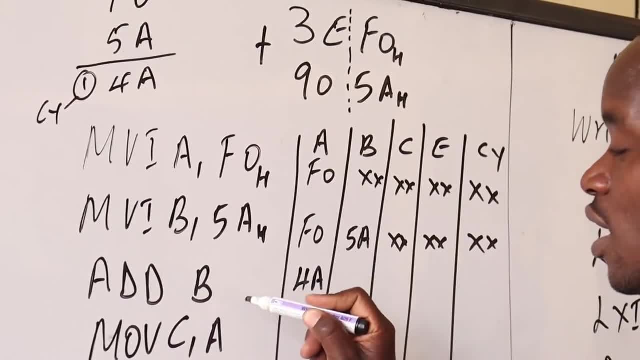 carry flag will be F. in what? Here now we have the result in A will be 4A, because now they are after addition. Since we agreed that add B means whatever is in A plus what is in B, the answer goes back to A. So here, 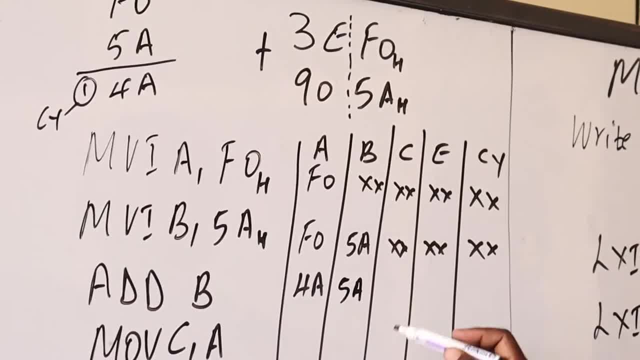 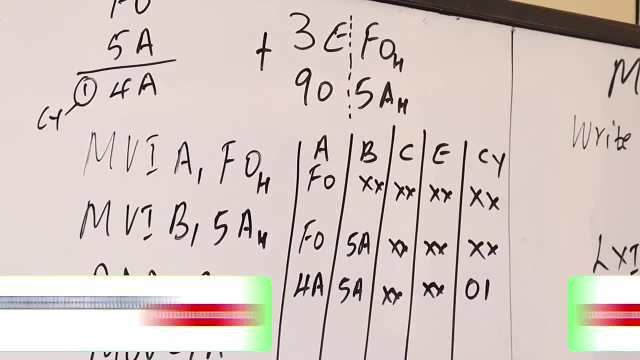 we have 4A Here we have 5A. We don't know what is in C, We don't know what is in E, but we are sure that the carry- now there is a carry in the carry flag. So the moment the 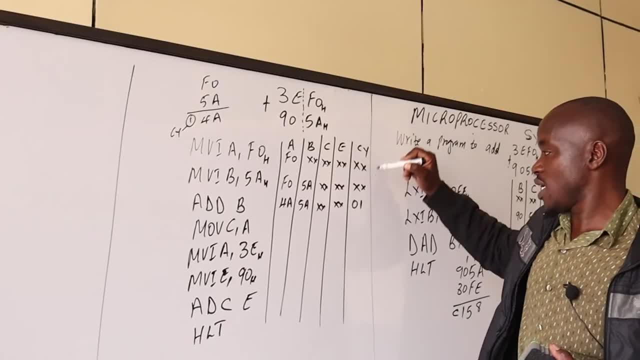 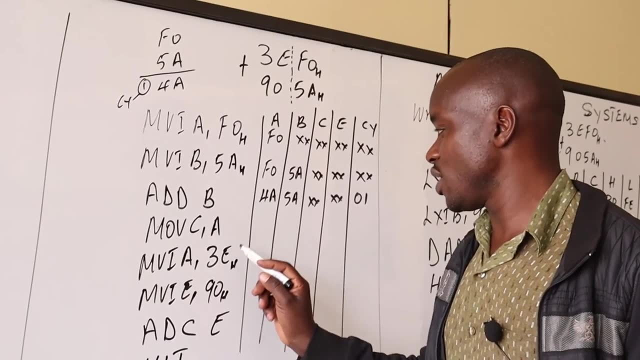 carry occurs. now. what I want you to see as a candidate is: the carry goes direct to the carry flag. Otherwise, copy the result from whatever is in A to C. Now we are sure in C we have something, Here we have 4A. In C we have 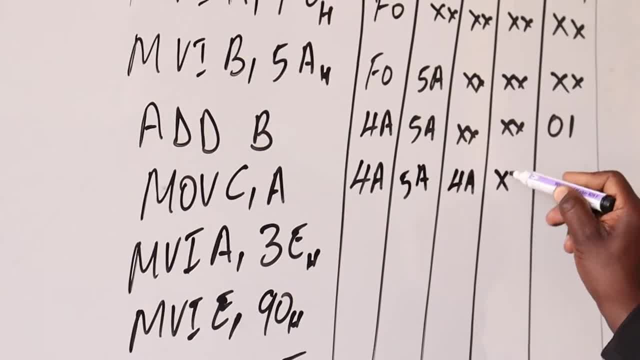 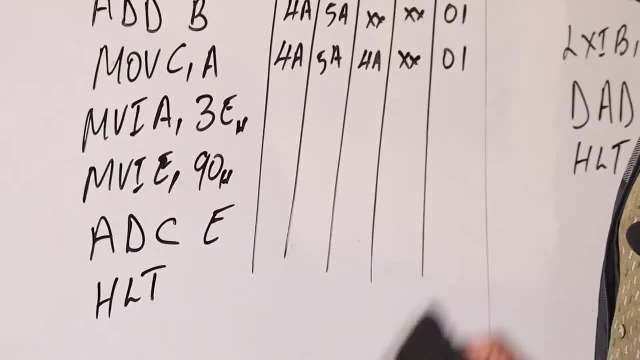 also 4A. Here we have 5A. We don't know what is here, but we have the carry Next instruction, Move immediate Register A 3E. So now we are sure, here we have 3E. Here we. 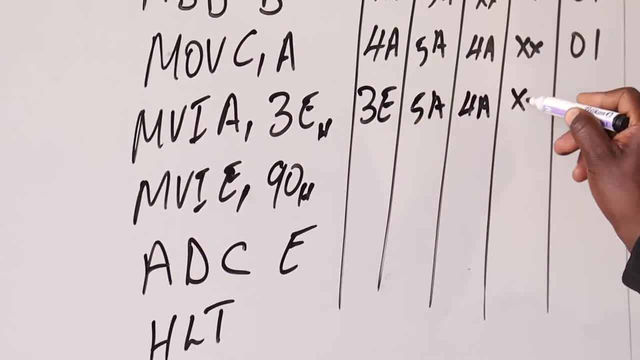 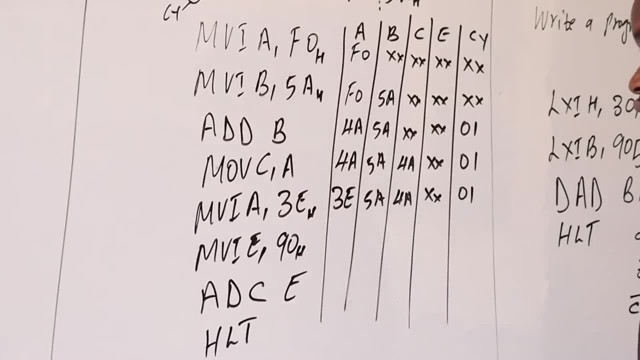 have 5A. Here we have 4A Here. we don't know what is here. Here we have the carry Next instruction: Move immediate E 90.. So here now we are sure that in A we have 3E. 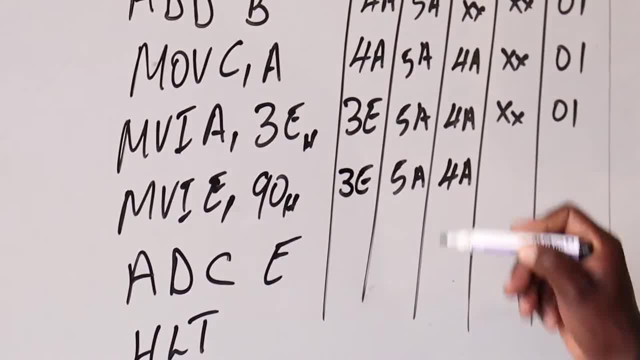 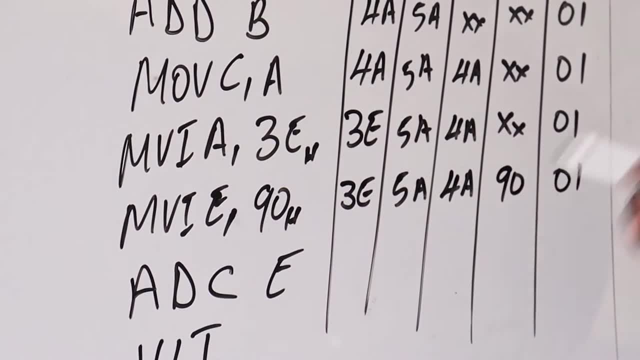 In B we have 5A. In C we copied 4A there E. now we are sure that is what 9-0.. And then we have the carry in the carry flag. Now check the next instruction. It says what Add. 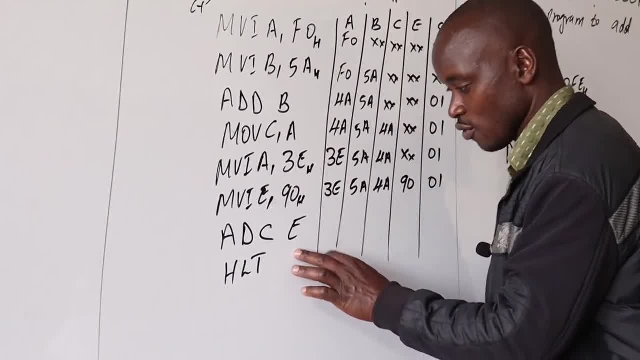 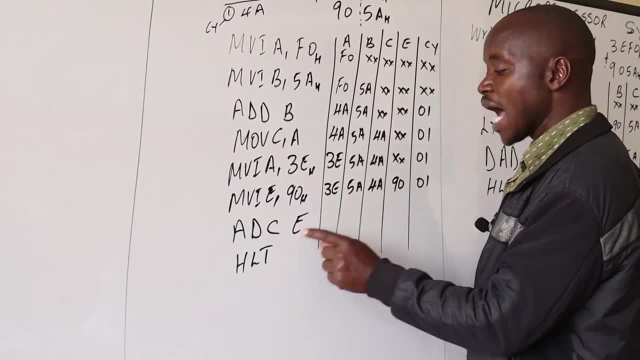 with carry register E. So it means this way: We check what's in A, which is 3E, We add what's in E, which is 9-0. And a carry in the carry flag 3.. So it will be. 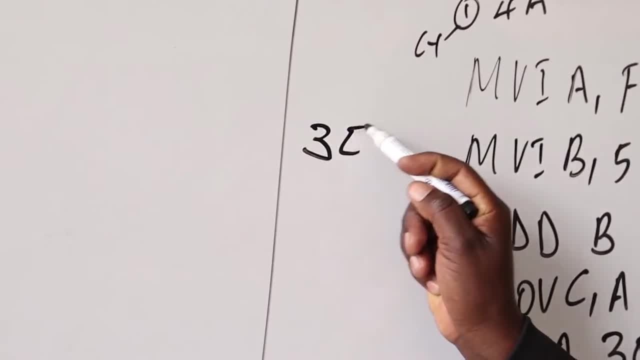 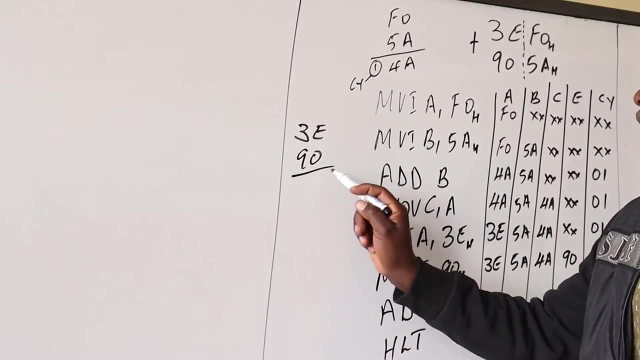 3E. I want to do it here so that you see It will be 3E in register A plus 9-0 in register E. So we get E and C. And then we remember the carry flag. There is a carry in the carry flag. 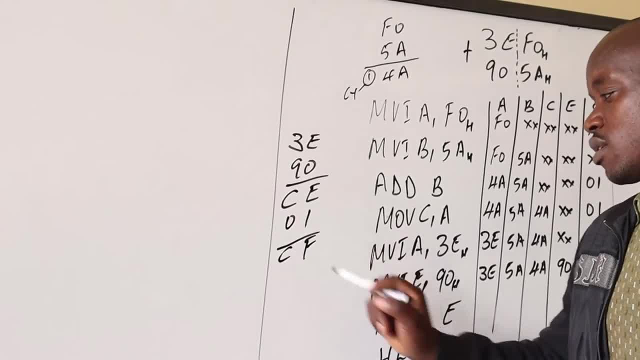 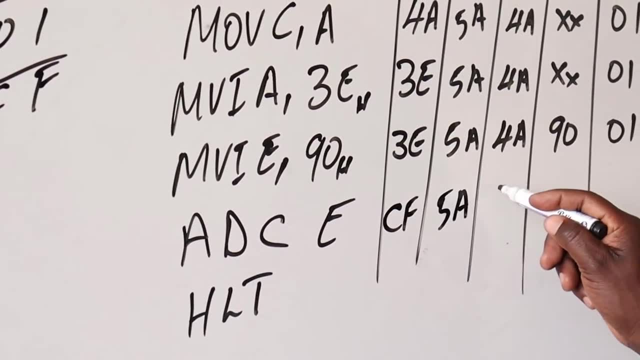 0-1.. We get F-C. So the answer: here now: in A we have C-F, Here we have 5A, Here we have 4A, Here we have 9-0.. And since the carry flag has been added, 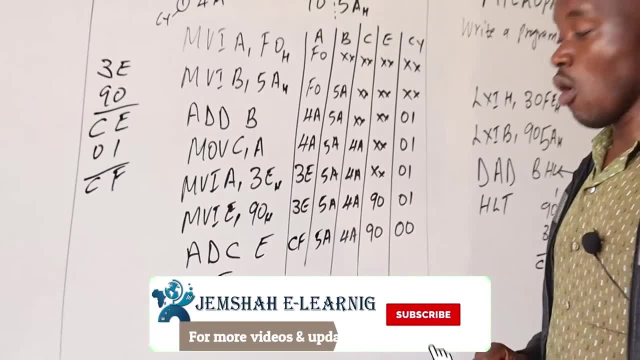 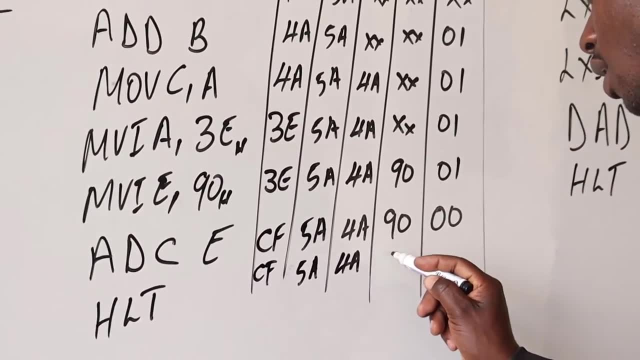 we remain with nothing in the carry flag Now when we stop Halt. So in A we have C-F, Here we have 5A, Here we have 4A, Here we have 9-0.. And here we have 0-0.. 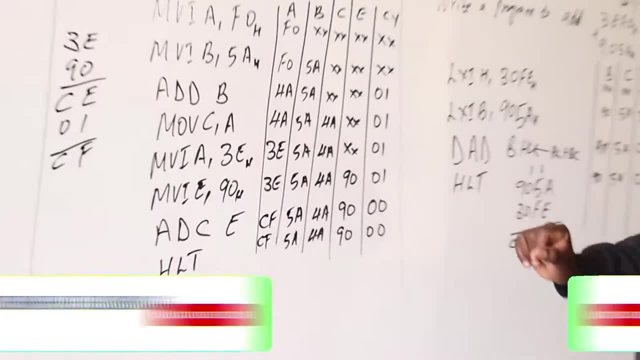 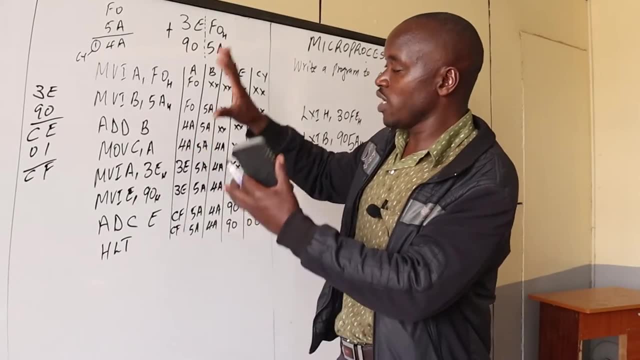 So now this is our trace table of this program. So I've done it two ways: Using register pairs: this is the way By using that instruction. Using registers: this is the way By using add B. I hope that by the end of the exercise, 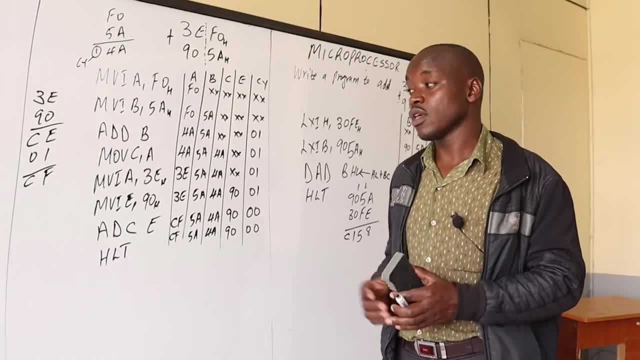 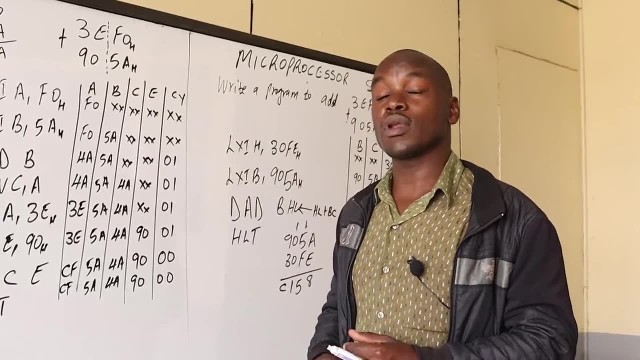 a candidate who is supposed to sit for easy exams or high exams should understand what's happening in this program. And once you understand these basics, even when you want to do the program which they call C, it will be easier for you to understand, because now you have already. 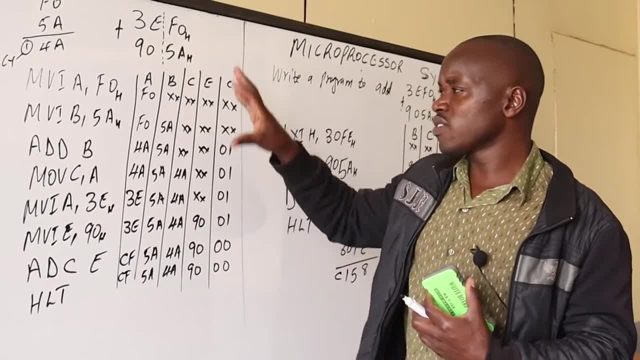 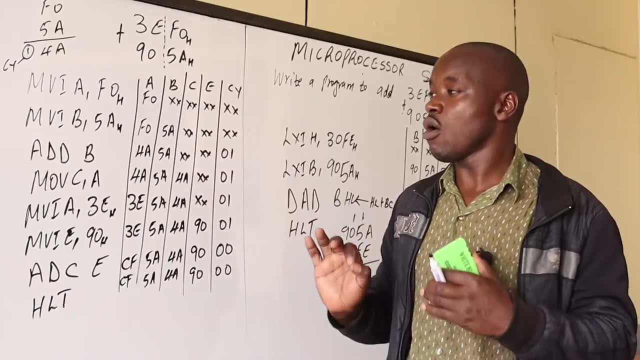 the basics of programming. Now, what's remaining out of this program maybe we have not done and we don't do today? is we need now to do what's called hand-decoding, or writing the x-decimal machine code using the instruction set? So as we are proceeding, 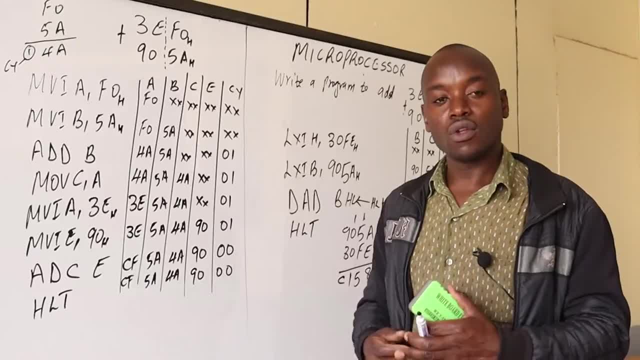 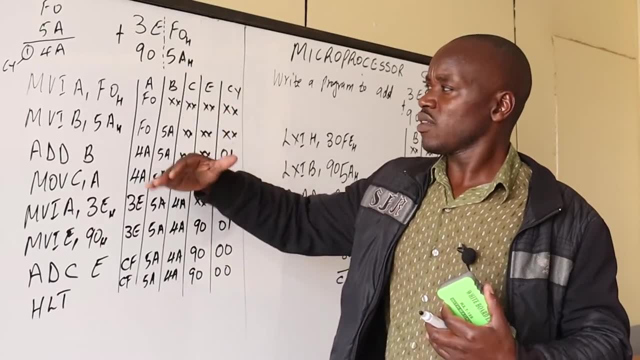 we shall see, or we shall use the instruction set to write what Programs Today. I told you that we are doing several examples, so that the three programs that we are doing are three examples, So at least you can understand how this microprocessor is easier. 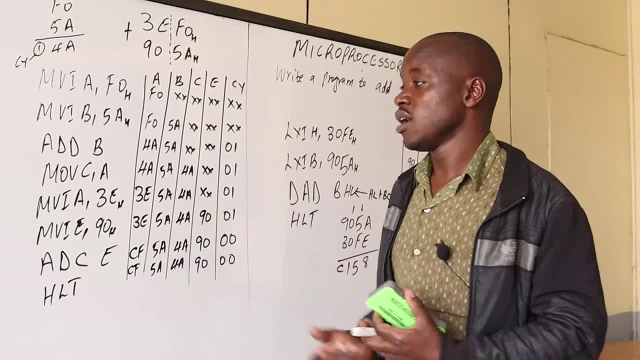 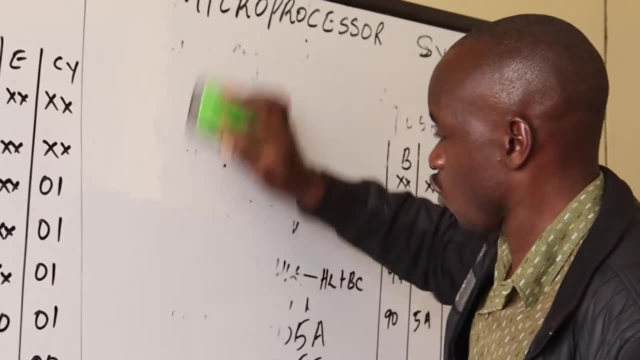 and does not have a lot of difficulties, the way people tend to think. So I want to do another example here, example two and the microprocessor programming. now Example two is to do the following operation: Let me just reset my accumulator here. 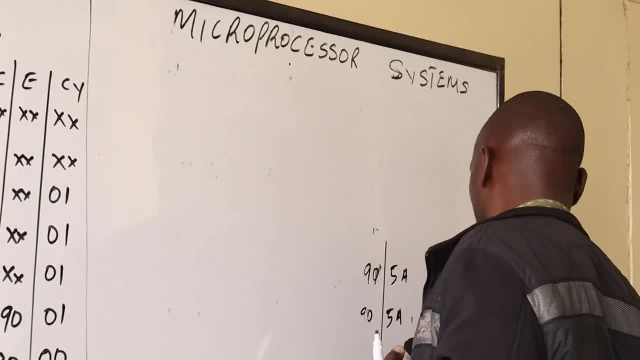 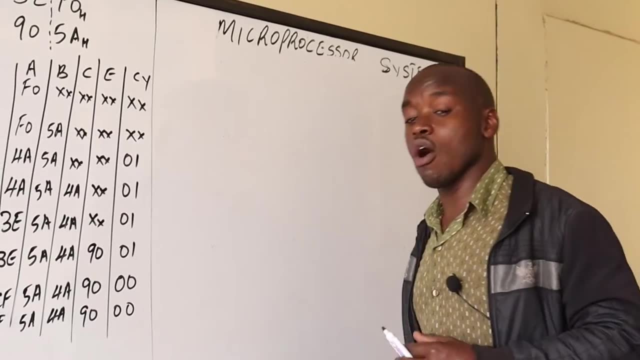 My accumulator is a board, So that now again we do another question We see, So that at least before the lesson ends, at least someone who is checking in our YouTube, it will be easy for her or for him to understand this program. So the second one. now I want us to do this: 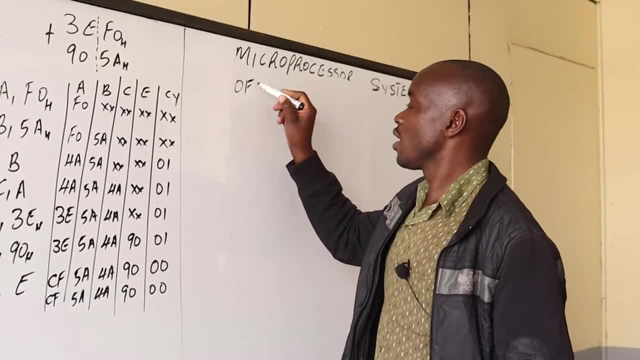 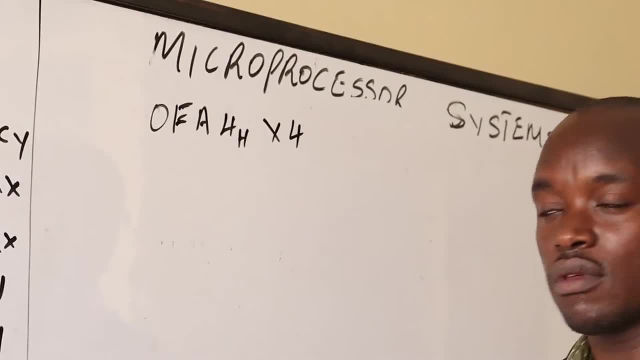 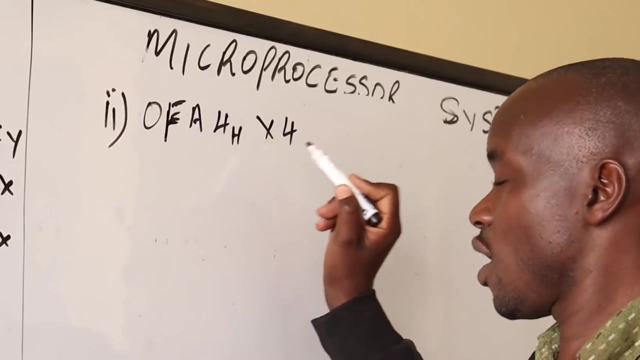 An operation which says zero, F A four, maybe H times four. You write a program to do that. So write a program to do the operation of one, two, zero, F, A, F times four. Most of the time the candidate sees this, then they will start wondering. 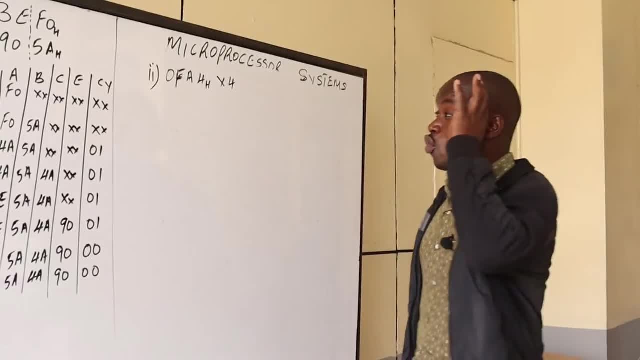 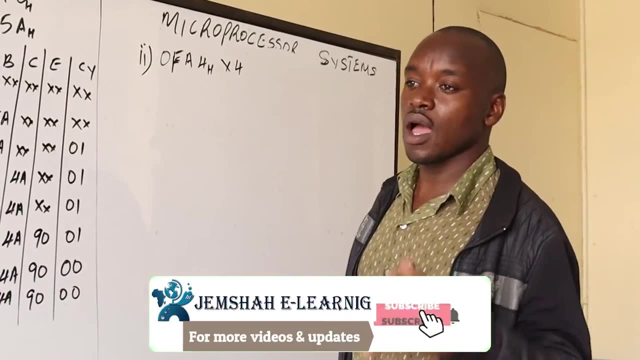 what are we supposed to do here? So I want to show you what happens, What we do already. We know that this data is 16 bits, So, since it is 16 bits, we have to use what Register pair, Now our register pair which can be used for addition? 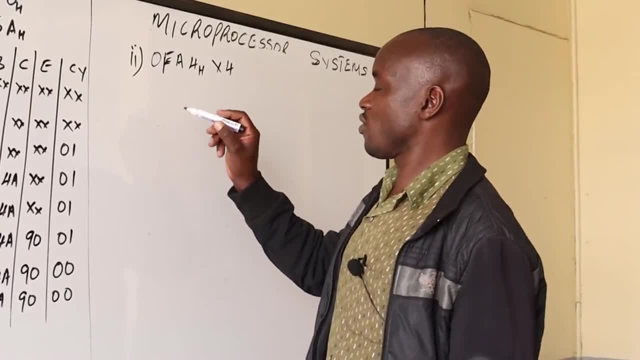 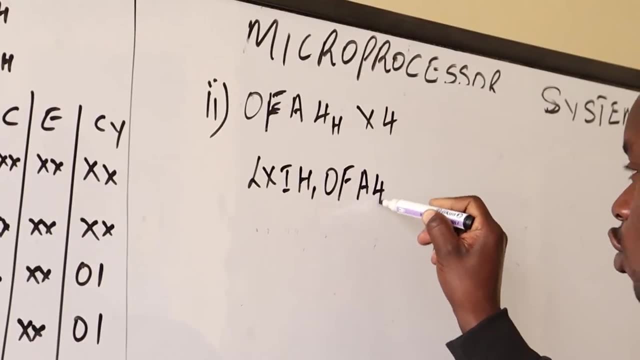 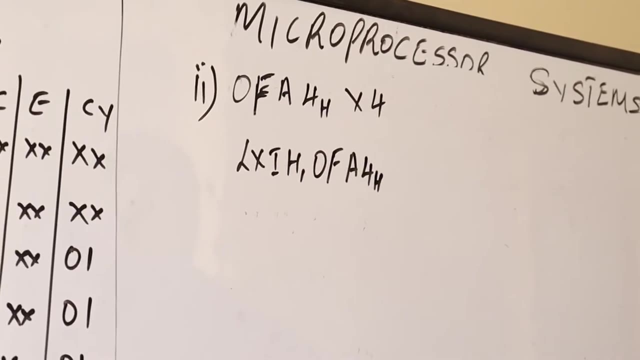 is register H, L. So what do we do? We come here and then we say R, X, I, H, zero, F, A, four, H. So I have initialized this data 16 bits to register H. Then I ask myself: I cannot multiply a 16 bit data by two. 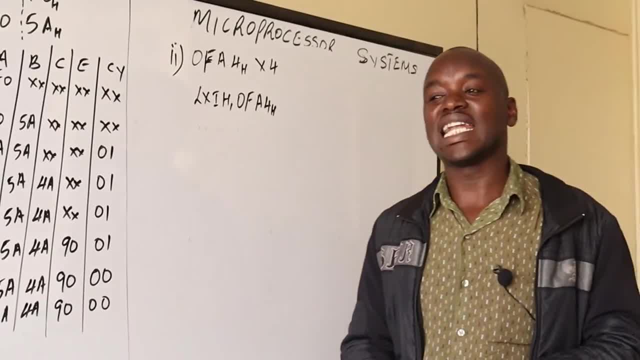 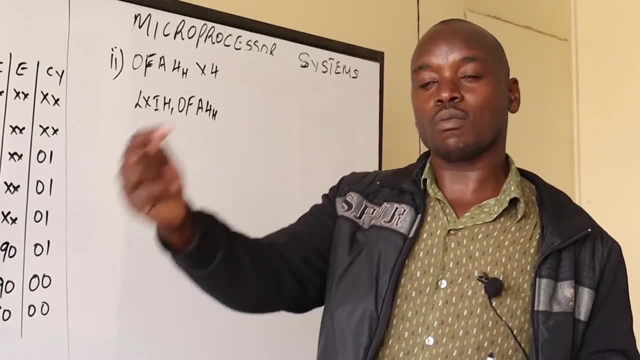 What am I supposed to do? So I remember this in strong, which is known as DAD Double addition. So I say DAD H, which means whatever is in H L add what was in H? L. the answer goes back to H? L. So I come here and then I say DAD H, DAD, DAD H. 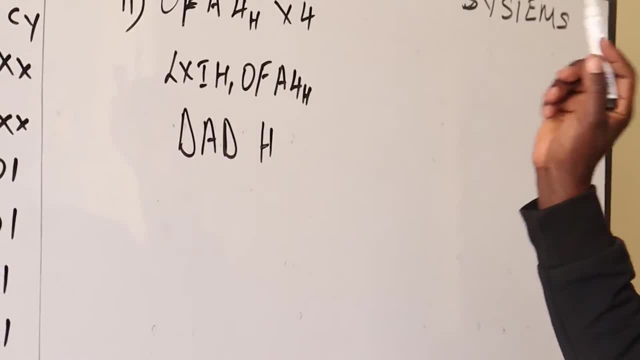 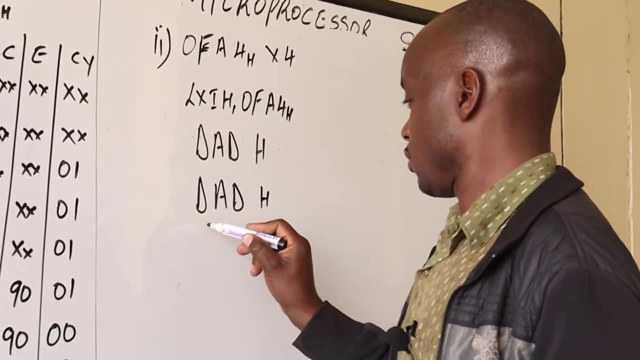 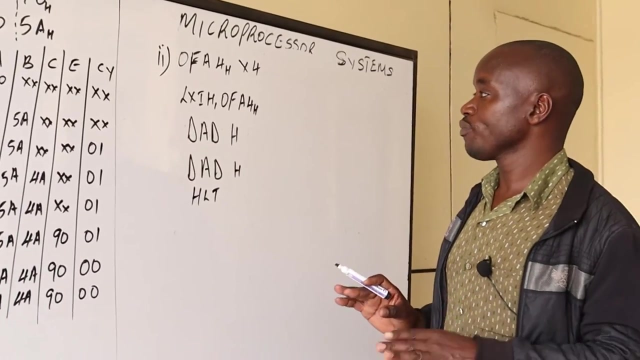 That's multiply by two. Our equation was multiply by four. I DAD H, again DAD H, Then I stop. I alt. So if you are a kid now, let me now try to show you what's happening. It is. I initialize this data: zero, F, A, four. 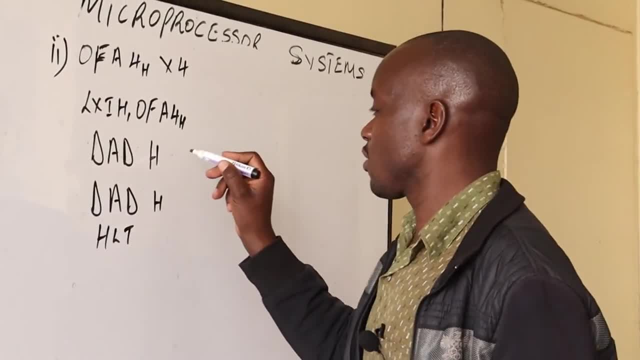 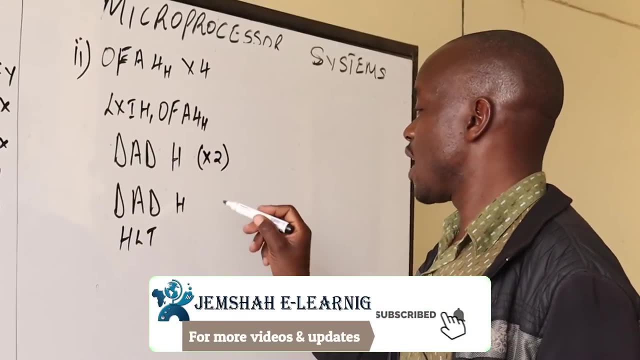 into register pair H L, DAD H in the bracket. let me put in the bracket so that people but in the exam don't do that way. It means multiply the data in H L by two DAD H again. it means multiply the data here by now four. 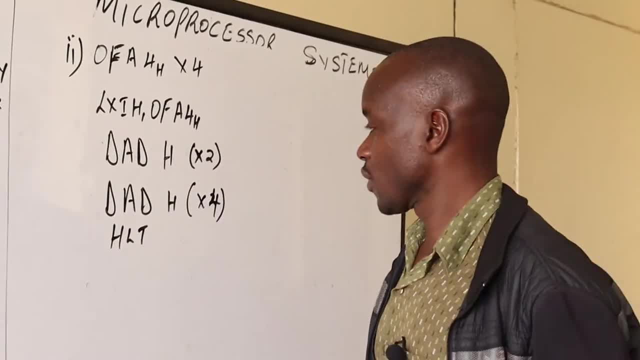 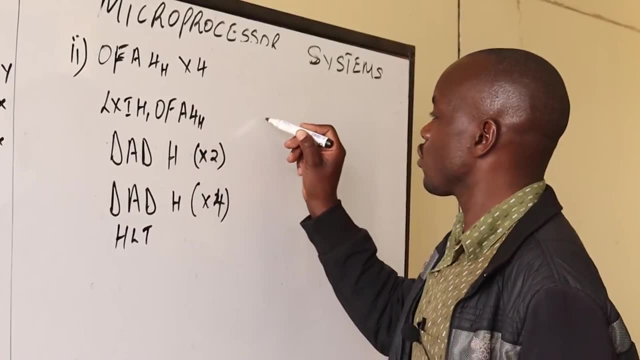 Because if DAD H, it is H L plus H L times two, Again DAD H. Now already what was in H L has changed Like now. let me show you practically what's happening here. So we have zero F A F plus zero F A F. 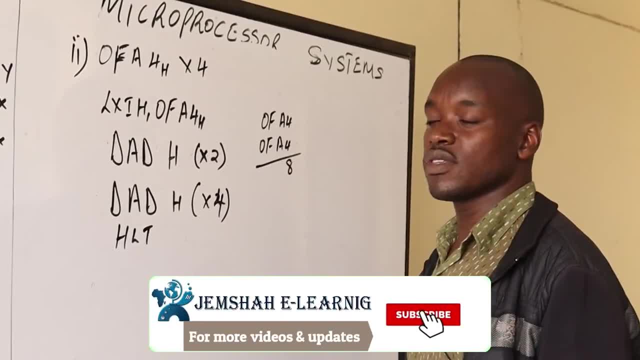 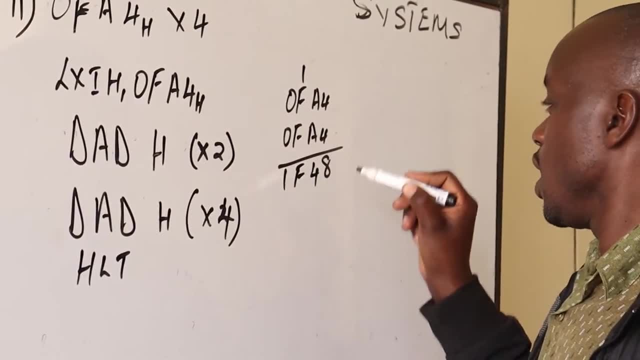 So here we have eight. This is 20 minus 16, should be four. carry one Already. this is remainder F. carry one. That's the first one. So if you are a kid, if you check, if you change two into a decimal and you multiply by two, 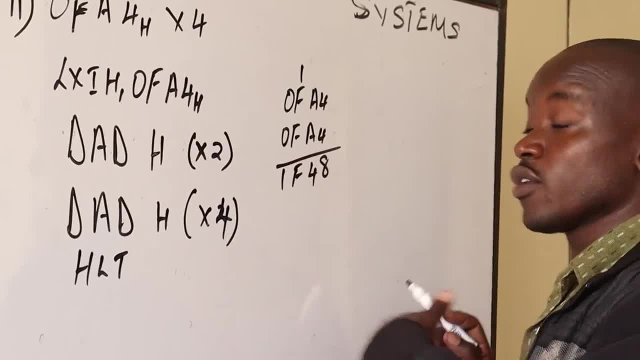 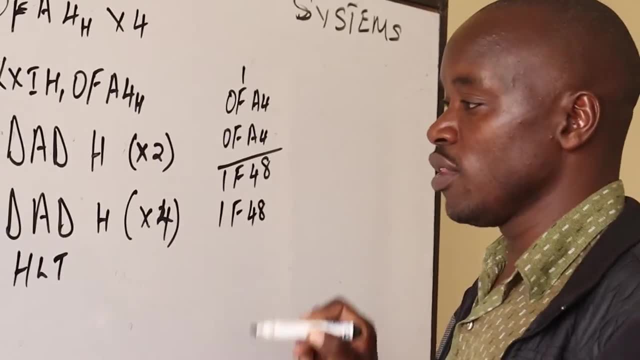 you can get this one, F, four, eight, which we can convert to decimal again. Then if you have a cross assembler, then we have again a DAD H. Now this DAD H is this second one, which implies already H L has changed from zero. F A four. 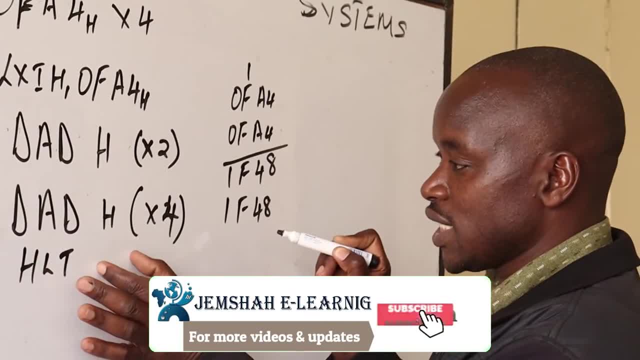 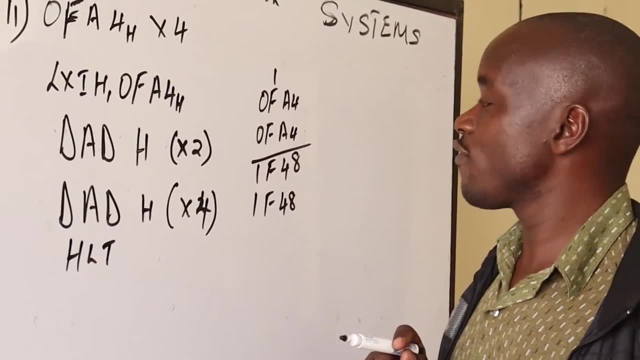 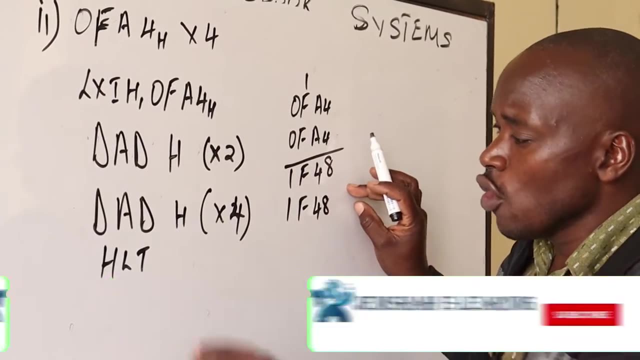 to one F four eight. Again DAD H. So what I want you to understand as a candidate, the first DAD H was zero F A four plus zero F A four, But now already H L. it has changed to one F four eight. 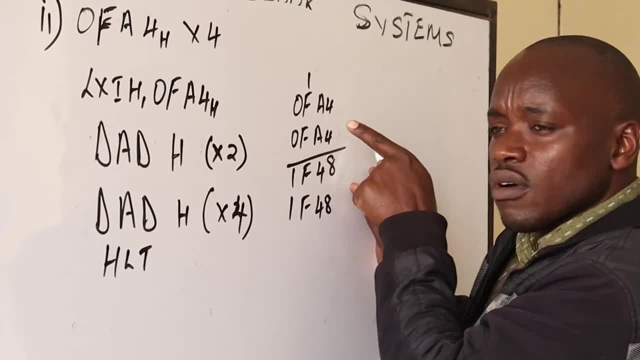 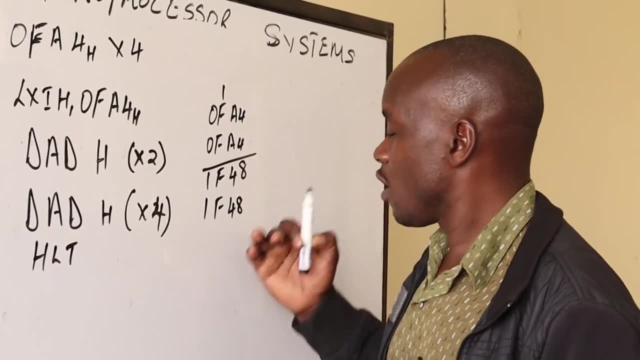 So when we say DAD H here, it's not zero F A four plus zero F A four, It's already changed to one F four eight. So we are doing one F four eight plus one F four eight. So basically this time is two. 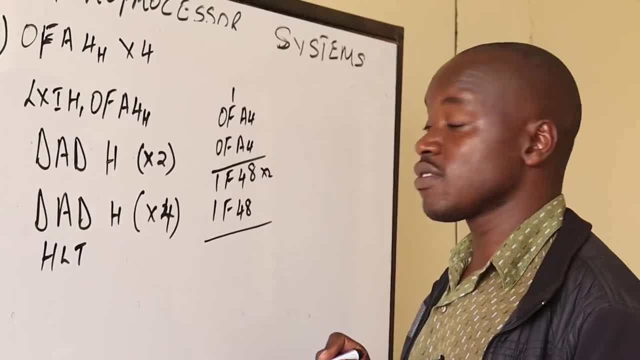 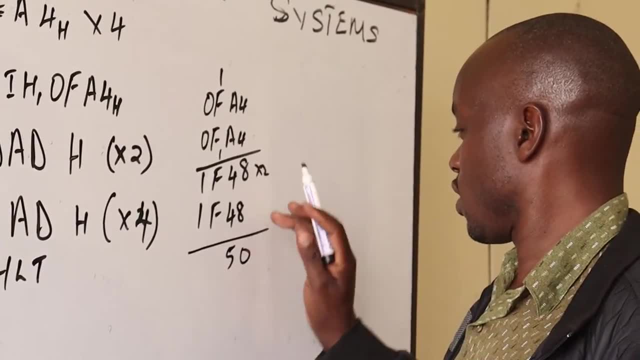 And now this one is times four, So we should get eight plus eight is 16, zero. carry one five. carry one here. This should be. let me see: This is for eight, eight, zero. This is five. there's no carry. 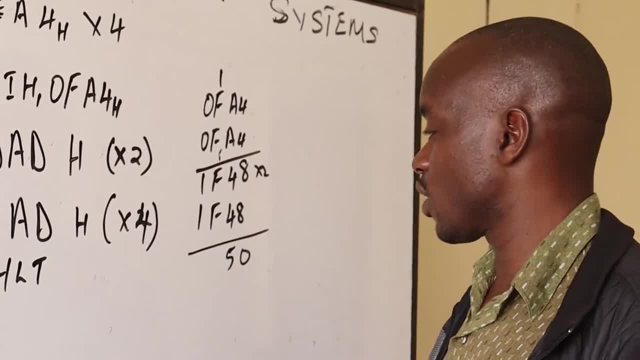 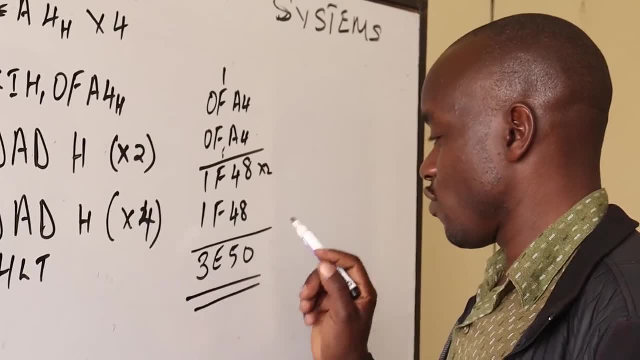 F plus F, that's 15 plus 15.. That's 30 minus whatever. it is 14, which is E. Then carry one three. So the answer is three E, F, five, zero H. So what I want maybe someone to confirm? 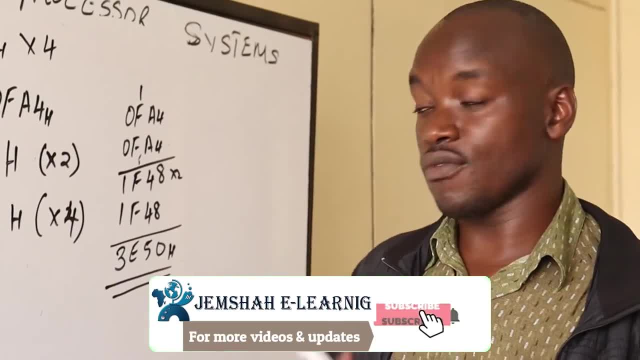 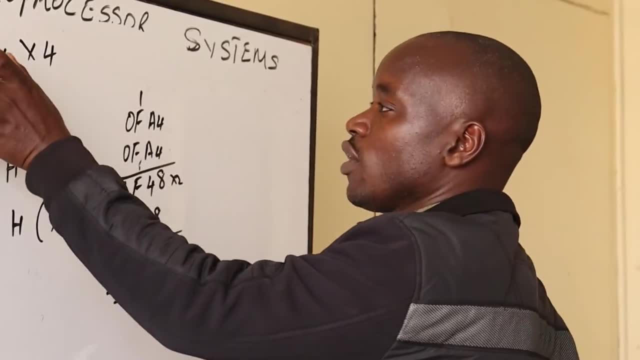 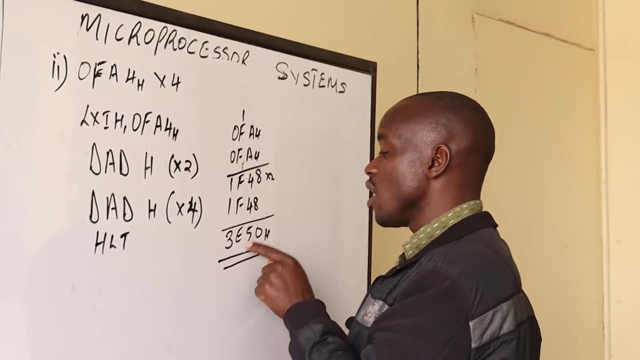 After you have checked our lesson and we have seen what we have done After this, what you do confirm: if three E five zero, You convert this one to decimal. you multiply by four. Then you change the result Into hexadecimal. You check if the answer is the same as three E five zero. 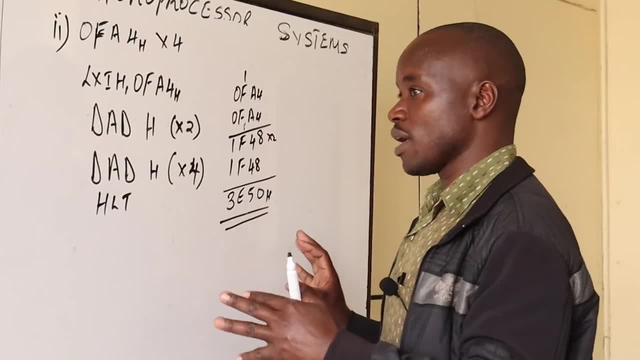 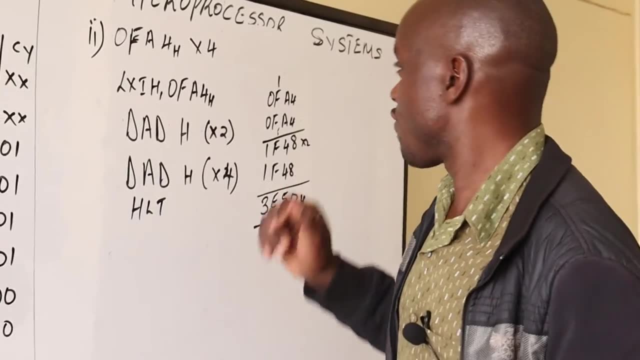 So by that way, now we can understand that we are multiplying the number by four. I want to add more. one more example here Want to do. I've remembered another instruction which way I need to introduce here so that people might not be suffering. 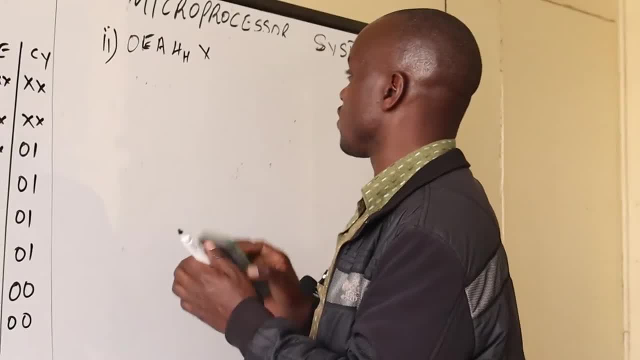 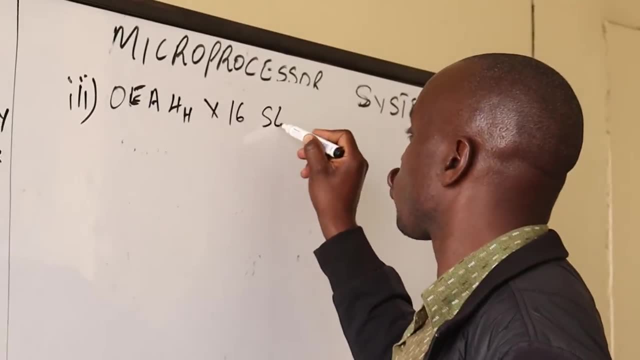 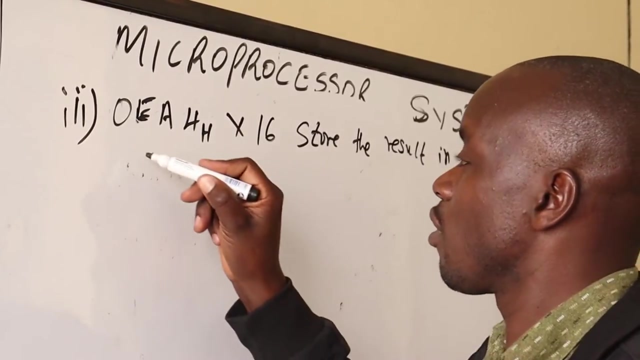 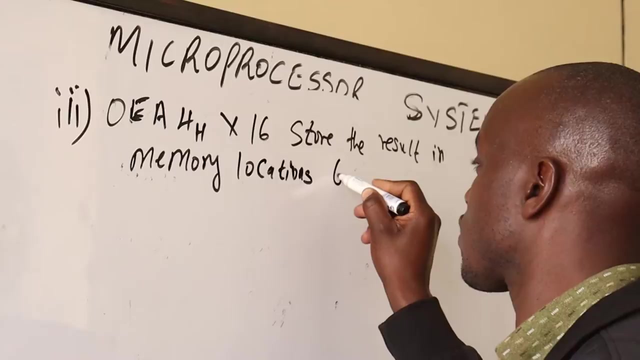 What if it was the same number multiplied by 16.. This same number multiplied by 16, now Roman three, Multiply by 16 and store the results in memory locations. I want to add soup here In memory locations 6,000 H and 6,001 H. 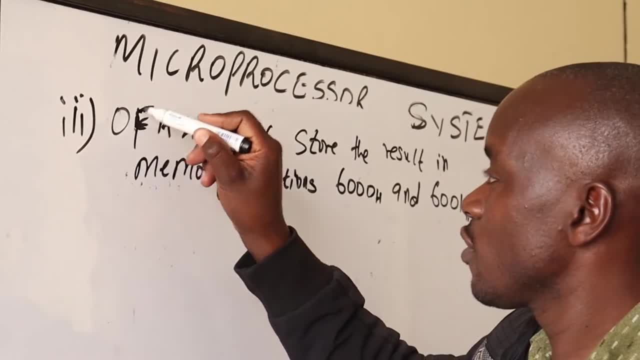 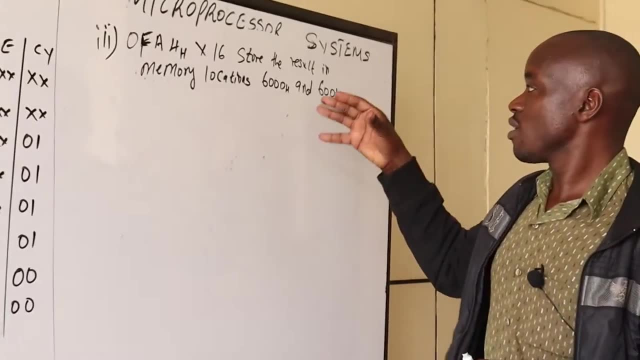 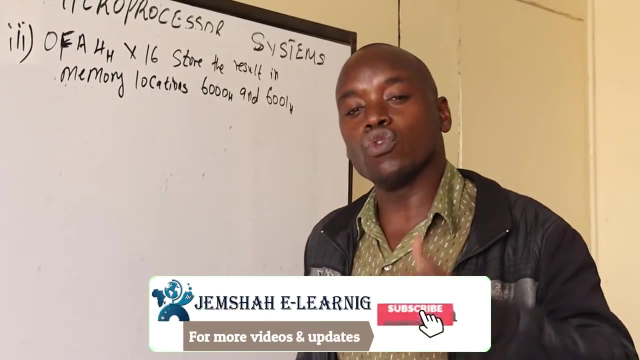 So we multiply this: the same zero F A, four H times 16.. And then we store the result in memory location 6,000 H and 6,001 H. Now, if you see that we have been given two memory locations, 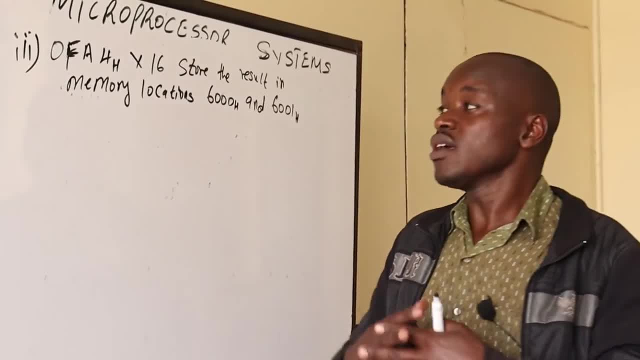 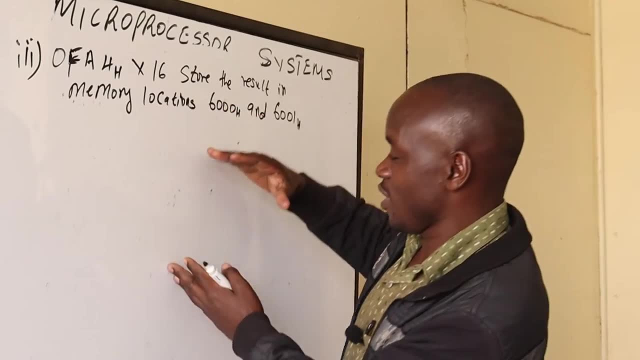 it means the result we are going to do is in 16 bits, And I think I will do this one Then. after doing this one now, which means you could have understood something, I will stop to the next one. I will come again and introduce more instructions. 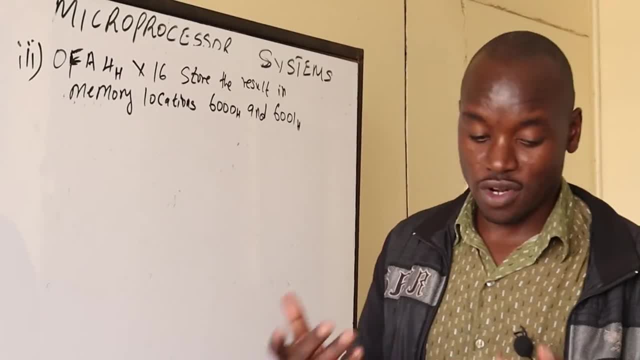 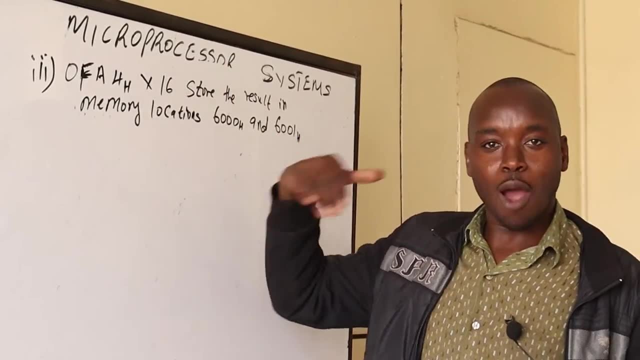 But I want to introduce a certain instruction here Which some people fear for no good reason. So what we do again, it is: we understand. the equation now is- I've done already: zero four A four times four. I want to show you: zero F A four times 16.. 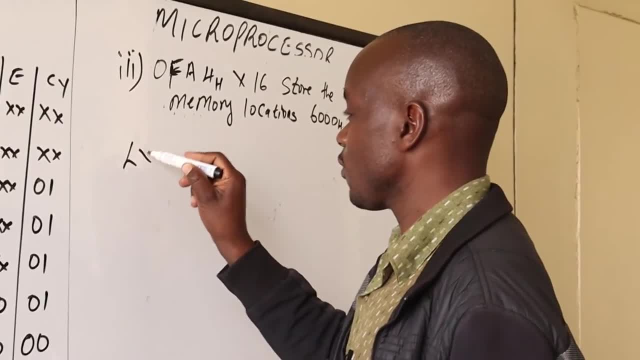 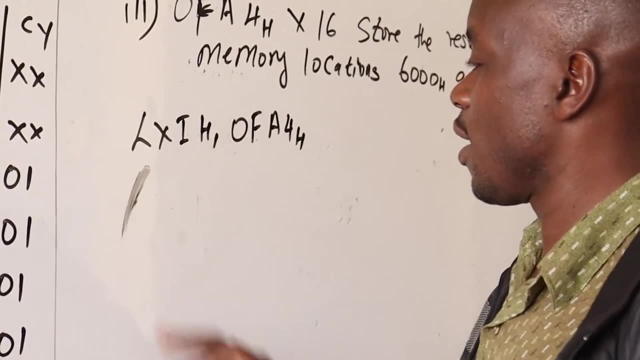 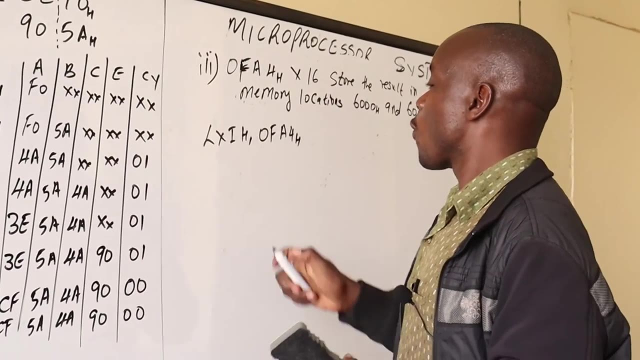 What am I supposed to do? So again, I say LXI, H, zero, four, A, four, H, LXI. Then we are multiplying by 16.. Remember we have agreed that H means multiply by two. So what do we do here now? We add H, Add H. 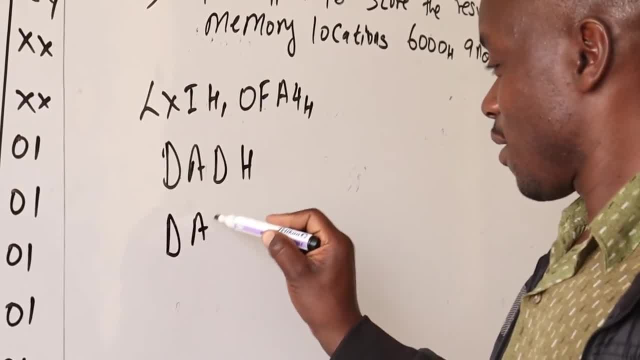 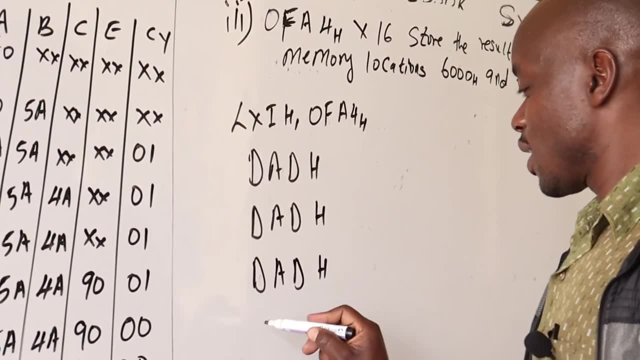 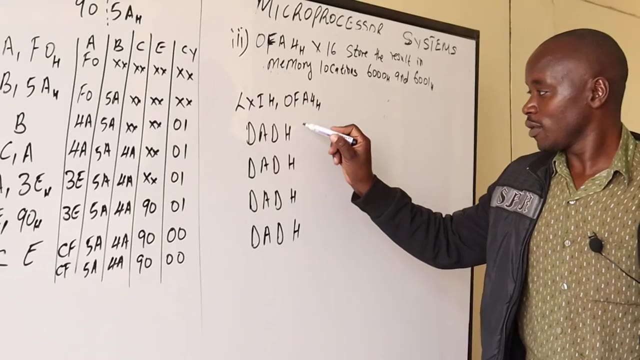 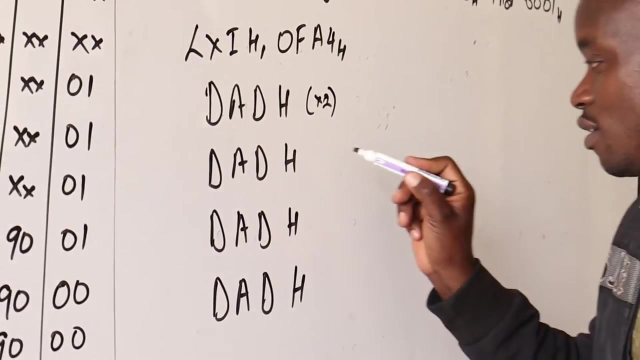 Then this by two, Add H By four, Add H By eight, Add H By 16.. So this by two. Just put that so that when you are revising you understand: This means zero F, A four times two. 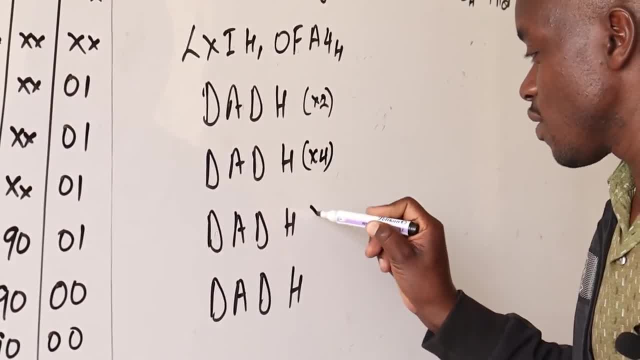 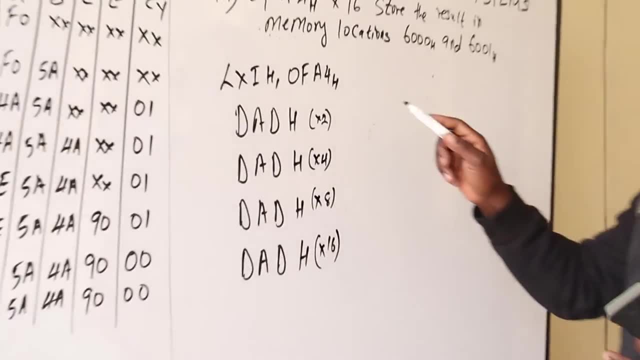 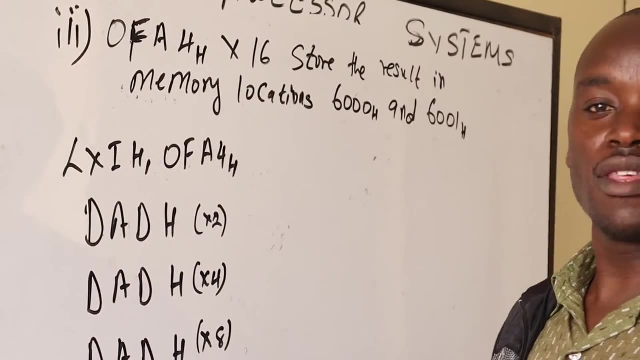 This means times four, This means times eight And two database times 16.. And then we look for an instruction which can take these reset, which is H A to memo location 600 and 6001.. And this one I'll draw the trace table. 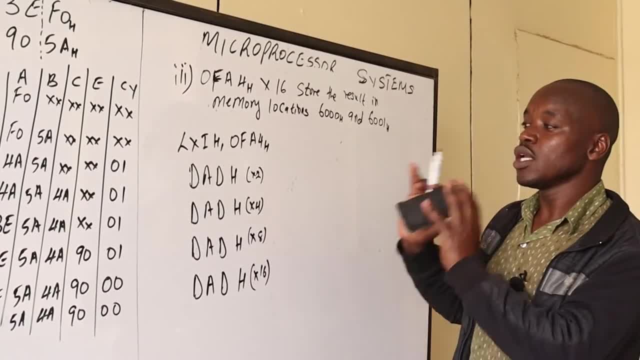 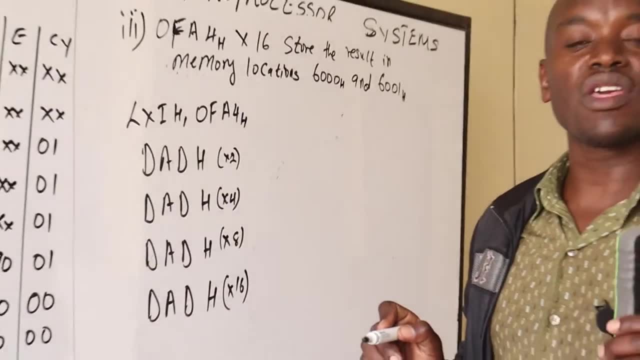 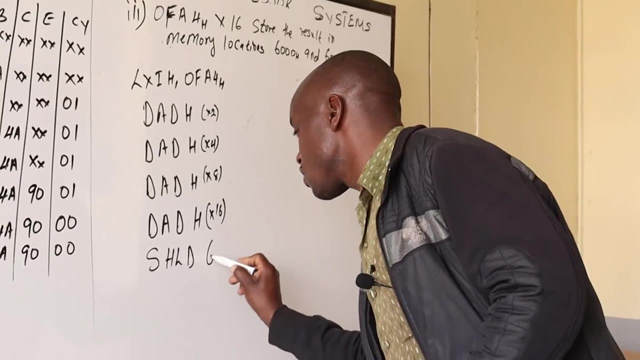 so that now people will understand clearly what's happening in each instruction execution. So now what will happen is I look for an instruction which can take two memory locations consecutively, So the instruction will be store: HL direct 6000H, Otherwise you stop. 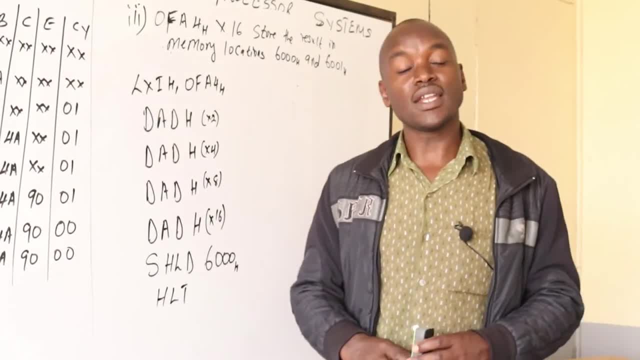 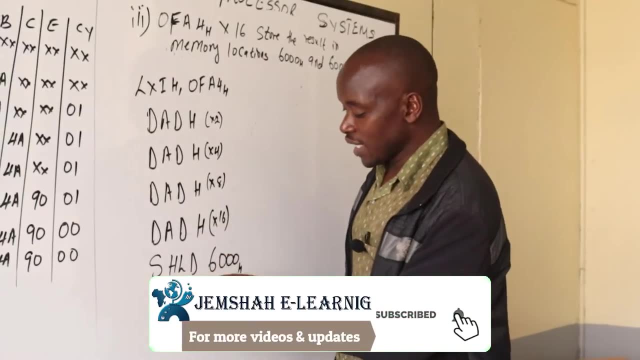 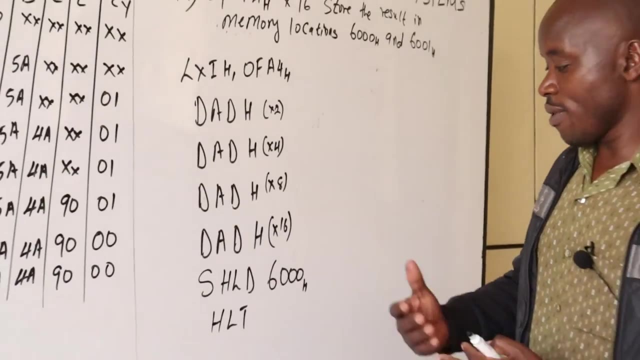 Most candidates, when they see this instruction, they tend to think that it's a very difficult instruction to understand. But what this instruction will do? it will add data in. it will store data in 16-bit data into memory locations, starting the lower byte, followed by the higher byte. 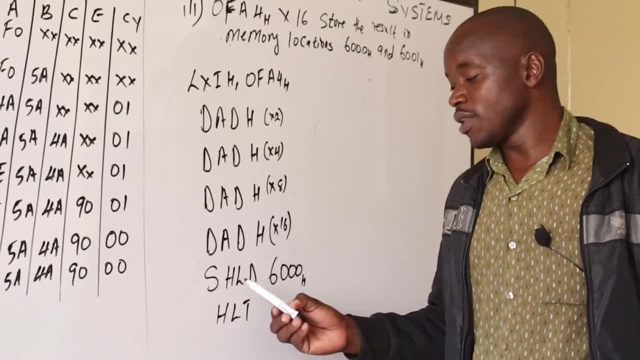 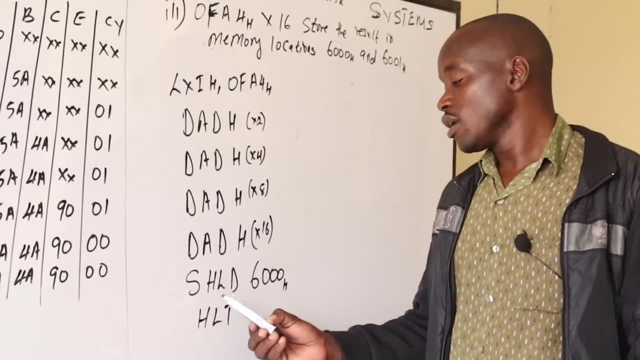 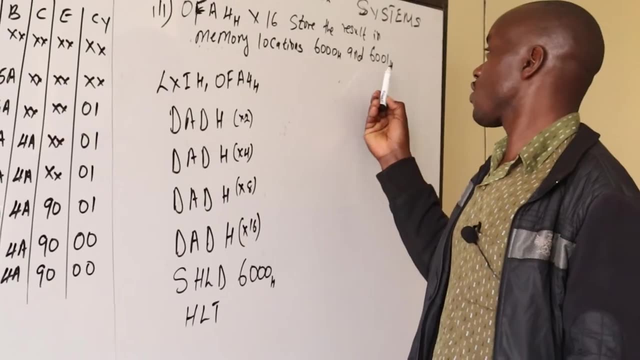 The lower byte will be in register L, while the higher byte will be in register H. So whatever is in register L will go to memory location 6000.. Whatever is in register H will go to memory location 6001.. So now the examiner will change to 5000 to 5001. 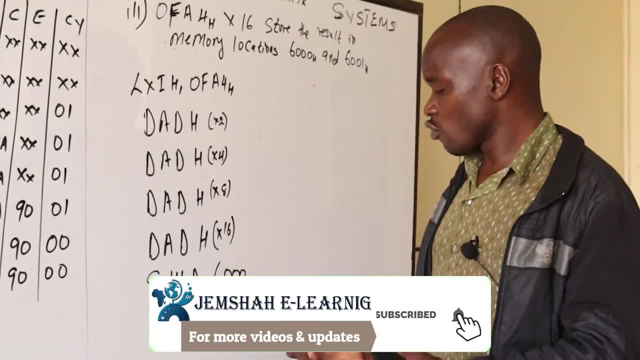 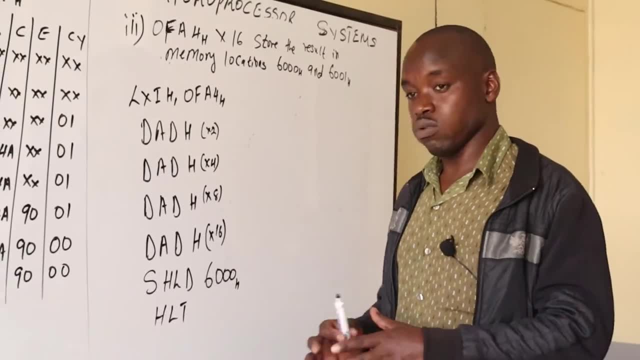 The same program will run that way, But the difference will be: now, instead of 6000, we say store HL direct 5000.. So before we stop, let us draw the trace table so that at least, even if you do not understand, 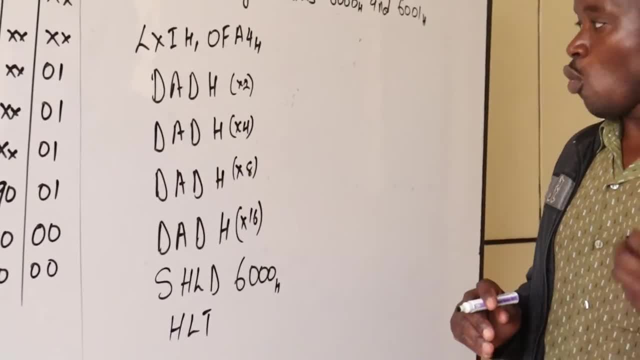 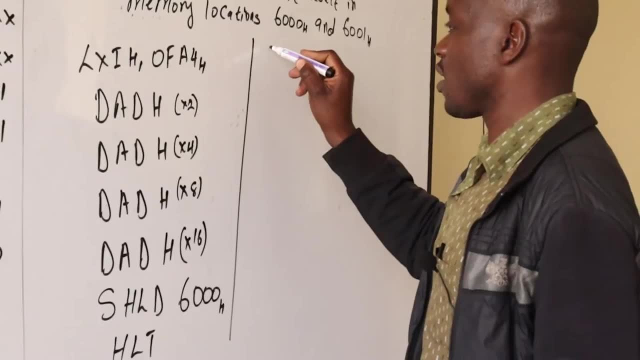 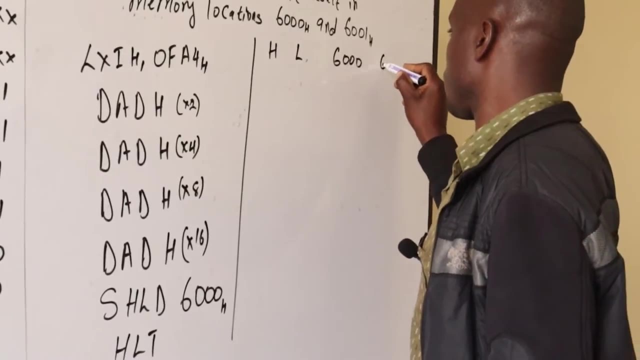 the trace table can enable one to understand correctly what was happening in each execution. So let us go. So let me draw. here We have register H, register L, We have memory location 60000 and 600001.. I don't know if we are going to get the card. 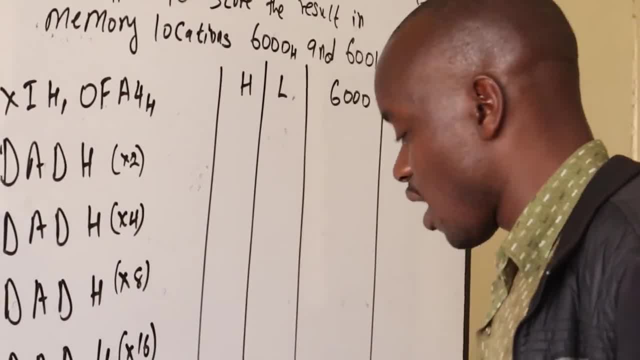 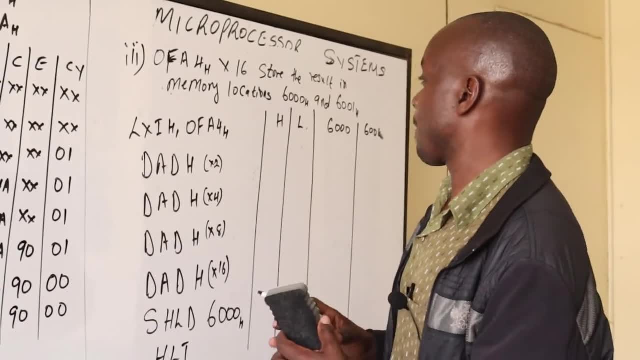 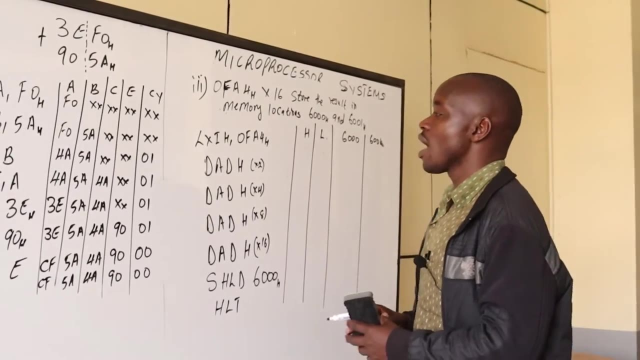 We are going to get the card flag, but let us continue. If we get that, the card flag will be affected. then we do the next thing. So what we do now, so that we get the data correctly. we start now. what's happening in each instruction? 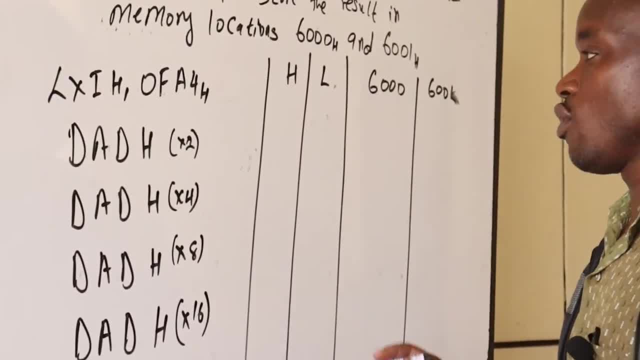 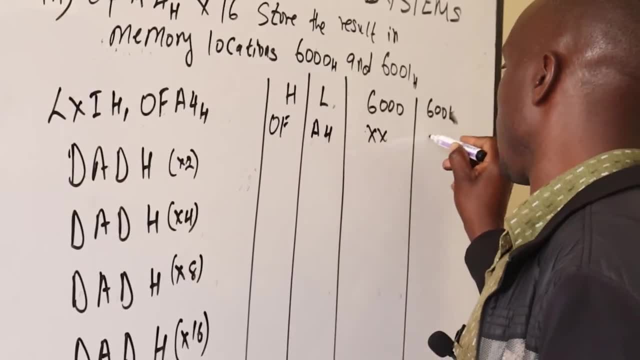 LXRH- 0F A4.. So HL will be affected, So it will be 0F A4.. We don't know what is here, neither here, We don't know what is there. It will be 0F A4, plus 0F A4.. 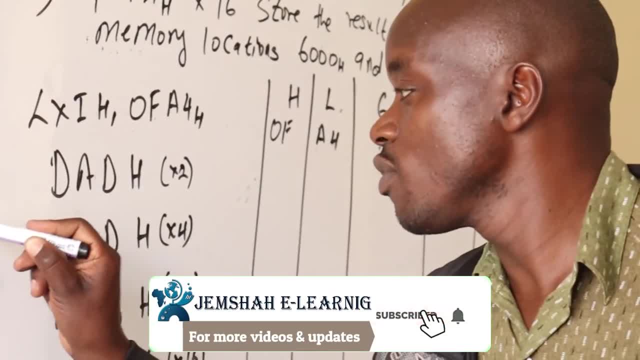 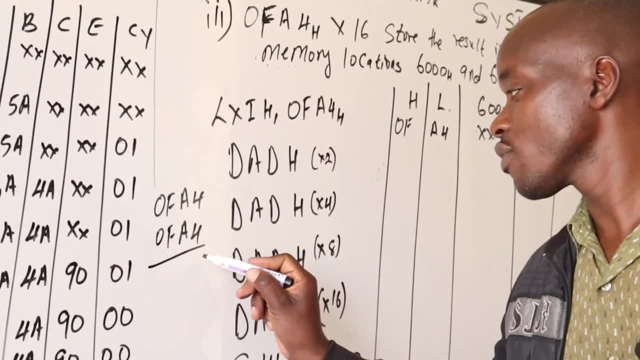 Then that H. we agree that H means times 2. But let us do it now. practically It will be 0F A4, plus 0F A4.. So here now we have 0. I want to reduce this byte to, maybe to a small number. 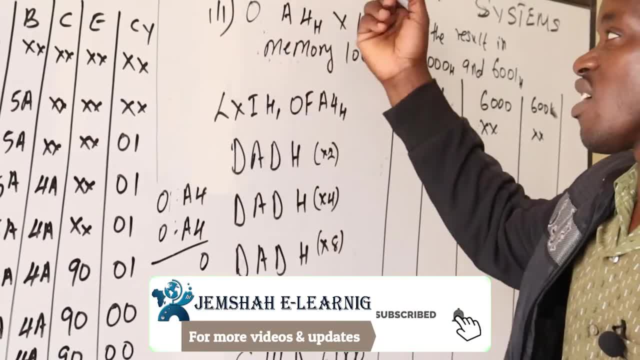 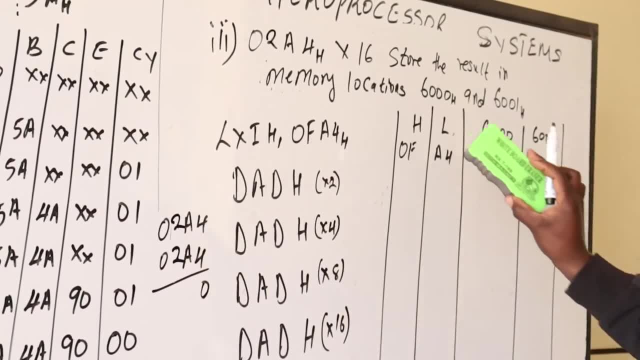 so that maybe I don't get the card. For our case, let us use something: 0,, 2,, A4. So let me use 2A, 2A. So even here We change it to 2.. 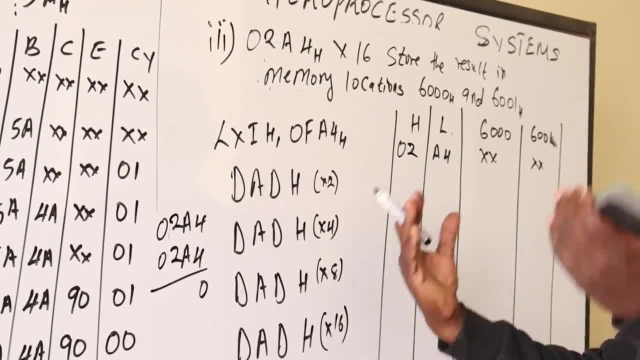 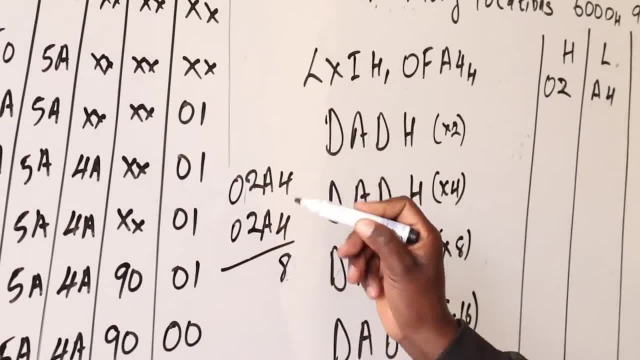 So that now I don't complicate matters, so that you start checking the card frame. So let us continue now. 4 plus 4.. So if this, 4 plus 4, that is 8.. A plus A: A is 10.. 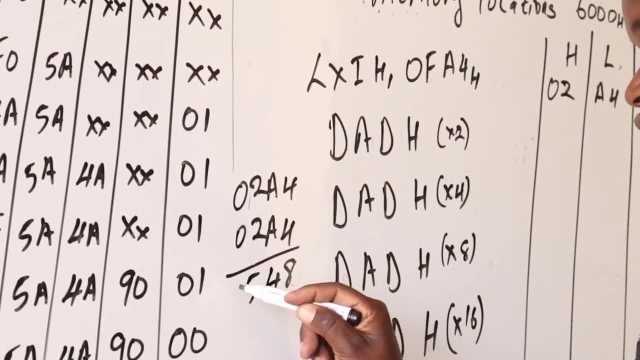 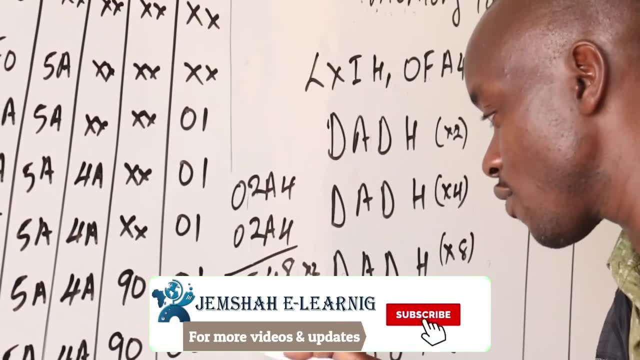 20 minus 16 should be 4.. Card 1,, that is 5. 0.. That's the first, Remember these times- 2.. That's how we agreed. Next now again is 0,, 5,, 4, 8.. 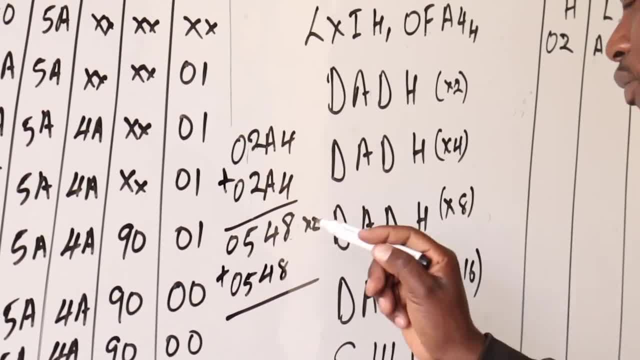 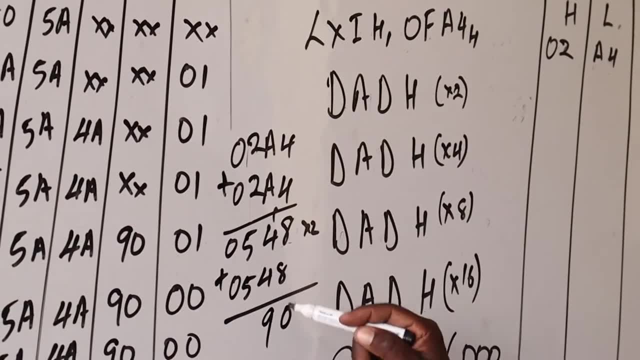 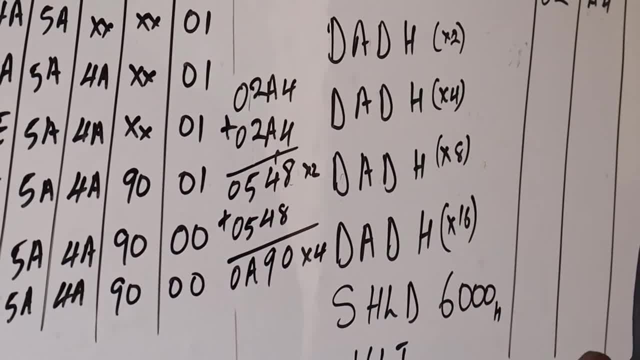 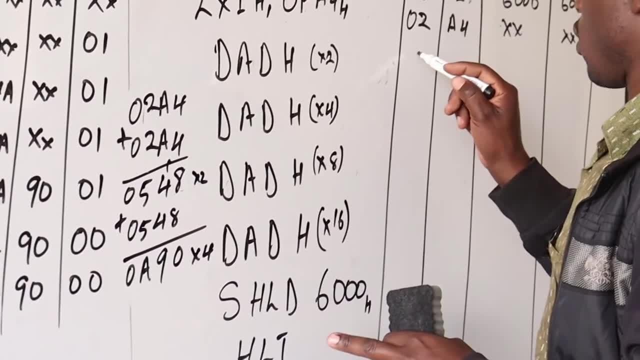 This is remember times 4.. Remember multiplication by 16.. So I'm supposed to be indicating after each what happens in HR, That H. here. now HR changes to 0,, 5,, 4,, 8.. Still, you don't know what is here. 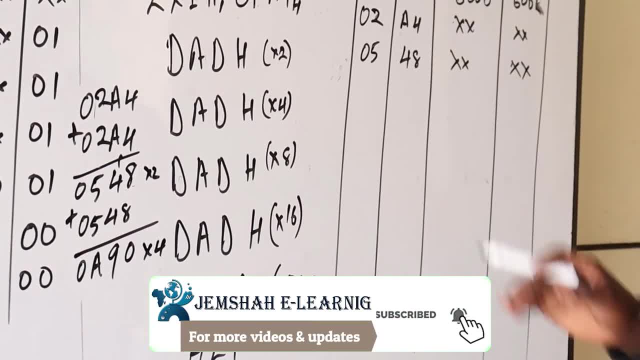 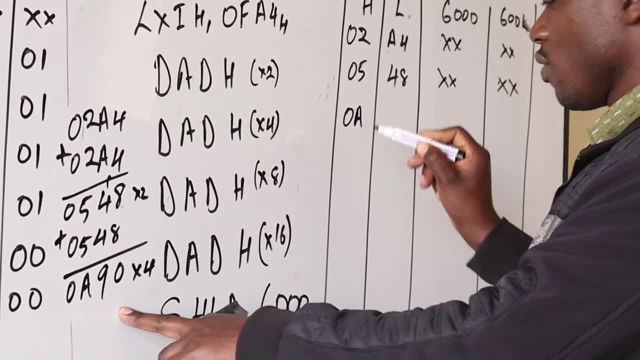 Neither we don't know what is here. Next is after that, again by 4,. here we have now guessing to that one from 2, 0A 9, 0. We don't know what is here, and yet we don't know what is here. 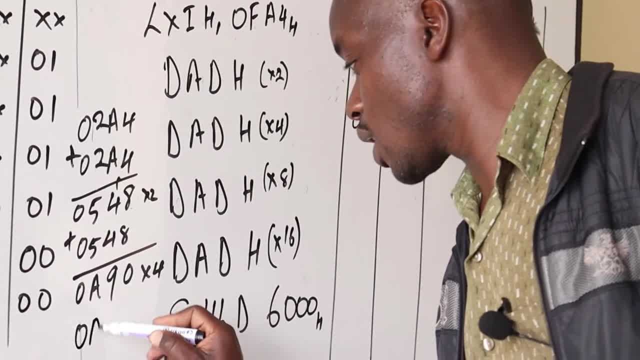 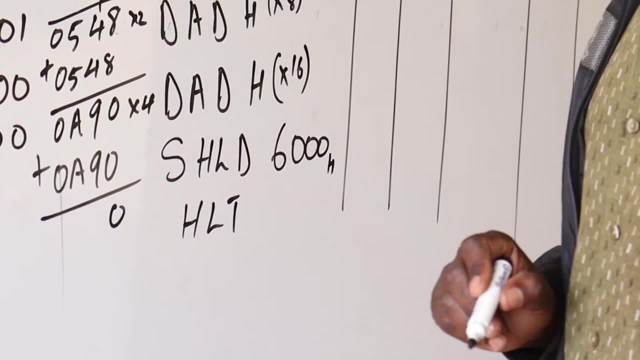 Then again that H times 8, that H 0A, that H Add again 0,, 0 is 0.. 9 plus 9 is 18.. That's 2. Card 1. 9 plus 9 is 18.. 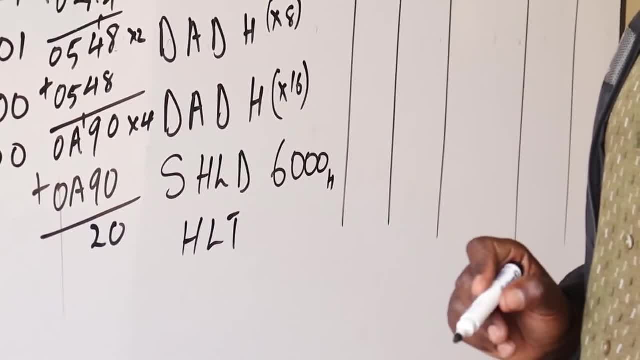 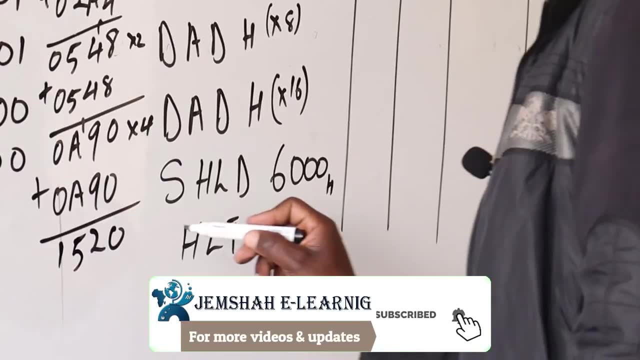 That's 2.. 1 plus 10 is 11, plus 10 is that should be 5, carry 1.. So the answer: this times 8, times 8 here. So here we have 1, 5, 2, 0.. 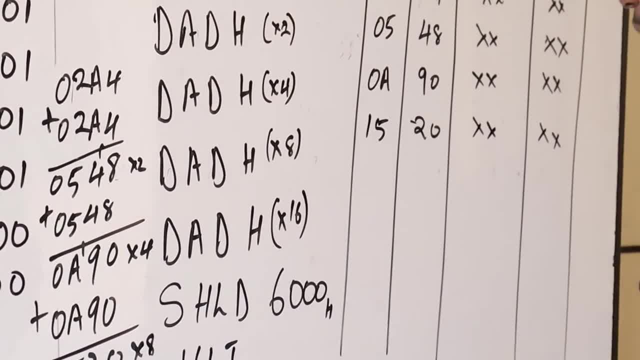 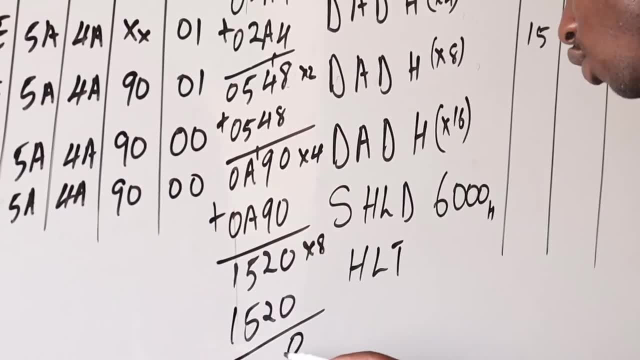 We don't know what is here, Neither we don't know what is here. And then lastly, that H again. So it is 1, 5, again, plus 1, 5, 2, 0.. So here we have 0, 4, A, 9, 0. 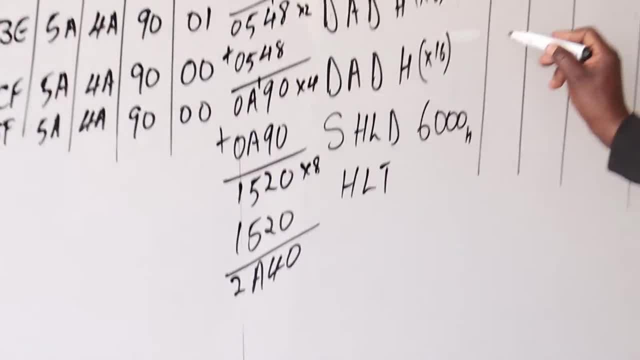 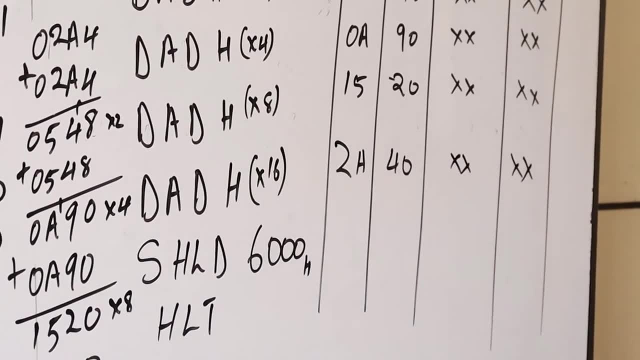 1, 5,, 2, 0.. 2, 8, 0.. 1, 5 here, Because we know how it should be. It is 1, 5, 0 here. Before we pay attention. before we pay attention. 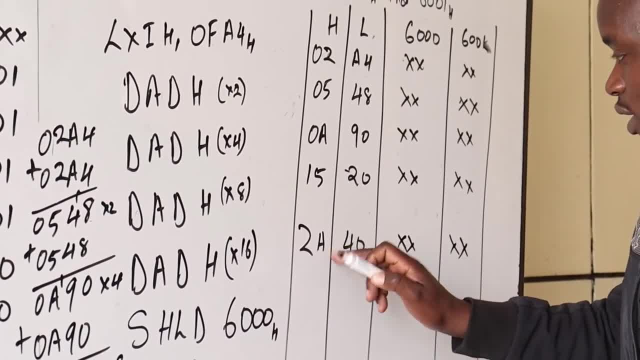 Then here we have 1, 10,, 1, 8, 0.. Then here we have 2, 8,, 1, 8, 0.. 1, 6, 8,, 1, 8, 0.. 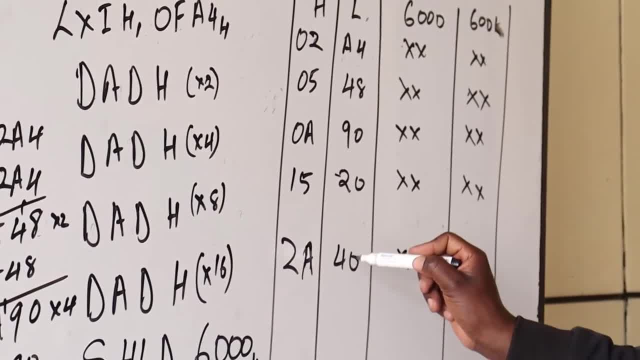 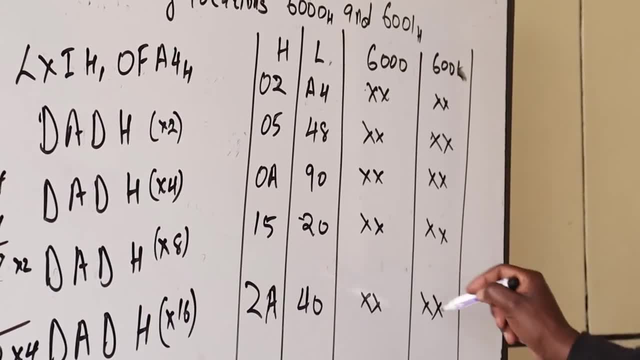 1, 6.. 5, 8, 1.. 1, 6.. We will surprise, because we know how to do this. what is right now? We have two And 2, 5, 0.. 2, 8, 0.. 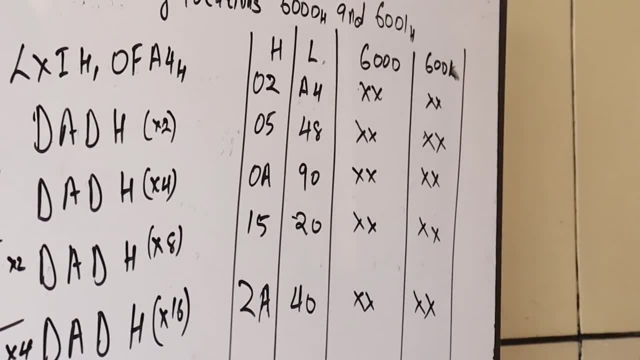 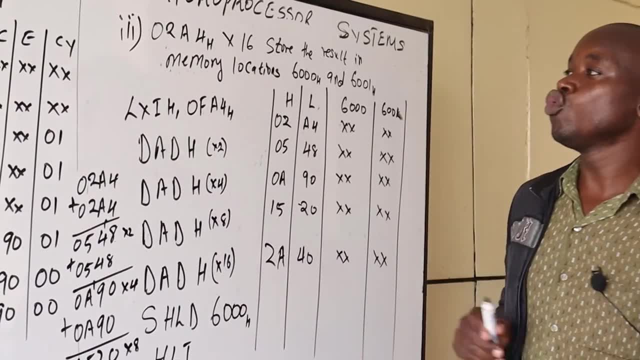 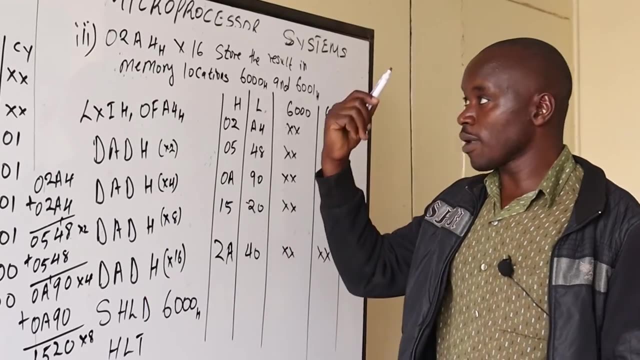 One 0. 1.. we want to be told to store hr direct. so before we end by store hr direct, i want to again you during your own time: convert this 202a4 into a decimal, then multiply by 16.. once you convert by 16, convert back to extra decimal. confirm if the result becomes what 2a40. 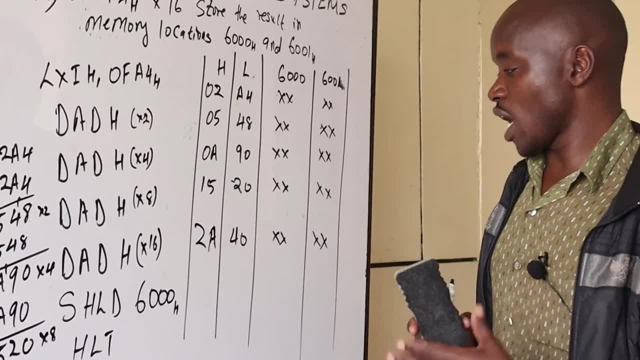 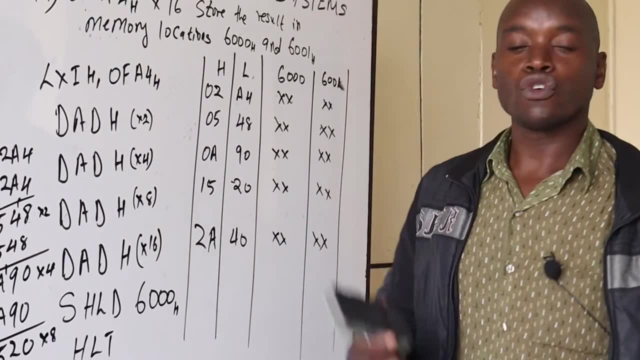 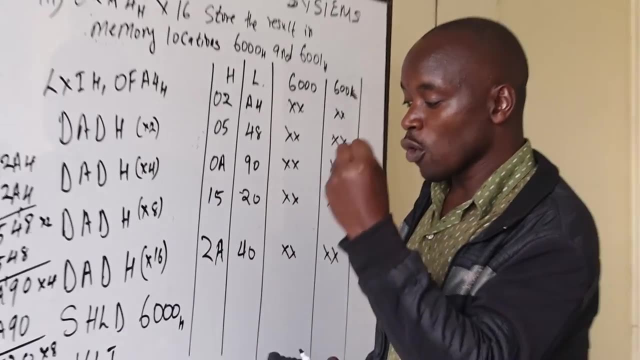 if it is that way, then now the program is able to do what to run. so that's difficult instruction. people tend to think it's difficult. i want to explain it using this example, which says: store hr direct 6000. we agree. this way it stores data into two consecutive memory locations, starting with 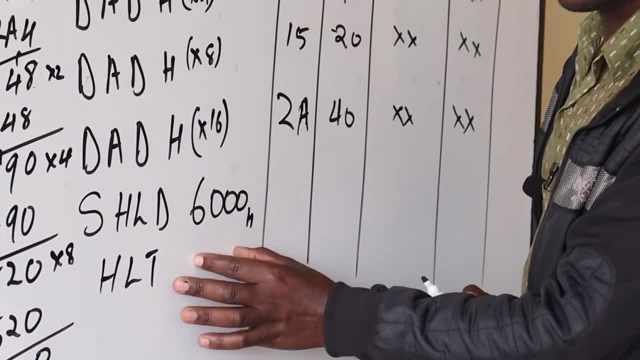 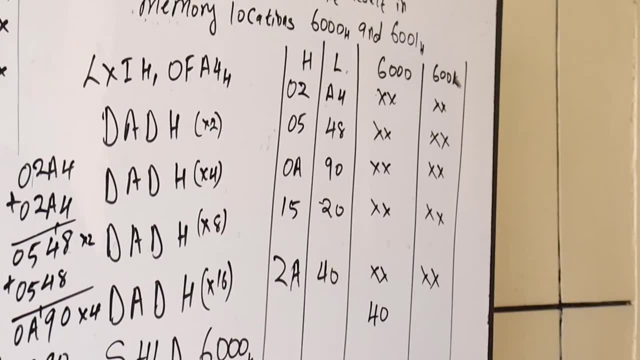 what's in air to 6000 and then what's in edge to 6001. what's in air is four zero four zero. it will go here. that's the memory location. six thousand. what's in edge is two a. we'll go to the next. 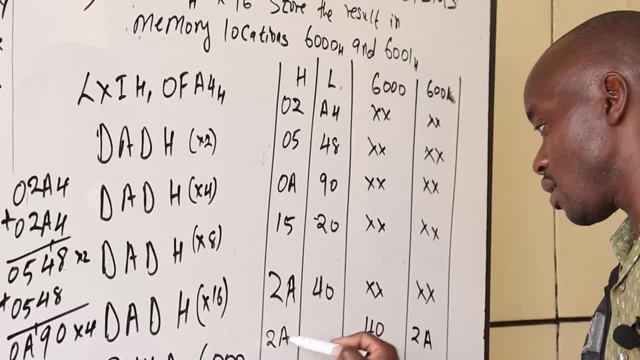 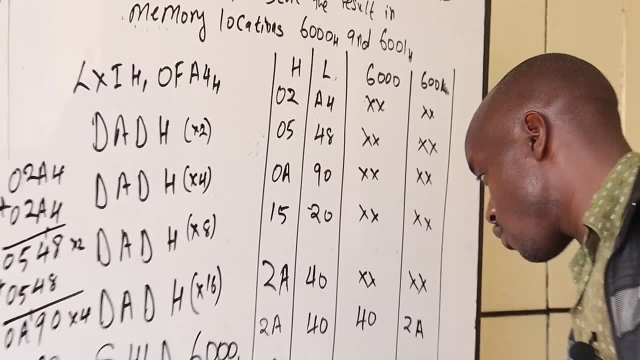 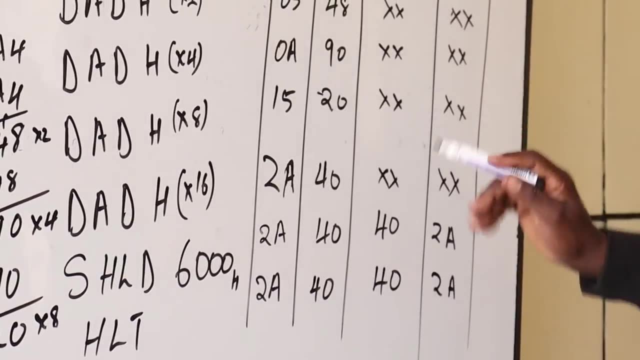 memory location, then again still will remain here four zero. so once we stop, still h will be f in two zero, r will be f in four zero. this memory location, because we have stored, will be f in four zero. and then we have two a, and now this is what the instruction will be doing in each execution. so i want to end by saying this way: 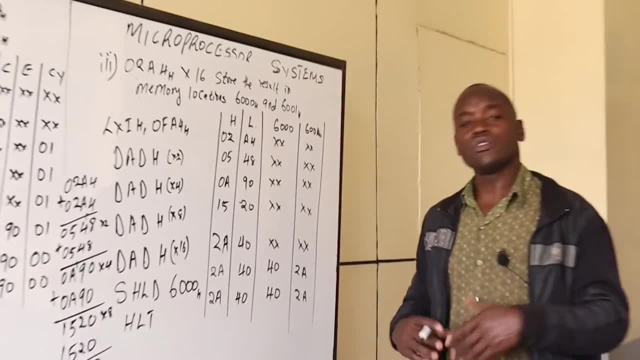 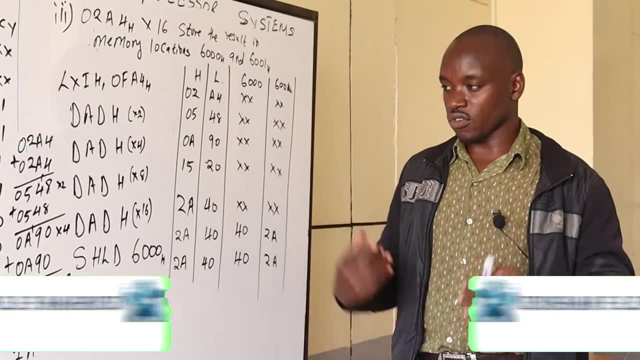 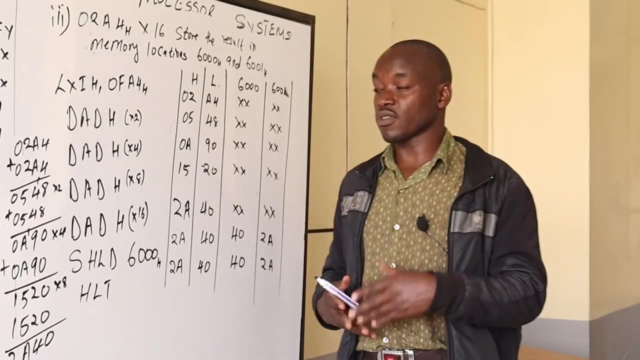 the entire 885. microprocessor programming is not difficult. what is required by the candidate or by the lecture i was teaching is to understand the instructions and then apply them in the writing, their programs. once you do this way and then if you have the, the microprocessor set, 888. 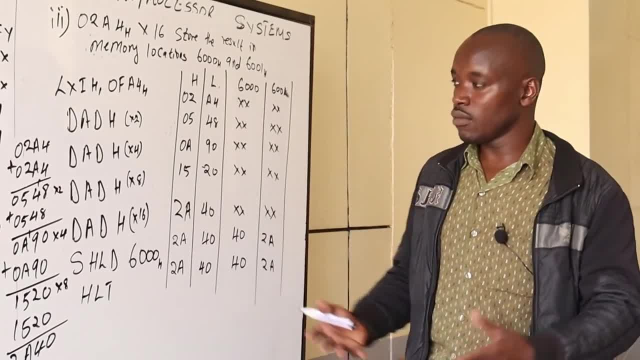 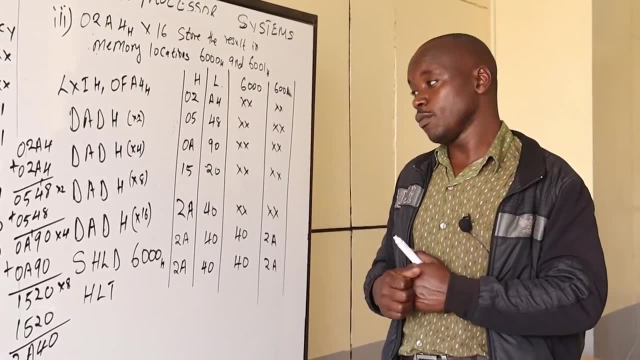 log 885. you run the programs, you assemble them there, you exclude them. then things will be cheap or will be easier to run, and if you have a question you can put them in our youtube gemusha. once we see them, we are. we should tackle them so that at least at the end of the course or at the 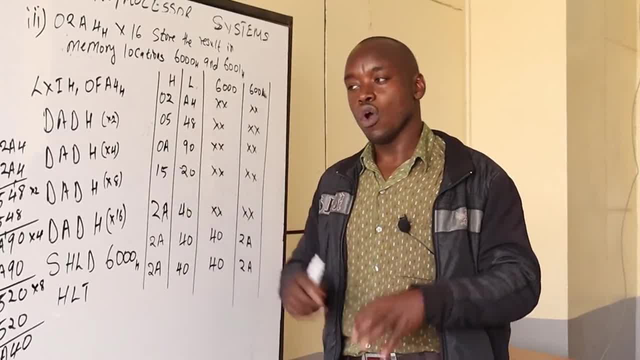 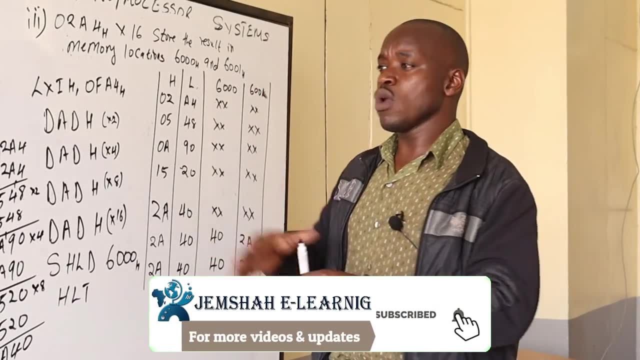 end of the day, at the end of the lessons, at least most of the lessons, are going to be done by the microprocessor, so that at least most of you have understood what's happening in microprocessor. those who fear microprocessor, who tend to think the program is very hard, you have seen since we 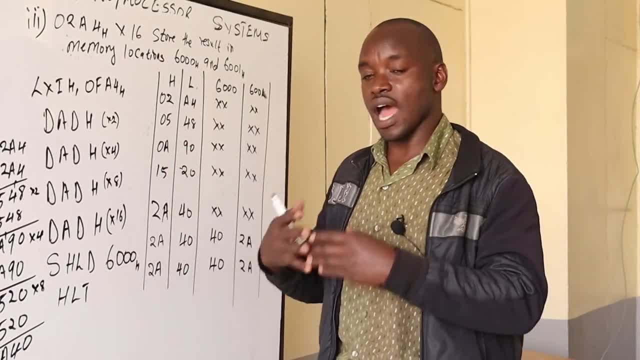 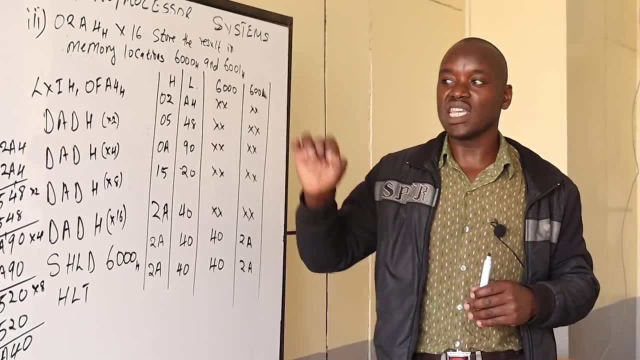 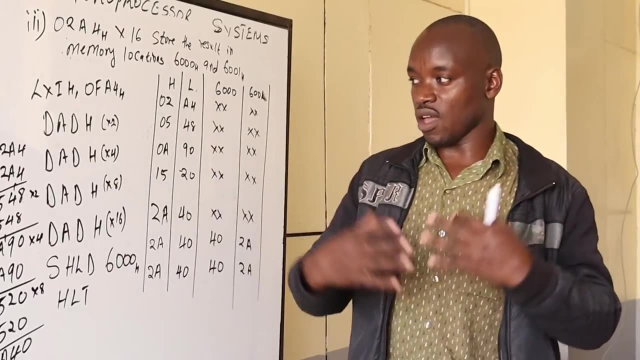 started with you here what we are doing. things are simple, so long as you understand the instructions and so long as you know where you apply them. when we shall meet next, we shall go to more instructions. in 880, stroke 885, write more programs, do more calculations here and there, answer your.